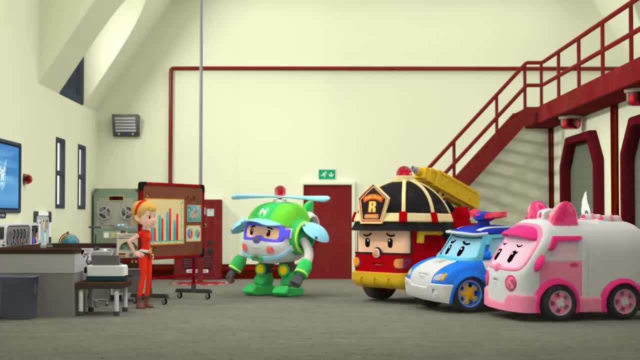 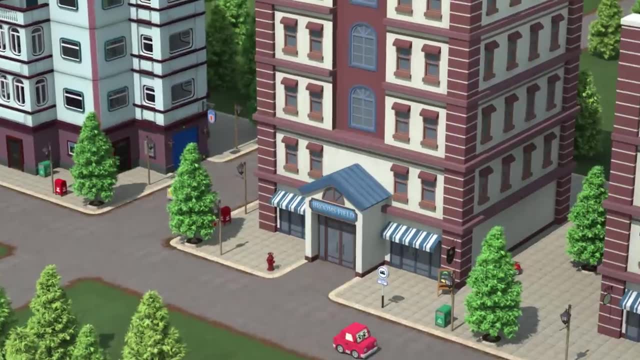 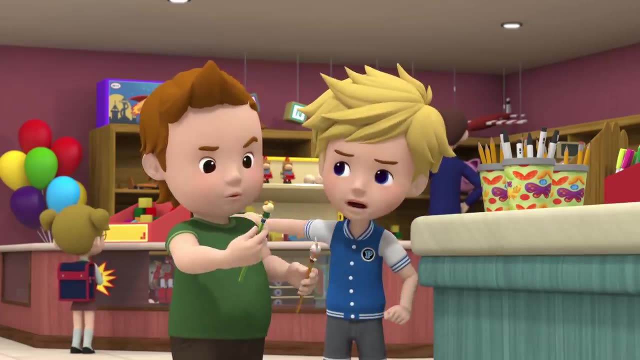 Sounds like a serious problem. Yes, it is, And we seriously need to do something about it. We must start teaching people fire safety now. Hmm, the bunny or the doggy? Which one, Johnny? let's go to the toy store. 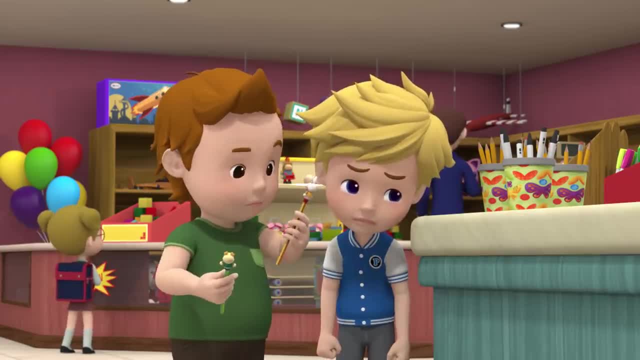 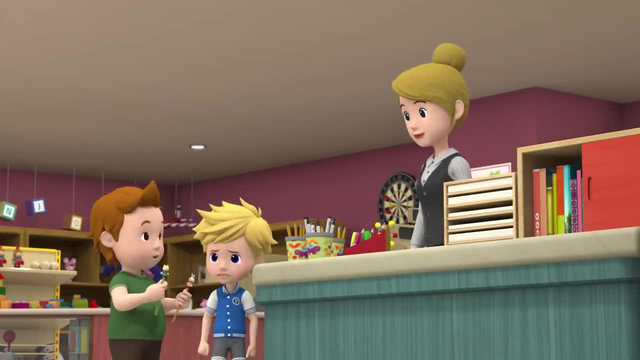 Just hang on, Peter, I haven't figured out which one. Do you need some help? Uh, hello Need help finding something. Yes, I'm just trying to figure out which pencil to get a girl. I'm torn between these two. 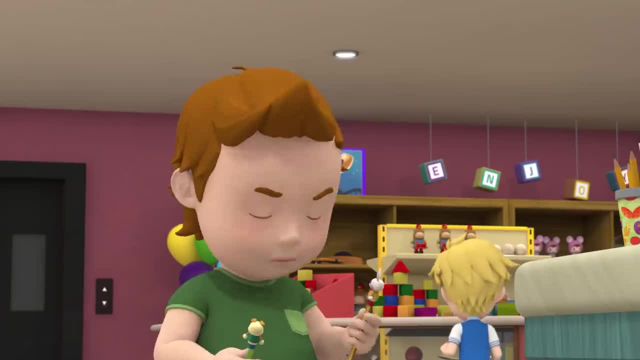 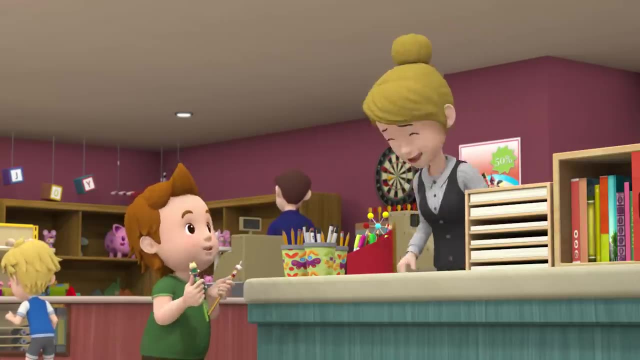 Well, I think she would be happy with either one. Hmm, do you have one with a gorilla on top A gorilla? I think there might be one in the back That would rule. I'll just go get it. I'll be back in a sec. 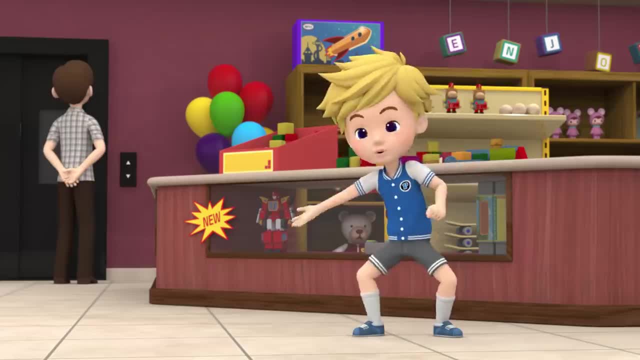 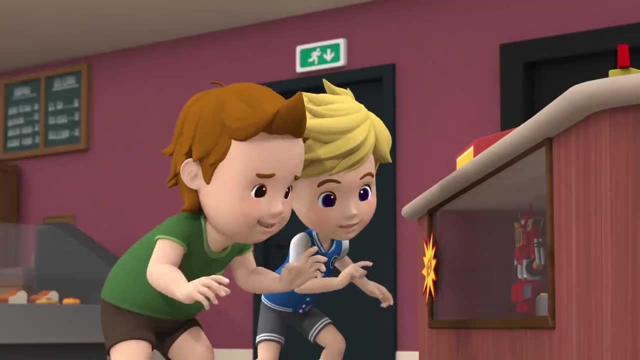 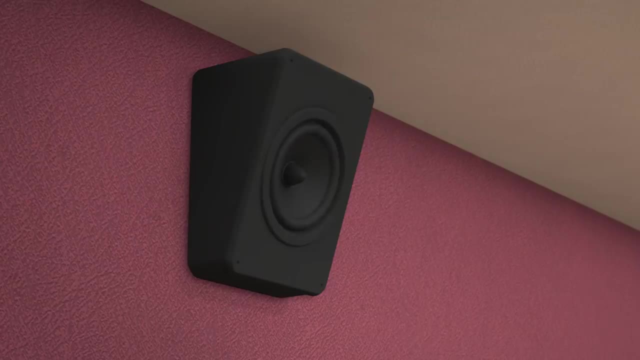 Great, Hey, thanks a lot, Johnny. look A super dragon. Wow, It's awesome. Oh, wow, Huh, What's that noise? Attention customers: A fire has broken out on the third floor. Please follow the staff and safely exit the building. 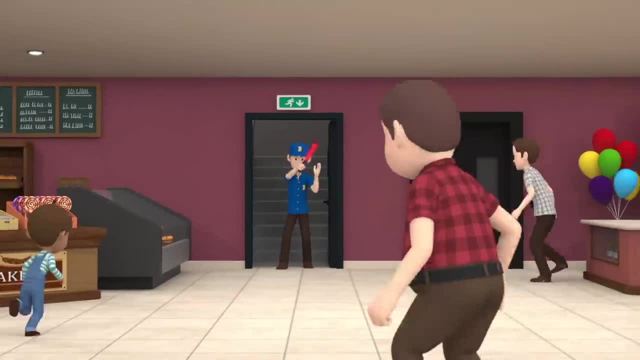 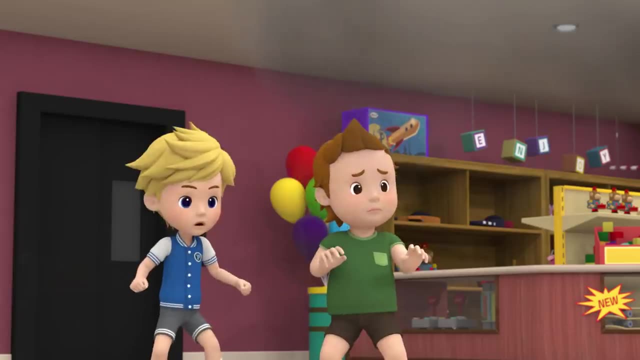 Again. please follow the staff and safely exit the building. Come on This way. everyone Over here, Everybody out, Be careful. Come on, Look, There really must be a fire. Huh, Whoa. I've never seen a real fire. 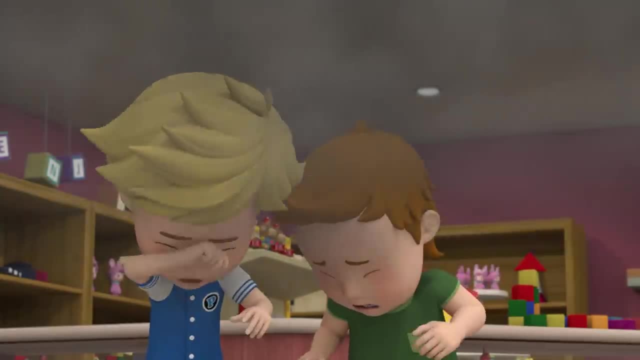 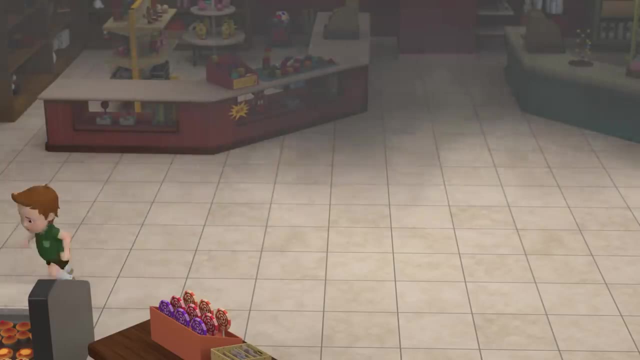 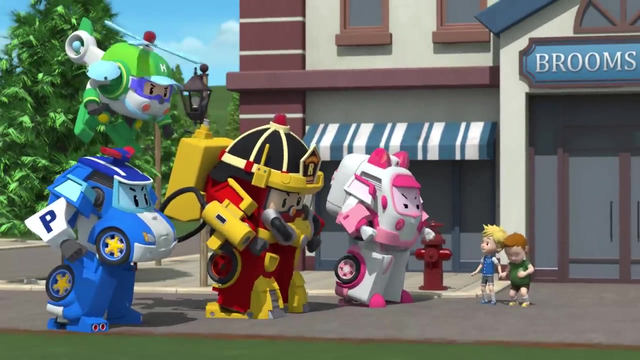 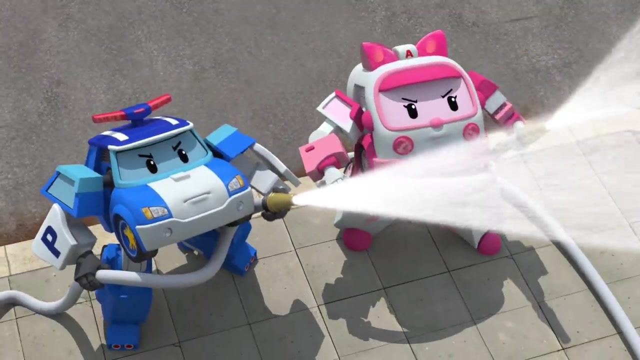 Ugh, I can't breathe. It burns my eyes. Boys, you're in danger. Follow me, Okay. Children, are you all right? Amber, It's dangerous here. Go somewhere safe. Uh-huh, Ah, Heli, put out the fire on the top floor. 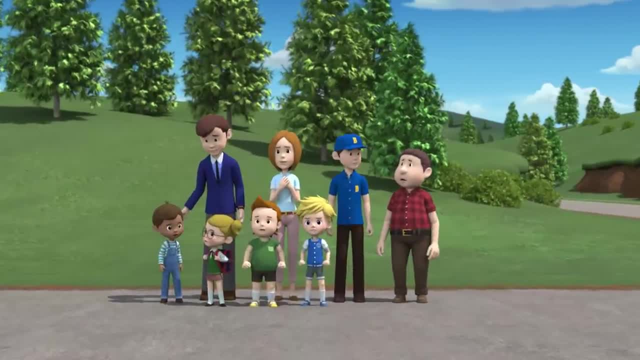 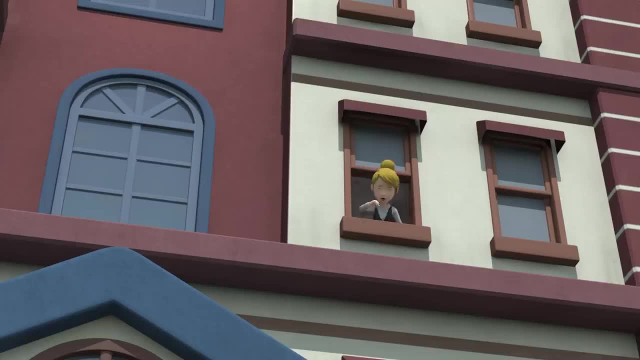 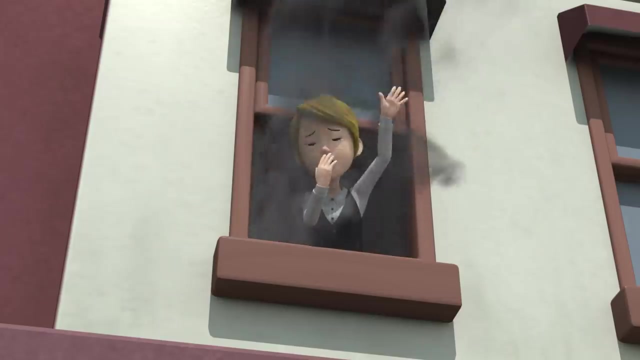 On it. Who knew fire could spread so fast? Fire is really scary stuff. Help, I'm here. I can't get out. It's the Gorilla Clerks. Please Help Polly Amber. Keep dousing the fire. 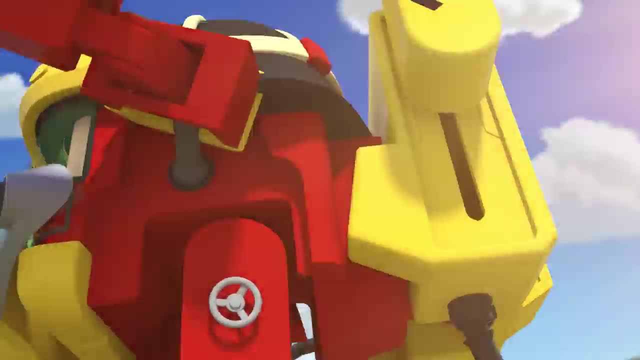 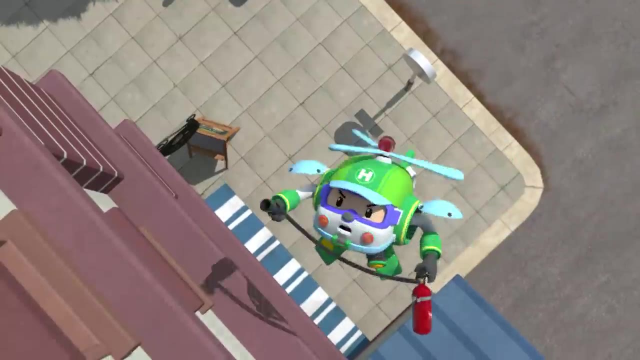 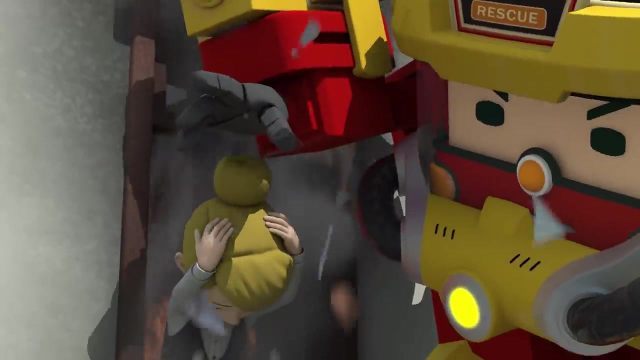 Heli and I will go help her. 10-4, Roy, 10-4, Roy, Hmph, Hmph, Ah, Somebody help. Ah, Ah, Ah, Ah, Ah, Ah. Here, take my hand. 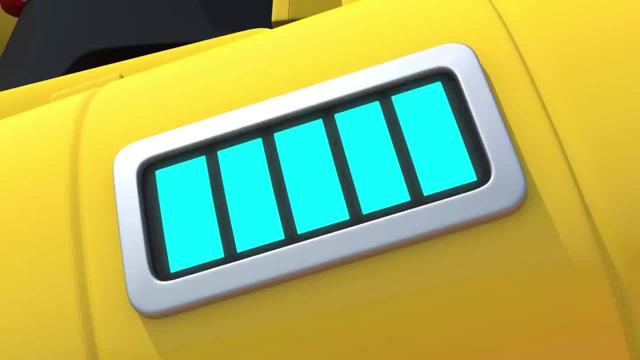 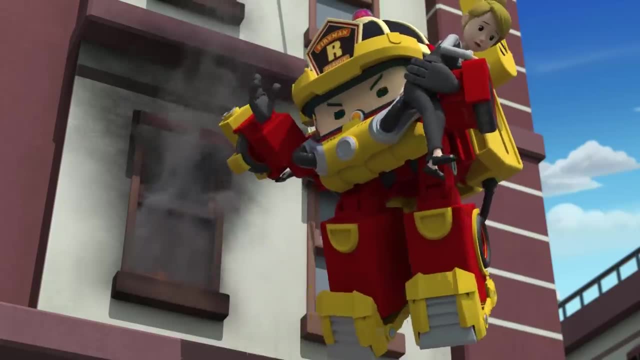 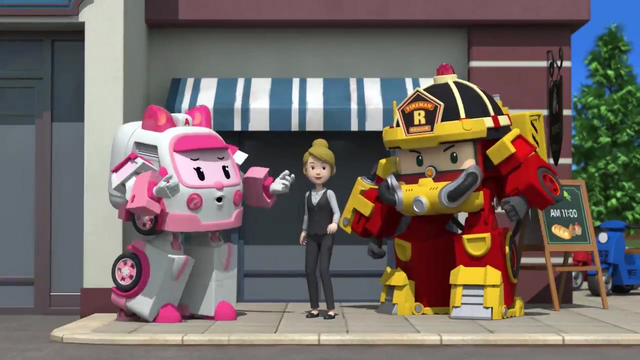 Yeah, I'll try. Ah, Ah, Hmph, Hmph, Hmph, Hmph, Hmph. Heli, please say to the rest: 10-4!. Did you get injured at all? I think I'm fine, thanks. 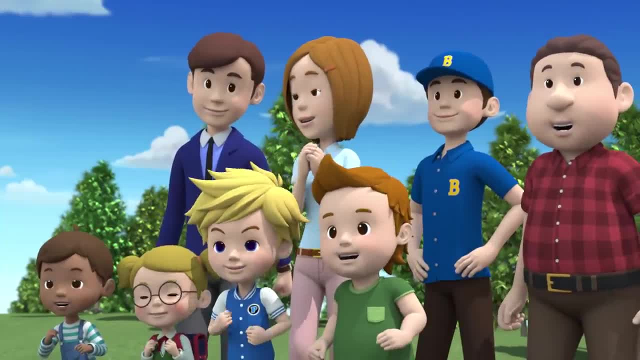 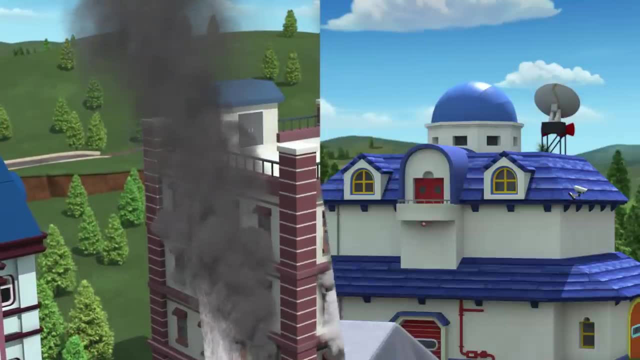 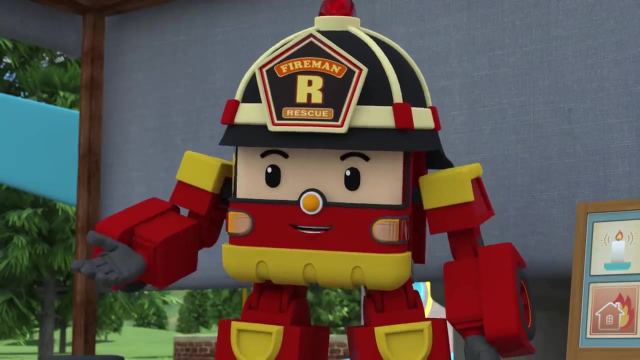 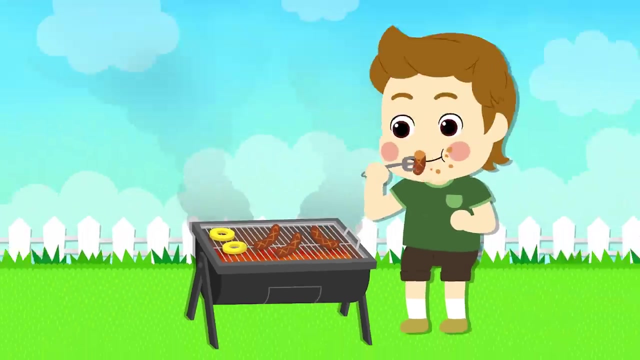 Thank you so much. Yeah, Yeah, Whoa Phew. Today's topic is scary but useful: fire- Okay, Roy, Fire is a very powerful and useful element. It lights up the darkness, making life much more convenient. It also heats and cooks food and keeps us warm when the weather's cold. 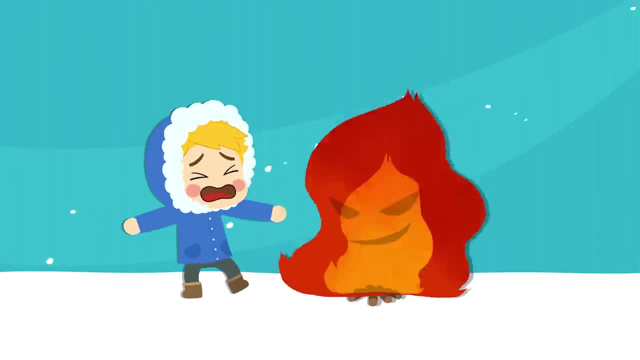 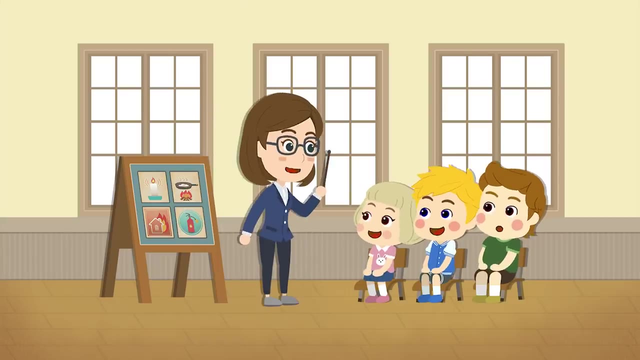 But when a fire gets out of control it can become a very scary thing. It can burn up not only the stuff we love but the very house we live in. So it is very important to be properly educated in both fire safety and fire prevention. 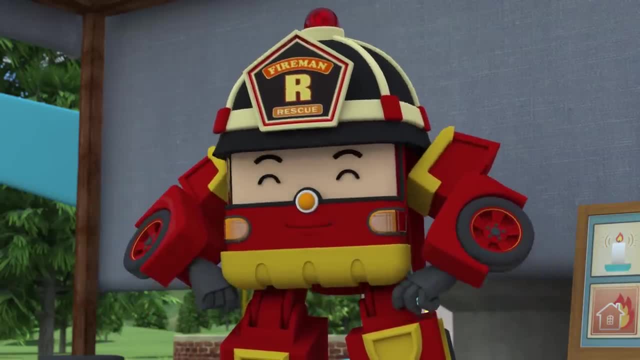 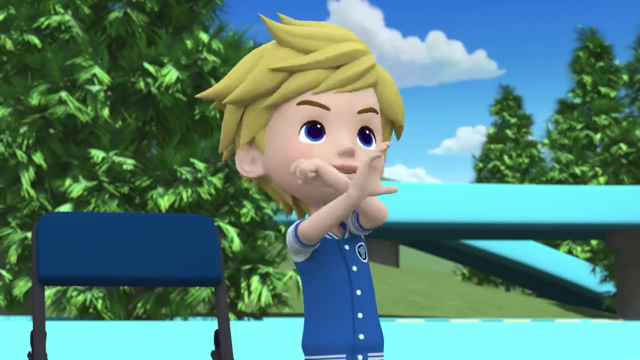 We must always be alert. A fire can break out at any time. Ah yes, sir Roy, What you did before was so awesome. Oh yeah, You heroically and bravely saved that trap clerk When you put out the fire. it was just the best. 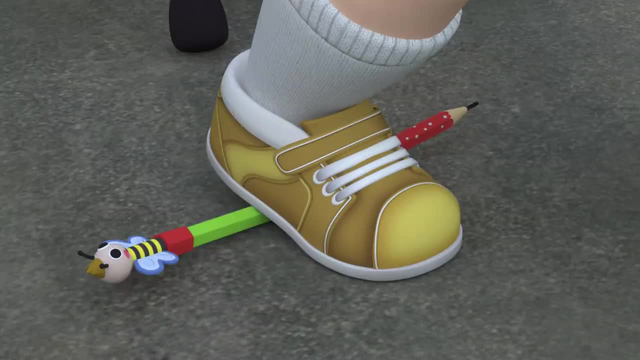 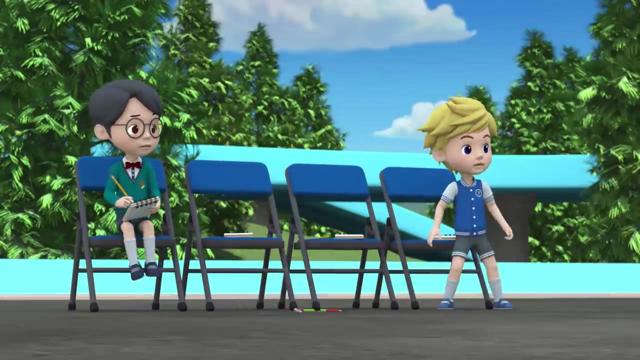 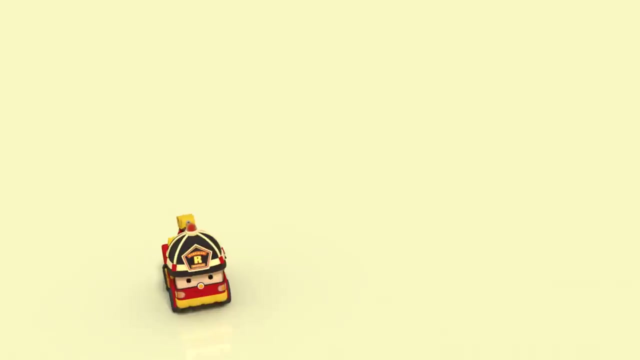 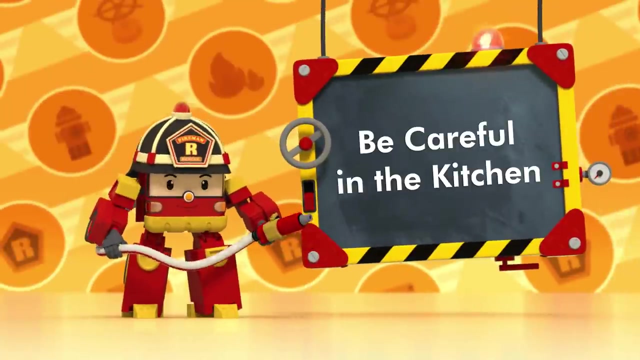 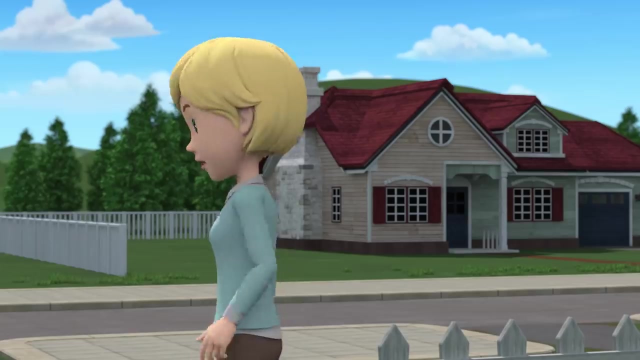 Oh Huh, Johnny, darn it. I love that pencil. I'm sorry, Cindy, Come back Bye-bye, Bye, You seem too happy I'm leaving. You better remember everything you promised me. Get all of our homework done. 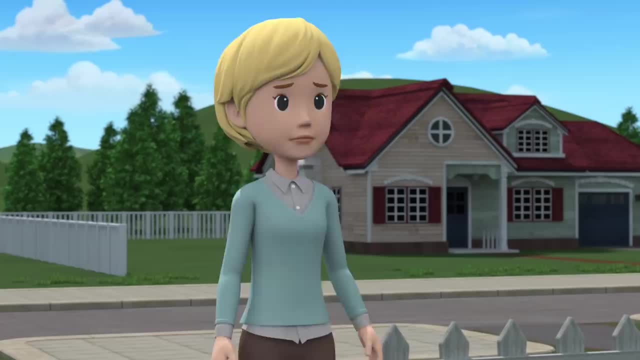 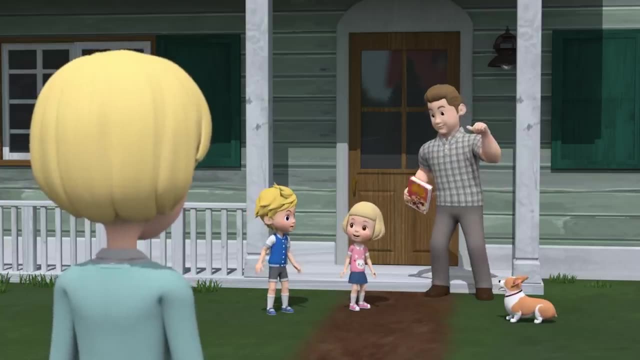 Don't leave messes anywhere And I will not let the children starve. Please don't give them only junk food. all right, Not gonna happen. I'm making something from the book. I'll make you whatever you want, as long as it's in here. 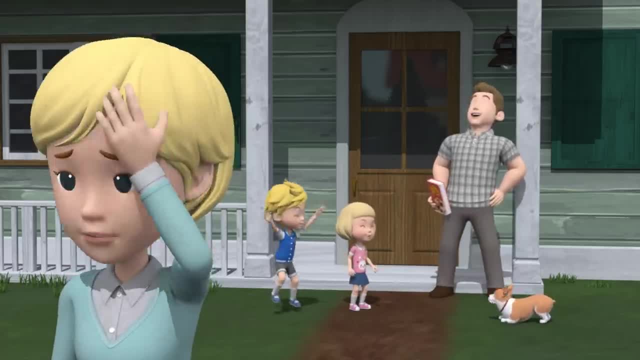 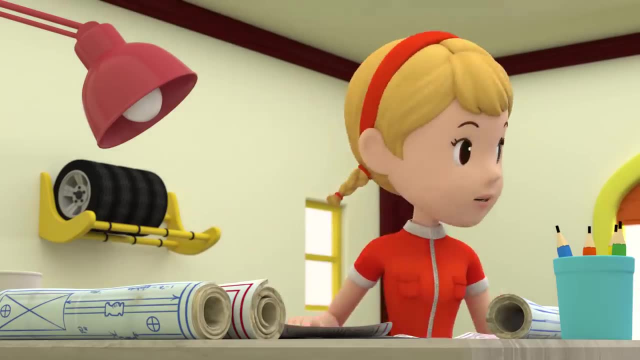 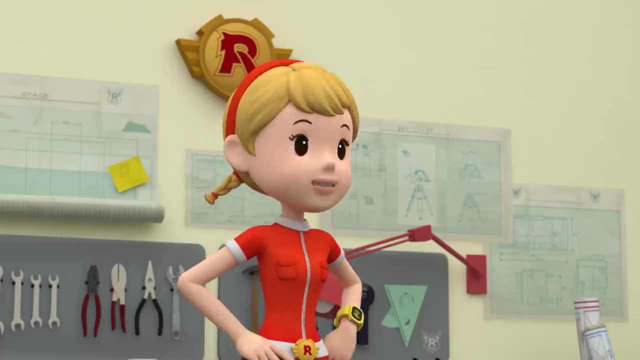 Oh Dad, That sounds awesome. Mm-hmm, Yahoo, I'm finally done. Jin, What's that, Jin? This is called the three-step alarm. Three-step alarm? I've never heard of that. That might be because I just invented it. 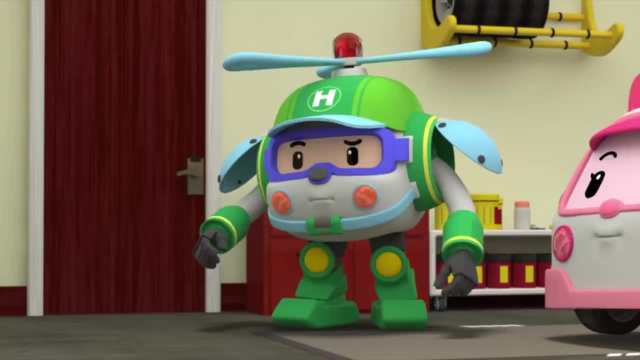 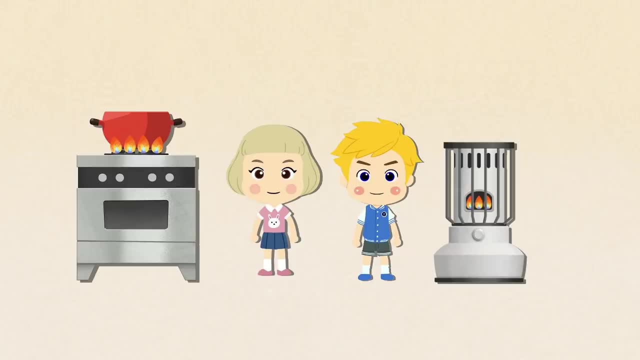 It rings when children cross into what should be a child-free area. Child-free area, Yeah, A child-free area is a one-meter zone around things that can cause an accident, like a stove or a heater. Children should be kept from entering that zone. 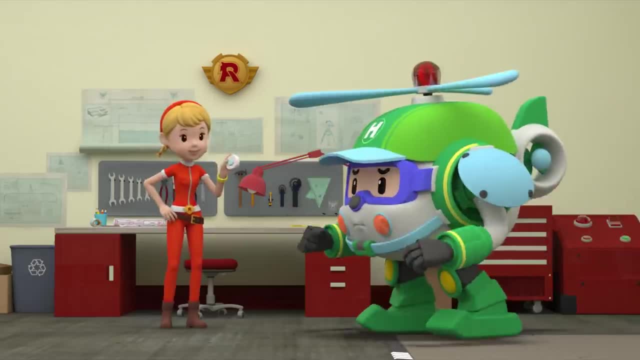 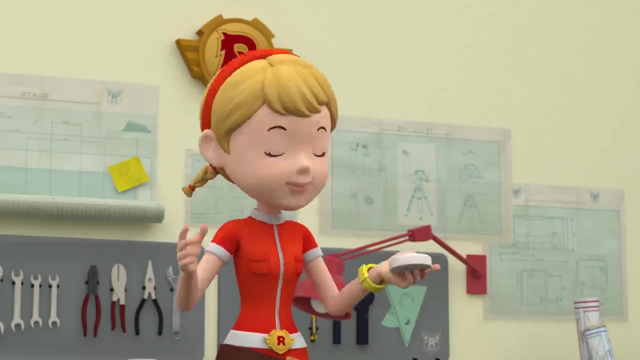 Very smart. Huh, Why is it ringing Jin? Well, a child walked into the area, didn't he? I am not a child. Just because you're big doesn't mean that you're an adult yet, Roar Ah. 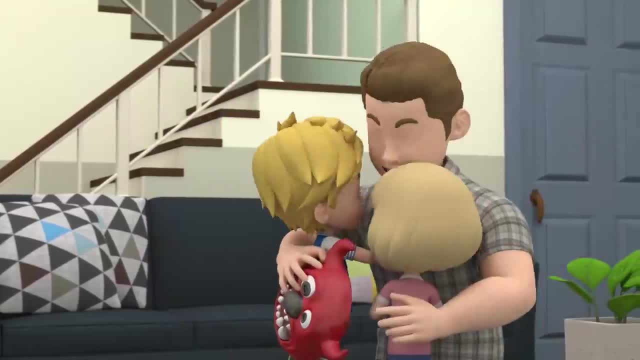 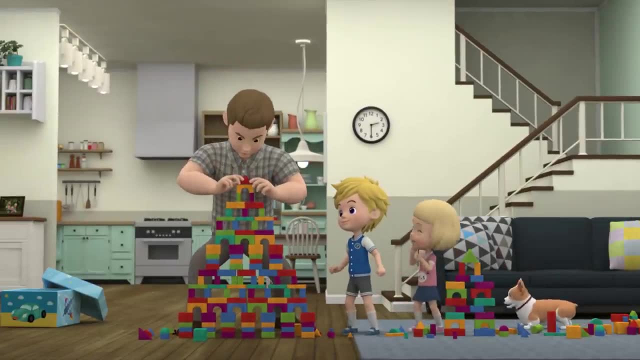 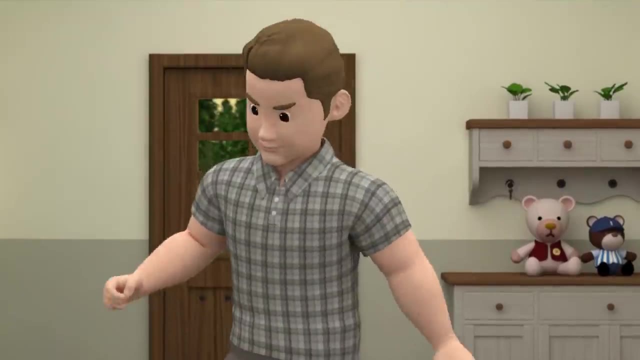 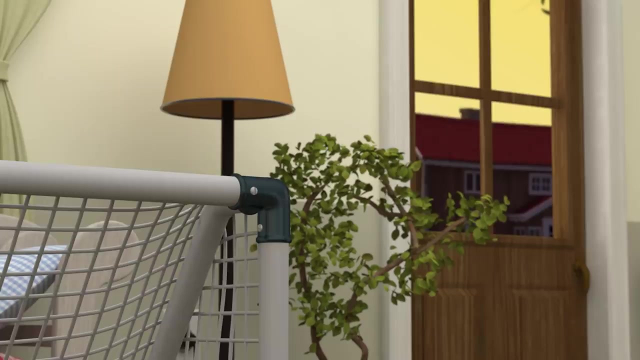 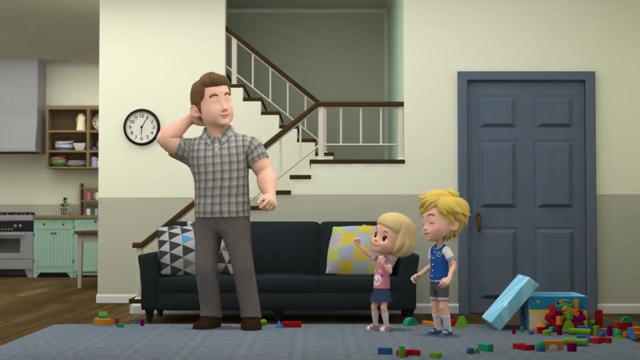 Go away, monster, Go away. That's amazing. Dad, It's done. huh Ow, I'm funny, Not a chance, Not a chance. And he shoots. Tweet: You're out, Dad, Dad's out, Huh. 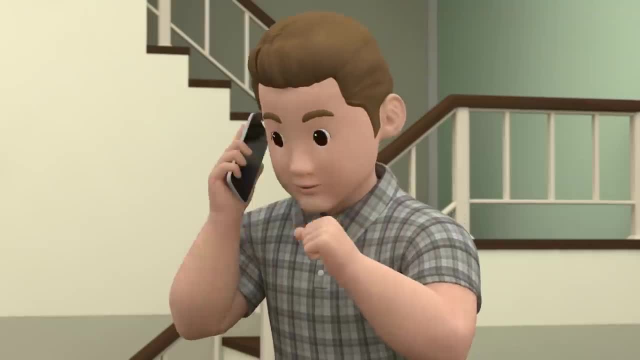 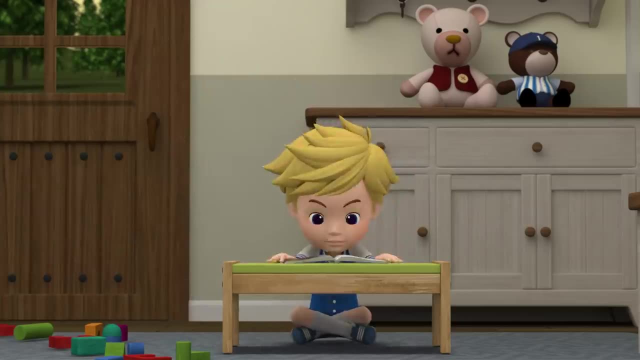 It's Mom Shh Shh Ahem. Hello, Everybody's fine. Peter, Of course he's doing his homework. Lucy, Oh yeah, She's picking up her toys Dinner Yep, Almost done. It already smells great. 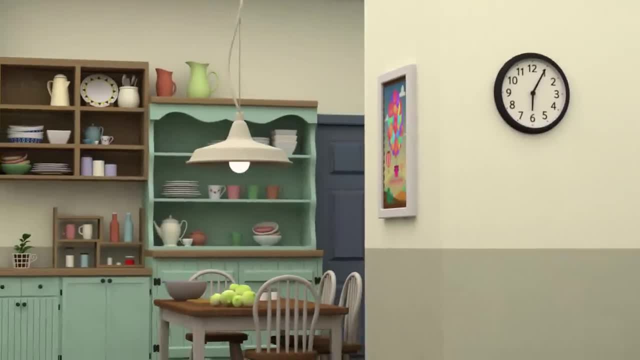 Guess I'll move along now. Please don't forget to install your new three-step alarm. We'll install it. Thanks again. Bye-bye, Roy. Next stop is Little Peter's house Right. First we chop all the onions up. 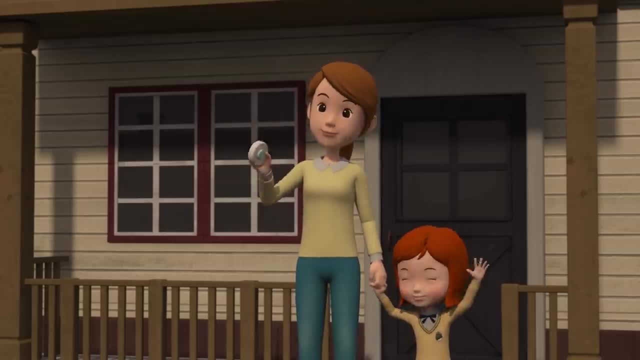 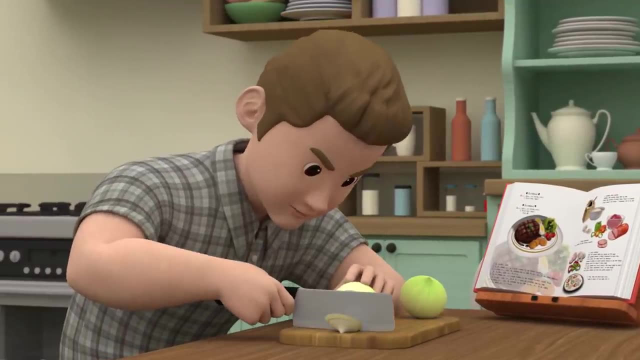 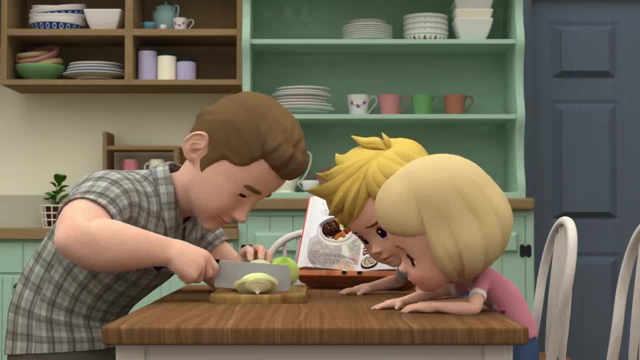 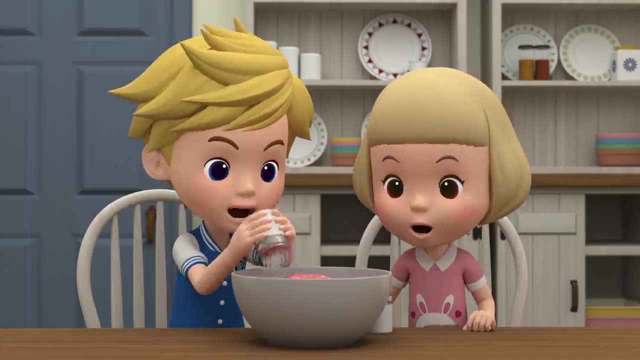 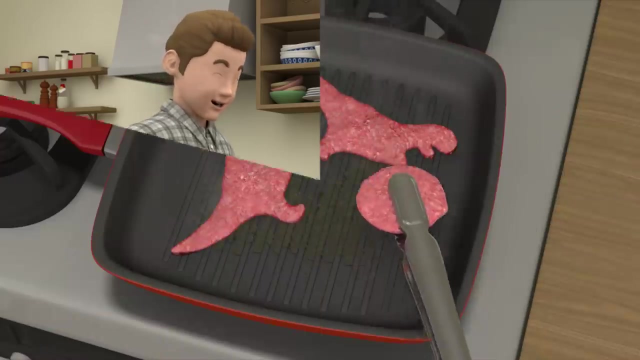 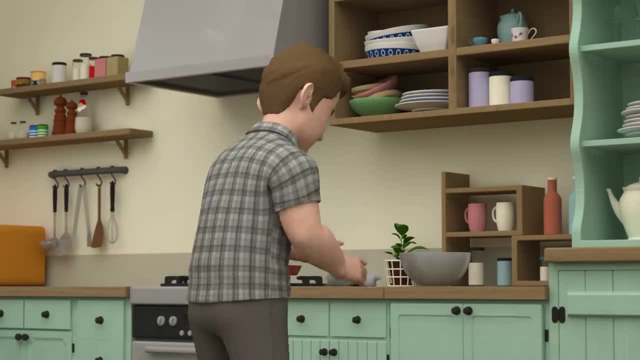 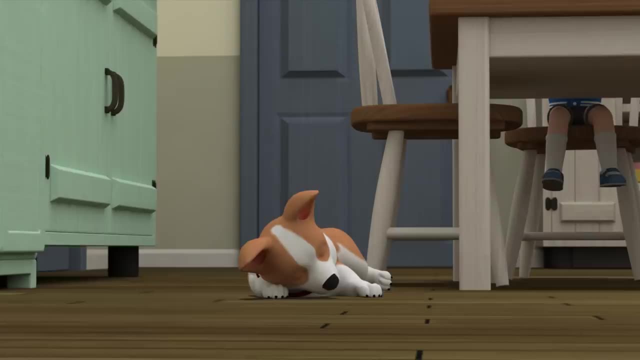 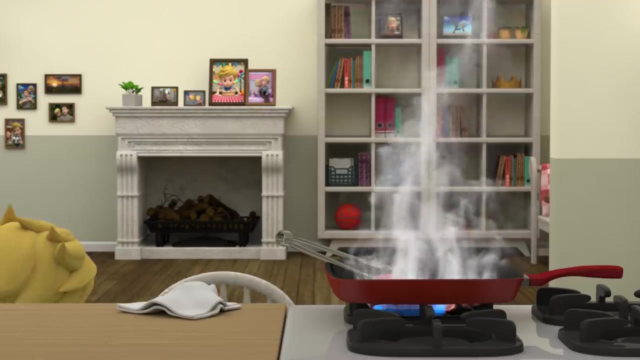 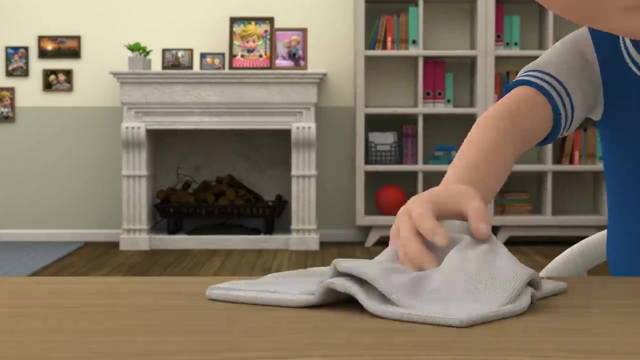 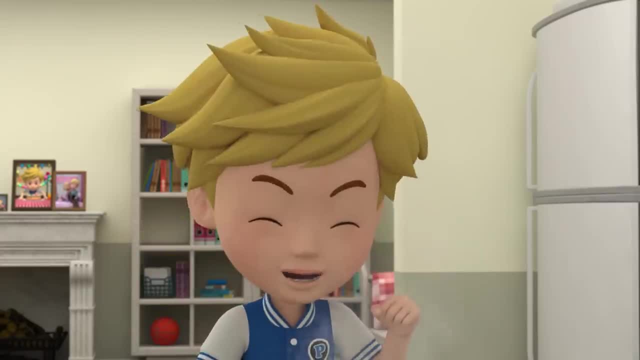 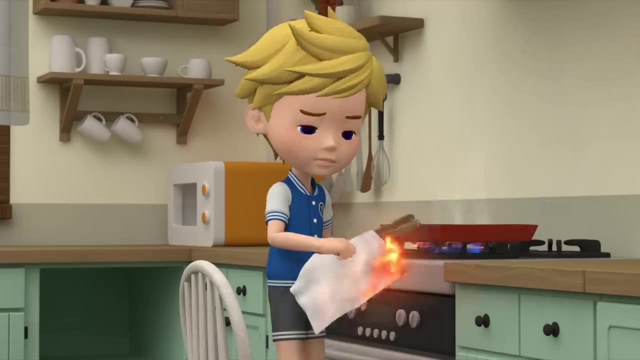 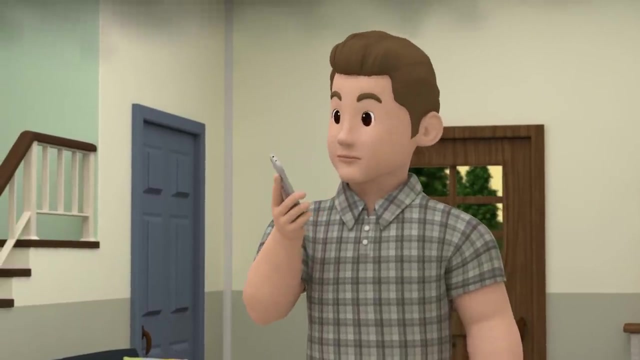 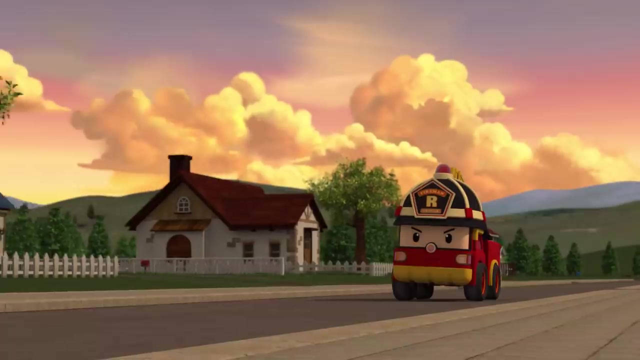 Ow, Ow, Ow, Ow, Ow, Ow. Peter, Lucy, why do you keep screaming? Just look, Just look, We'll have dinner any minute now. Hurry home, Children. Huh, Smoke's coming out of Peter's house. 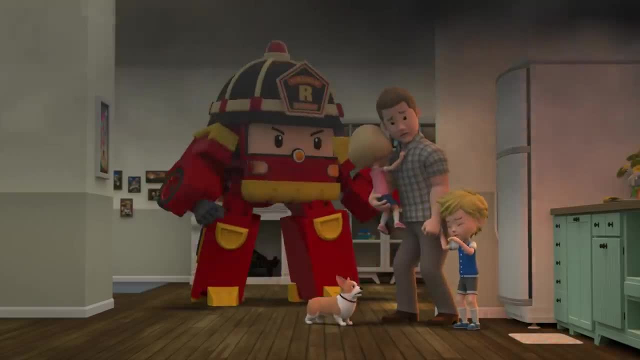 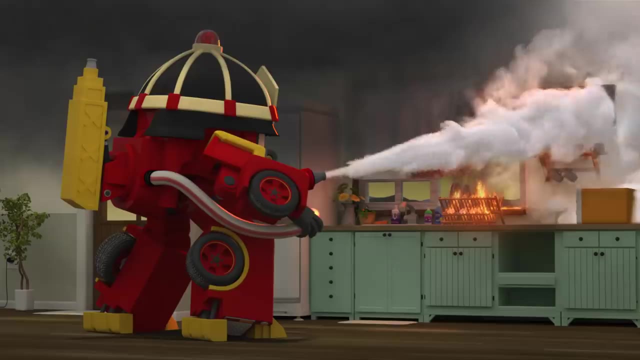 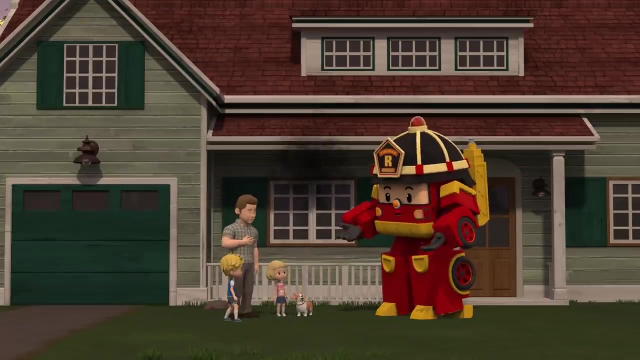 Peter, grab onto my hand. Okay, Children, Robert, You all need to get out of the house, Right? Sure, Huh, Just thank goodness that nobody got hurt. Thank you, Roy, You saved all our lives, I'm sure. 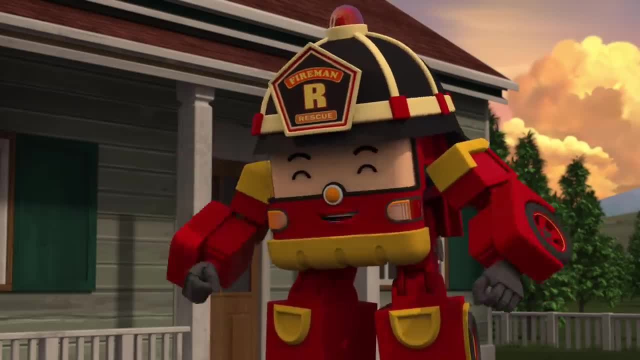 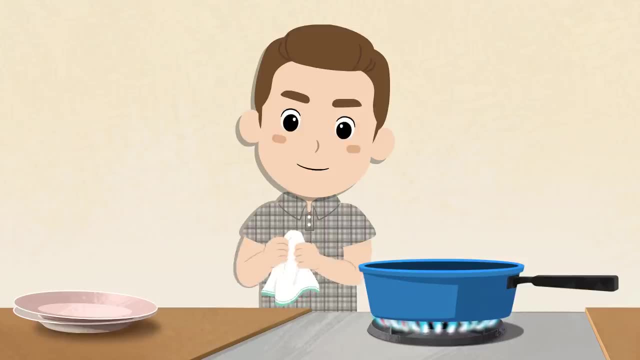 To make sure that this doesn't happen anymore, I've got some safety tips for you When you're cooking. never leave the kitchen while the stove is on. A fire can break out at any time. Also, put nothing flammable, such as towels or paper, near the stove's flame. 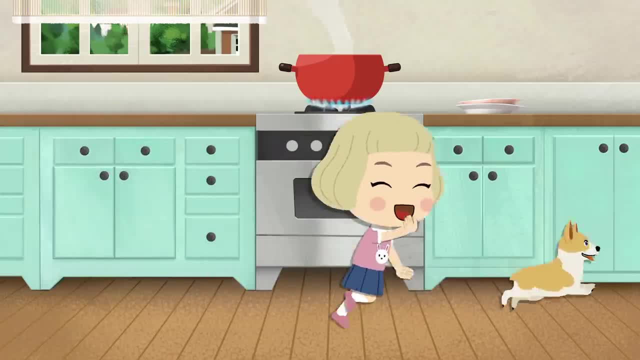 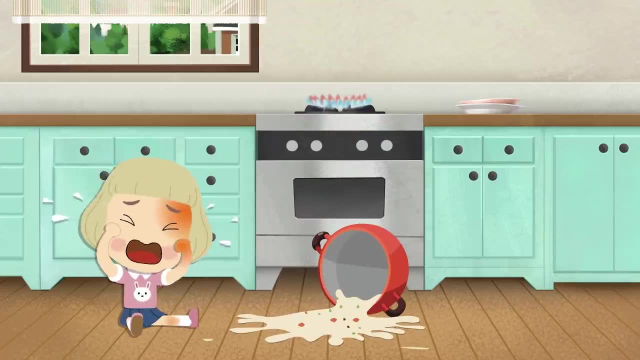 because these can easily spread fire, And don't let pets or children get near the flames or the hot food. They might have an accident and since they won't know how best to deal with it, they could be seriously injured. Yes, All right. 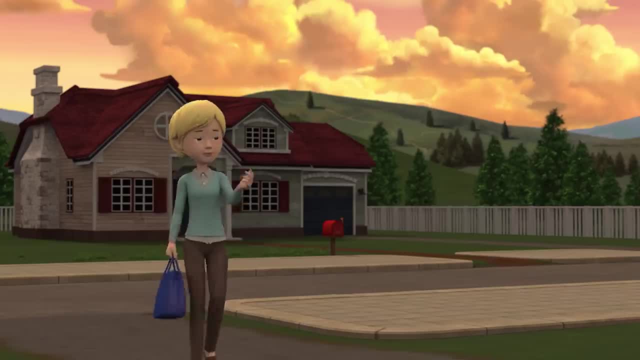 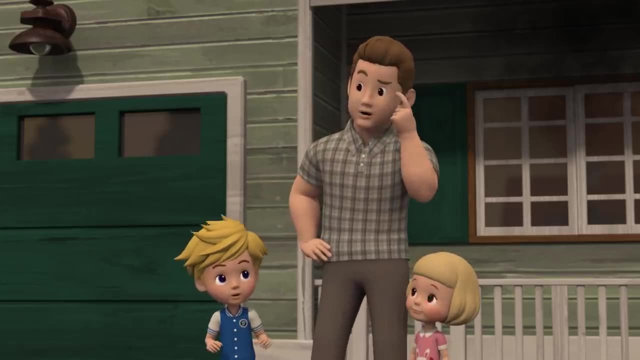 What's going on here? Huh, It's Mom. I'm home because you said dinner would be ready. now Why are you all outside? Uh, Well, Well, honey, you know about the dinner. The thing is, uh, we're eating out instead. 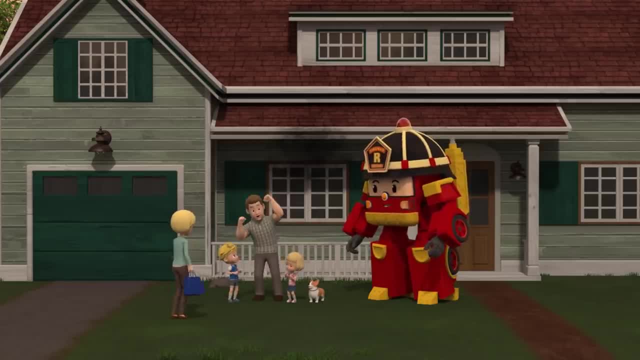 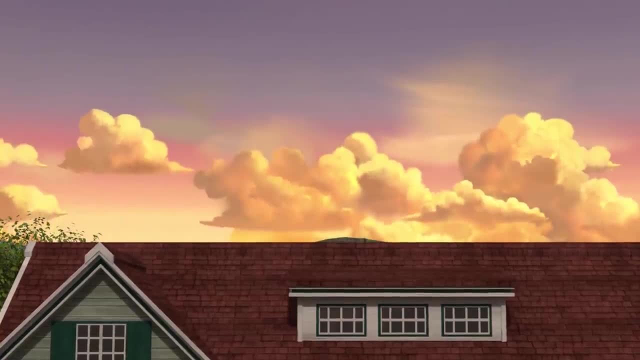 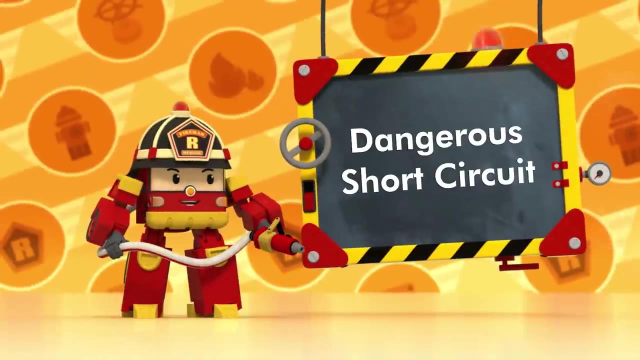 What are you talking about? I just thought we'd go out to eat. Yay, We're eating out. All right, I brought you a new cook Eating out, Eating out, Hmm, Hmm, Hmm, Hmm, Hmm, Hmm. 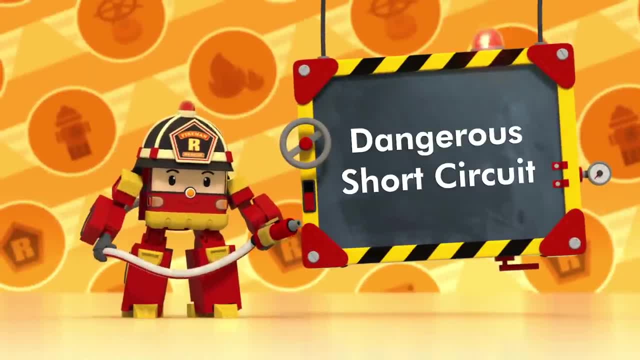 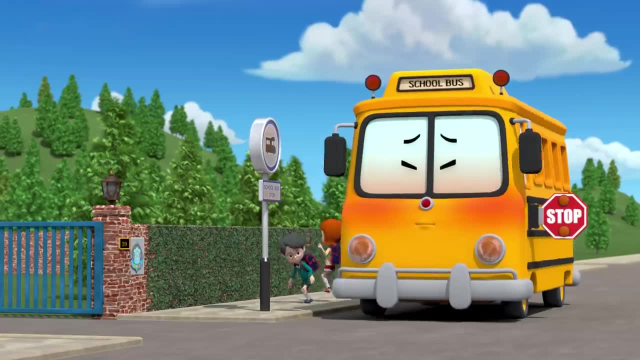 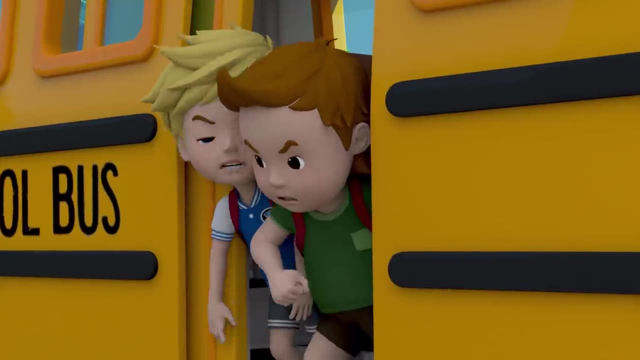 Dangerous Short Circuit. Oh, Oh Achoo. Goodness, Scooby, Are you sick? No way, I'm all right. Ugh, Let me off first. Jeez, I got here first, Just let me off. 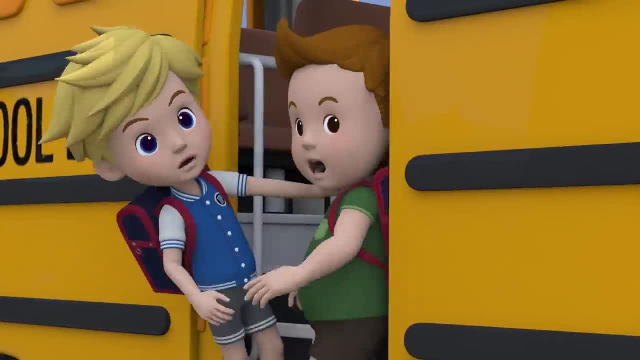 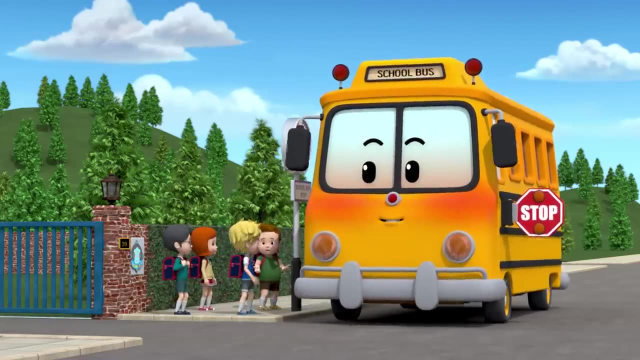 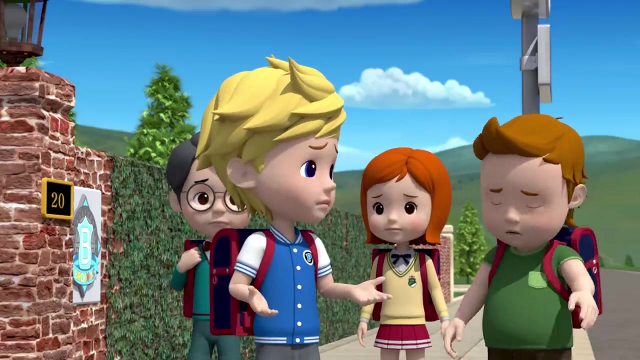 Cut it out. You guys are making Scooby feel even sicker. What Scooby Are you sick? Thanks, but I'm all right, guys, You don't need to worry at all. See you after a while. Scooby doesn't look good at all. 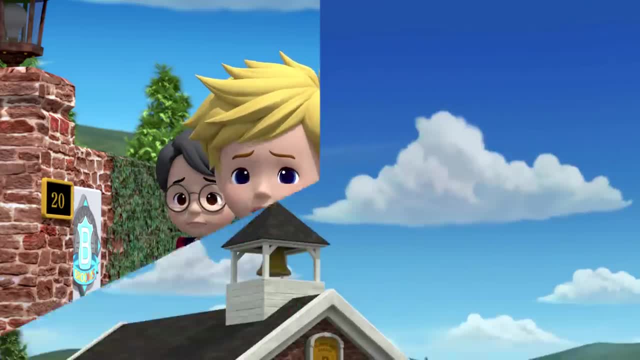 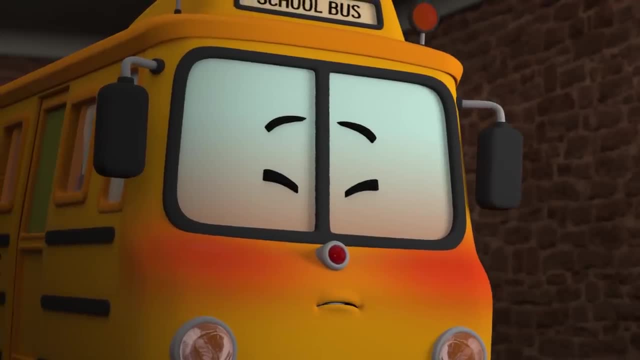 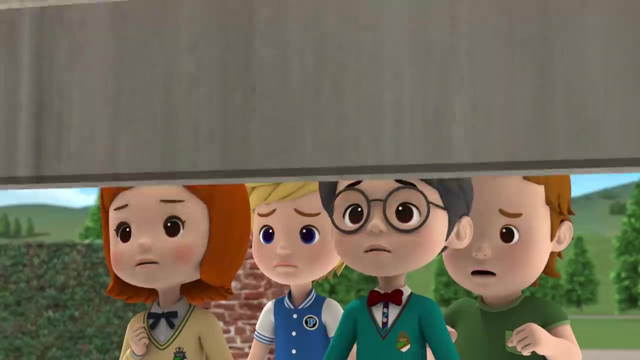 We made him feel even worse. Nice work, Hmph, Hmm, Hmm, Hmm, Hmm, Scooby Scooby, Huh, Kids Hi Scooby Scooby Scooby. we were really worried about you. You were 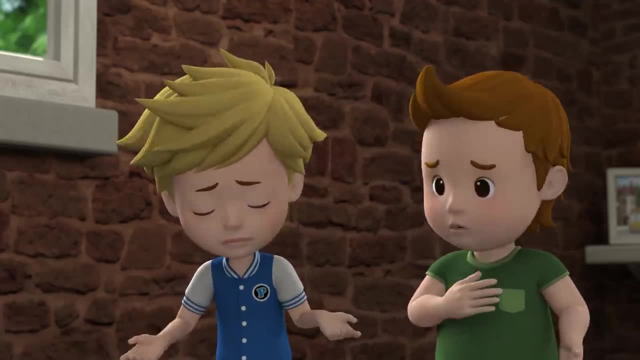 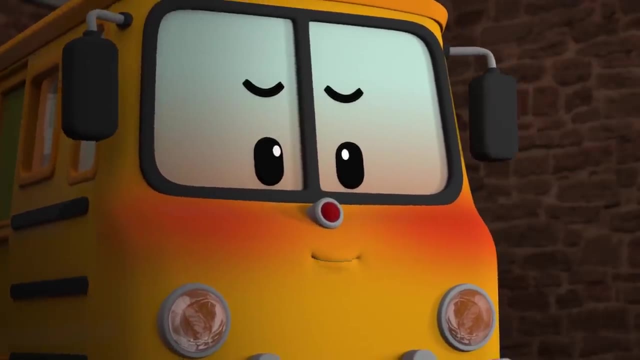 Scooby, we're sorry for earlier. Yeah, we're sorry. I didn't know that you were sick. It isn't your fault at all, guys. I've just got a little cold. I just need rest. Ha ha ha. 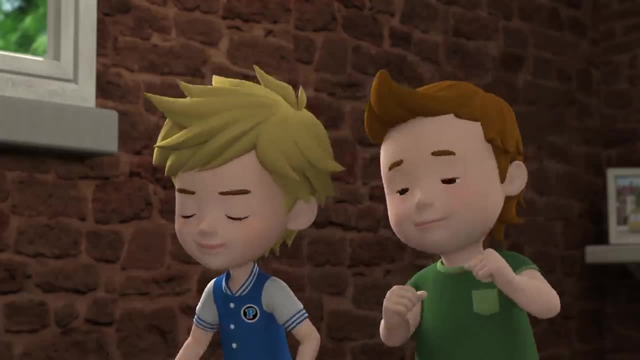 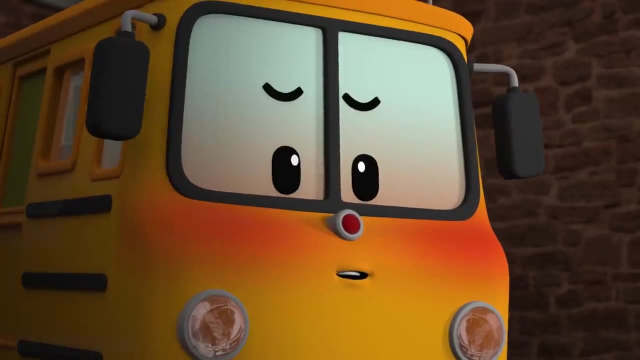 But thank you all for coming by. Scooby, Wait, There's more. We brought you some get well stuff. Huh, Just leave it to us, Scooby. We'll take good care of you until you get all better. Yes, we will. 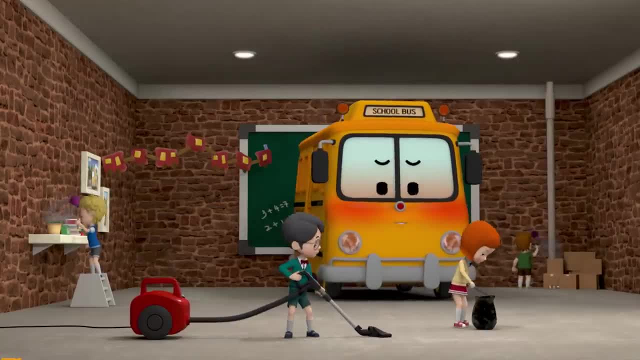 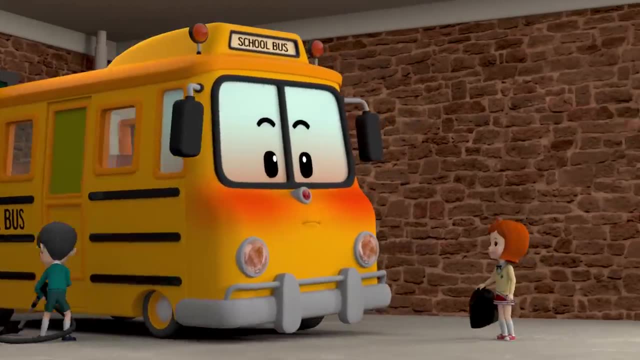 Hmm, Huh, Hmm, Hmm, Huh, Scooby, can you please lift your tire up? All right, Scooby. where do you put your garbage? Just right beside the door there. Ha ha ha, Hey, that tickles a lot. 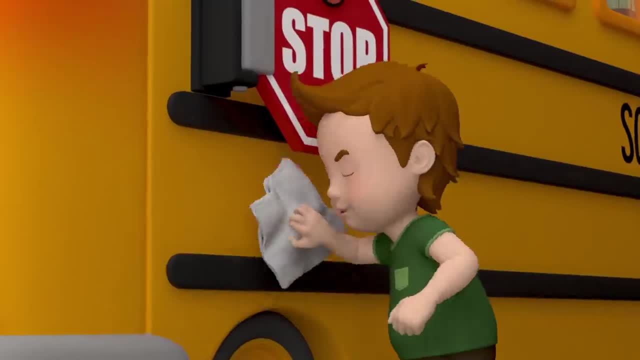 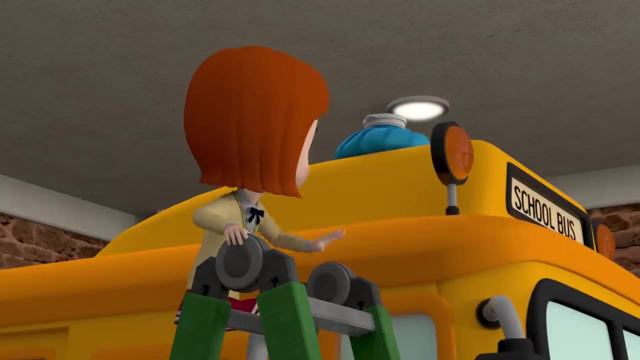 Ha ha ha. Ugh, There's dust everywhere. We'll freshen you up, Scooby. Ha ha ha, I can't take it. you guys Stop. Ha ha ha, That's cold. Huh, There, Scooby. 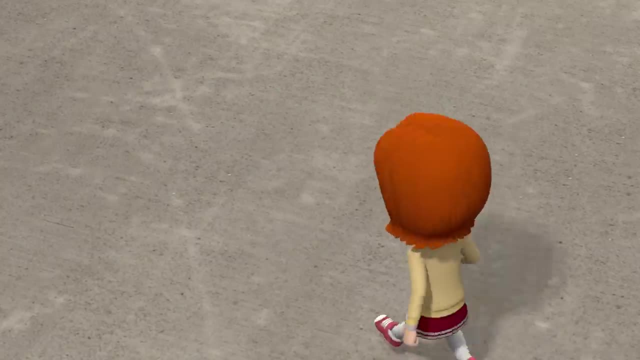 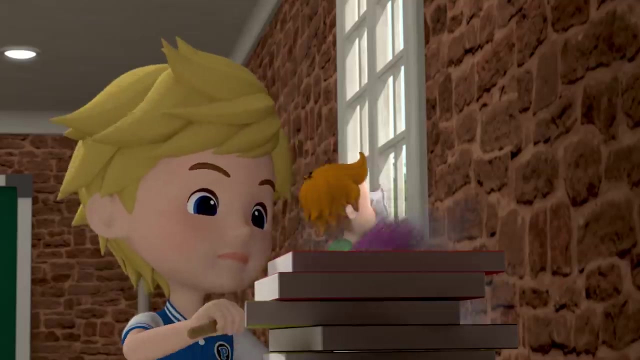 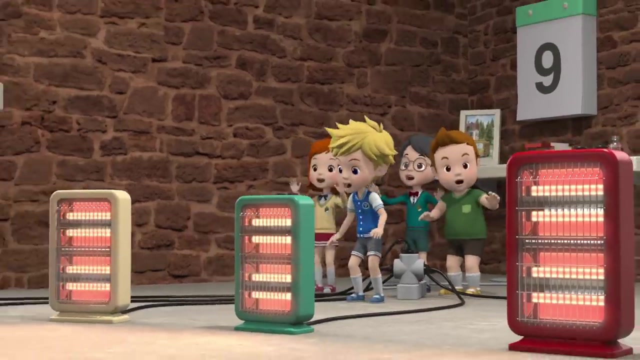 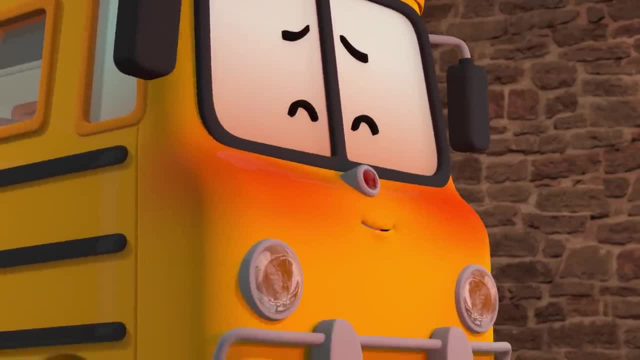 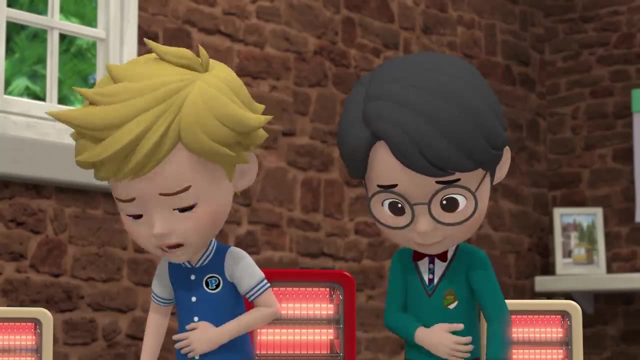 See ya down there, See ya, Look at that. It's so cool. Yeah, We made it back home. Goo Ha, ha, Ha, ha ha. There, Yeah, Great, We're good. Hum, hum, hum. 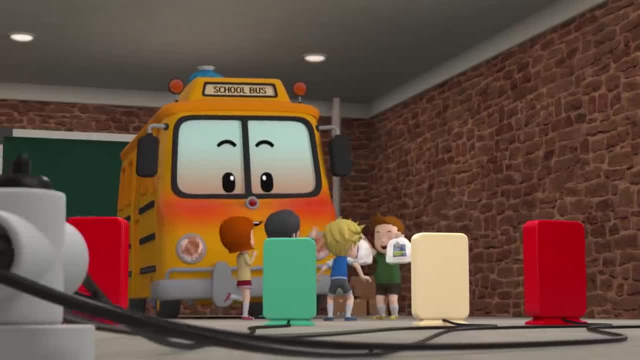 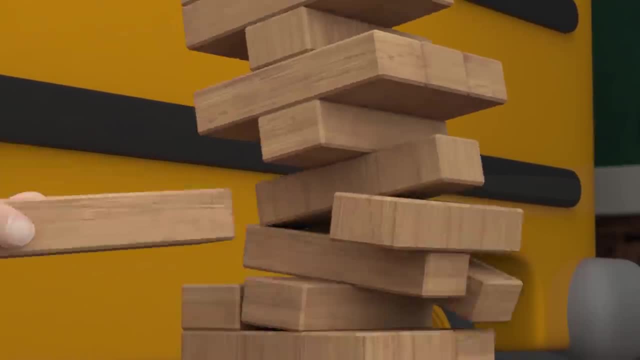 Nice and warm. Thanks very much, you guys. You're very welcome. Ha ha ha, Feel better, Scooby Goodness, I'm really hungry, Me too. Yeah, Good thing I thought to bring A whole bunch of awesome snacks. 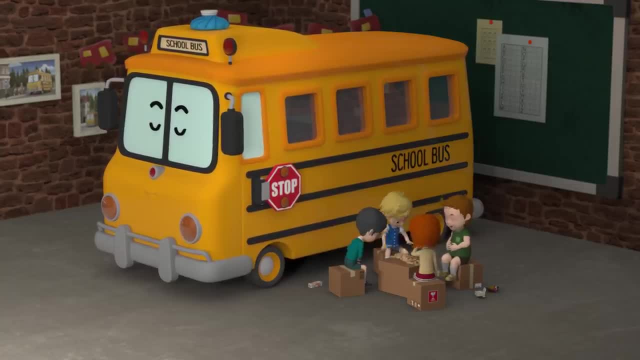 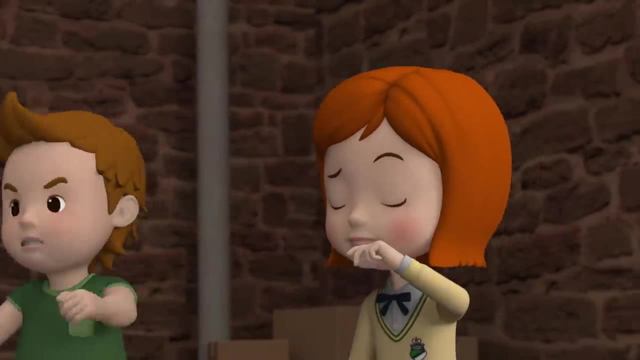 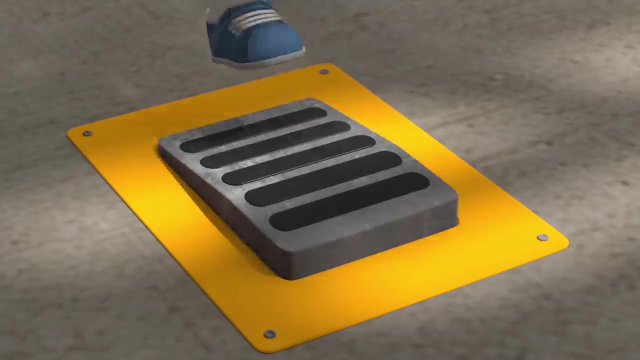 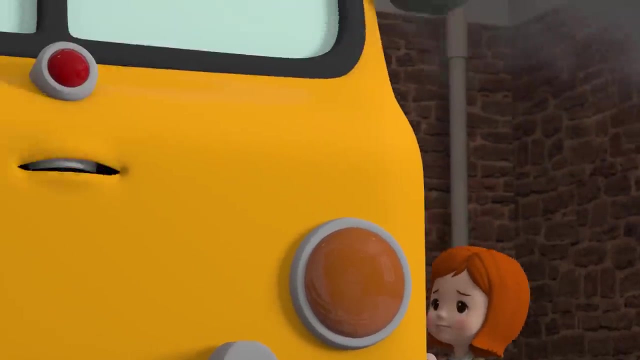 Ha ha, Oh, and there it goes. Hey guys, anybody else smell that? Johnny, stop eating bead dicks. Hey, it's not me. Huh, It smells like fire. Huh, Scooby, Oh, please wake up. 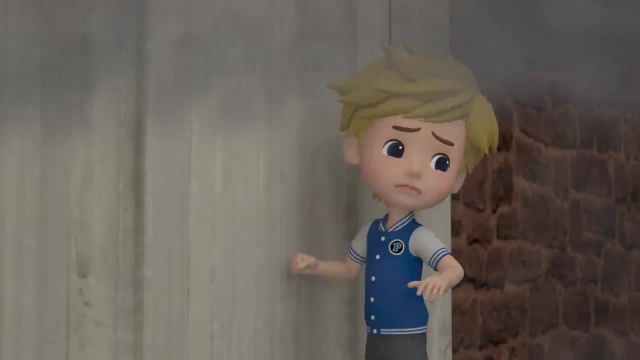 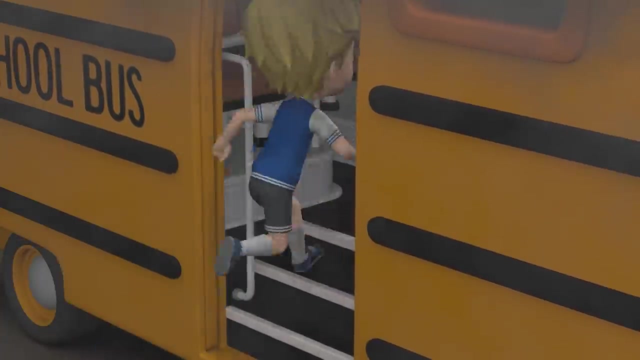 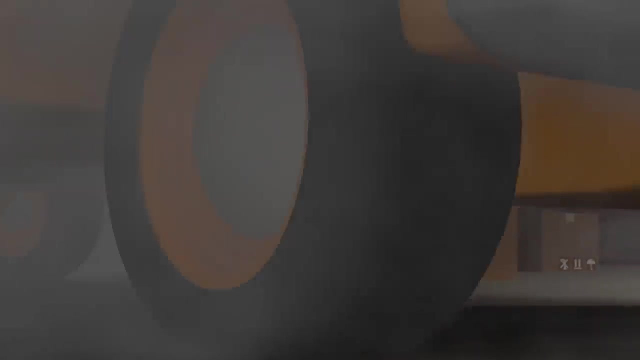 Oh, it's a fire. The door won't open. Scooby Children, hurry, climb aboard Now, put on your seat belts and hold on tight. All right? Huh, Smoke Seems to be coming from Scooby's place. 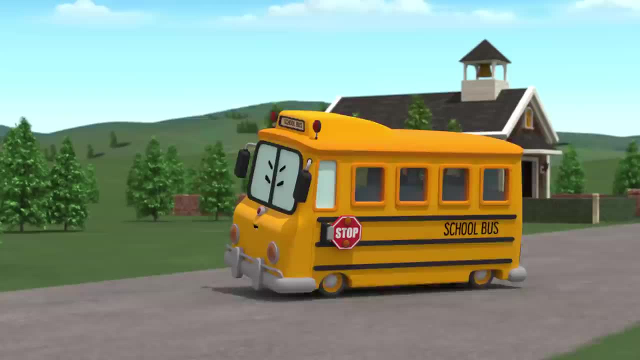 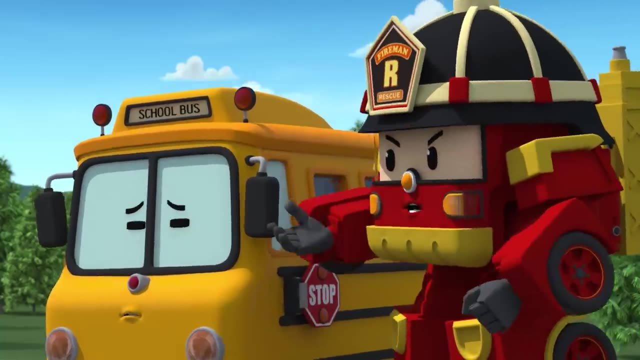 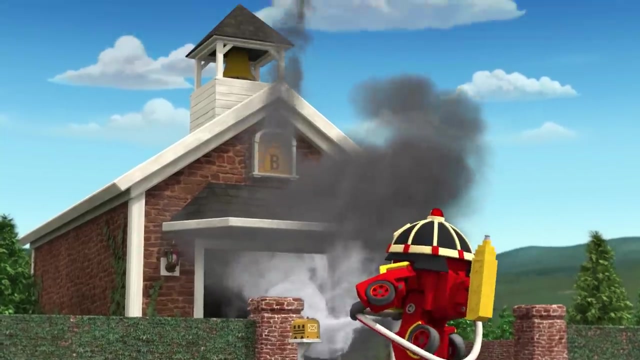 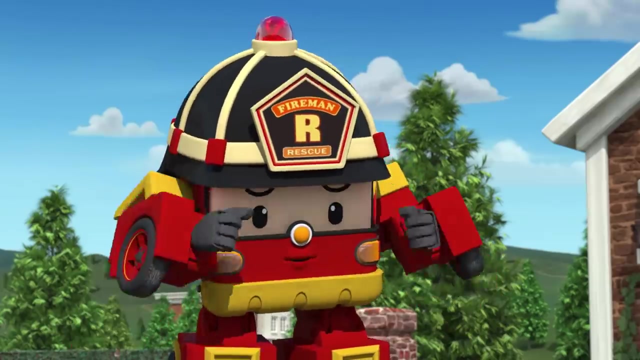 Look out. Ah, Ah, Ah, Ah. Now, please take the children somewhere safe Right away. Hmph, Huh Now then. Ah, That's what happened. It's really good to think of your friends, but you must use your electronics with care. 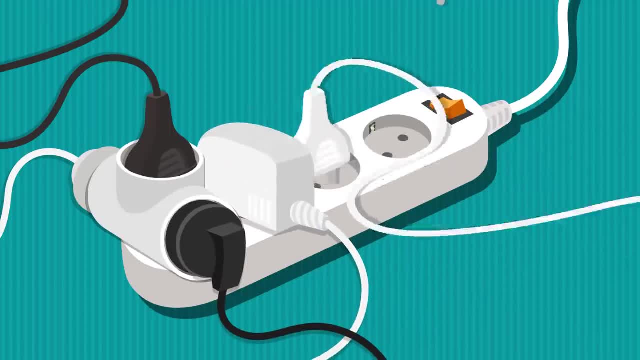 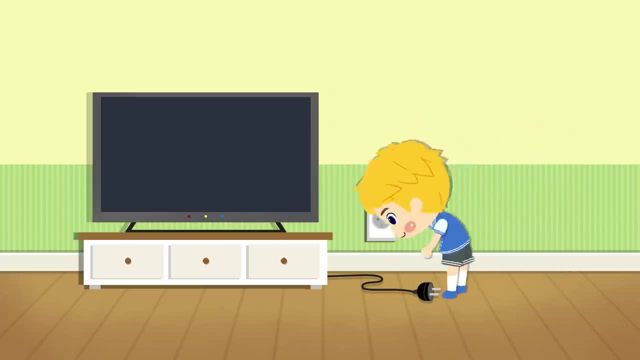 When you plug in devices, don't plug in too many at once. That much current flowing can overheat the outlet, which can lead to a fire. Also, loose plugs can be dangerous. Plugs that aren't pushed in all the way can cause sparks to occur, which can also start fires. 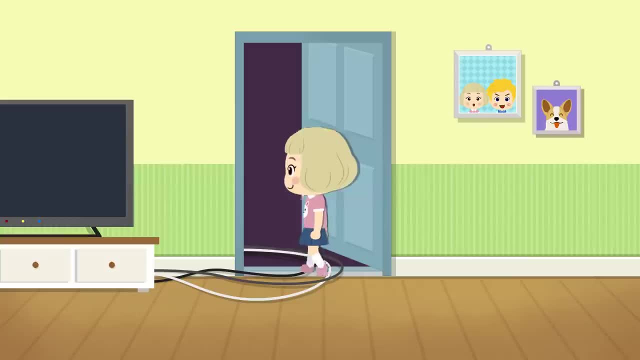 Lastly, make sure the insulation on the wires doesn't peel off and that water never gets in the plug. A short circuit can cause a fire too, Do you understand? Yes, Thank you Roy. Uh, sorry, Scooby. 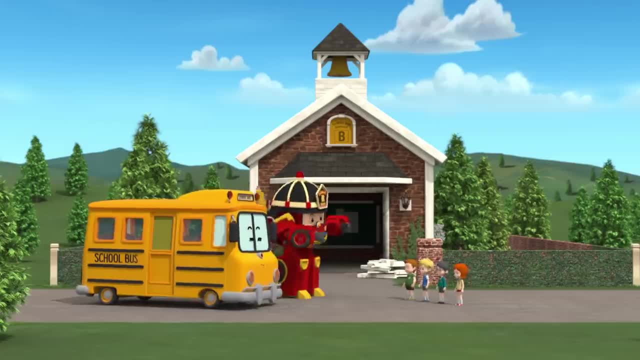 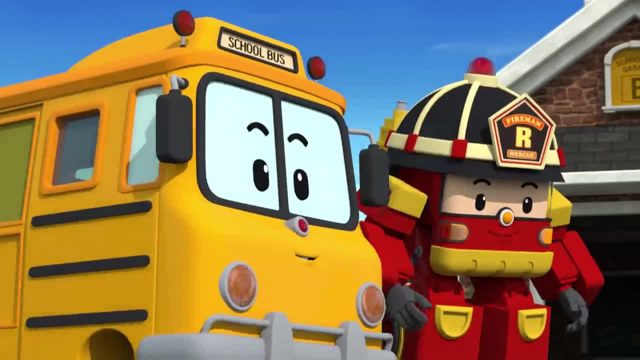 I'm glad you're okay, Scooby. I'm glad you're okay, Scooby. I'm glad you're okay, Scooby. It's fine guys. You made me feel so much better. I'm not sick anymore. You're not. 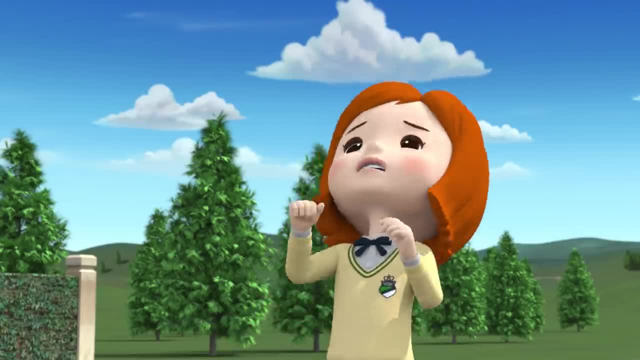 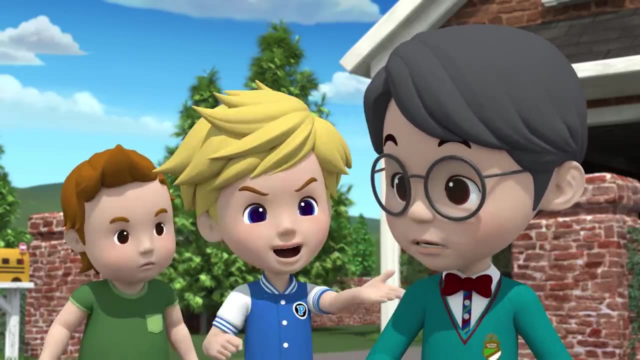 Awesome, Gee Scooby, that's great. Achoo Huh, It looks like you might have come down with Scooby's cold. Oh yeah, Guess it's Cindy's turn. right, Cindy, we're here to help. 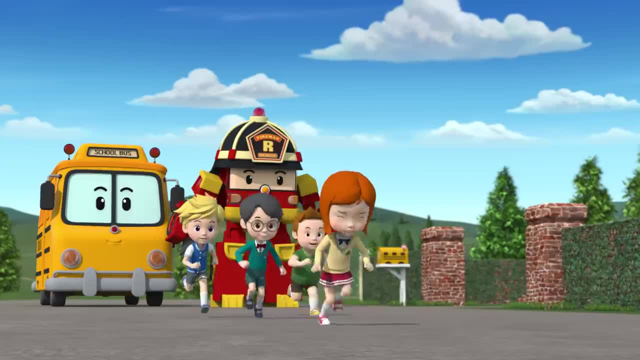 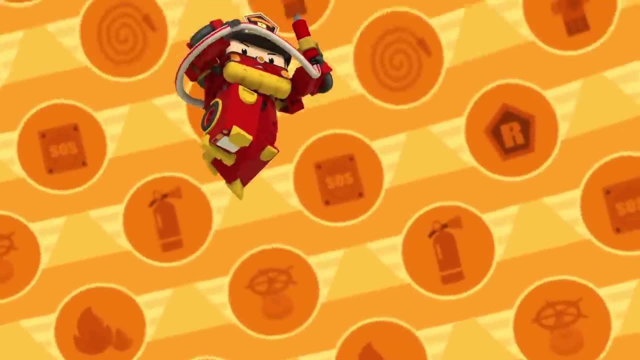 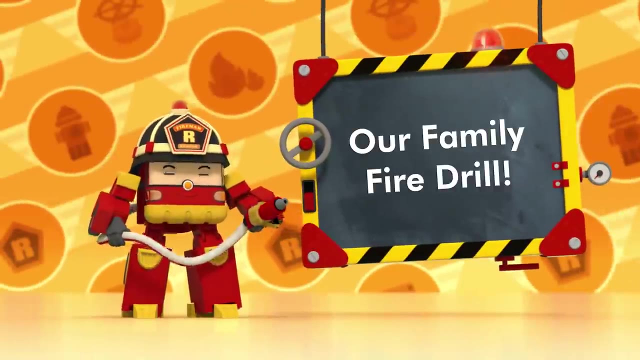 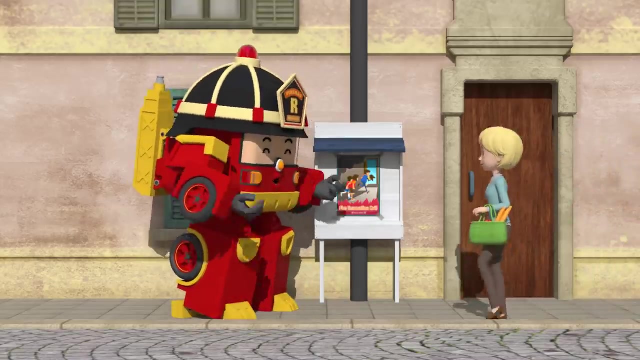 Uh, I'm fine. thanks, I'm very fine, Cindy, Bye, Bye, Cindy Bye, Our Family Fire Drill. Have a nice day. Oh, hi, Roy, Afternoon, What's that? Fire evacuation drill, Yup. 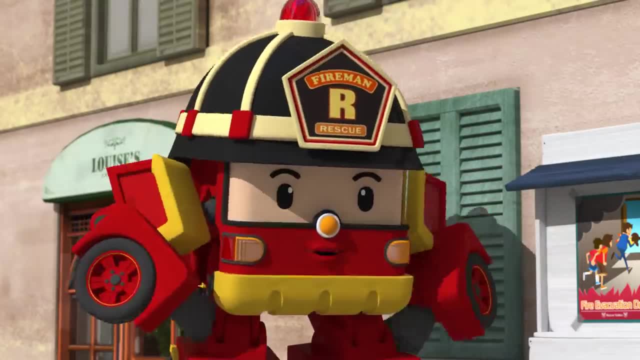 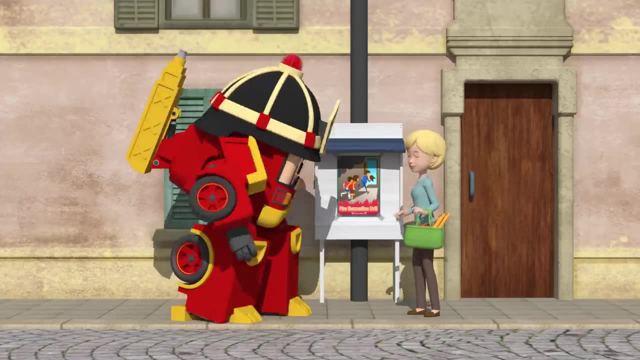 Families can all do this program, practice fire drills and make a plan so they know just what to do If they pass. they get a safety badge too. Oh, that's great. Would you like one, Roy? Huh? 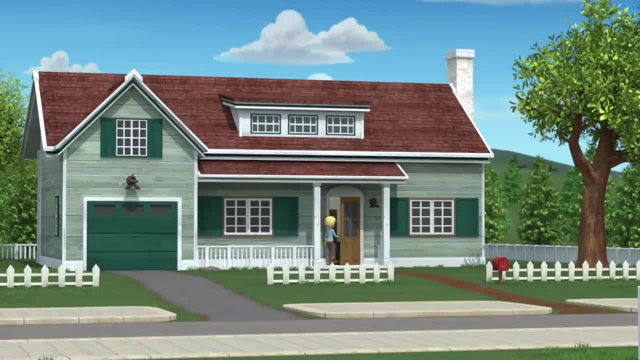 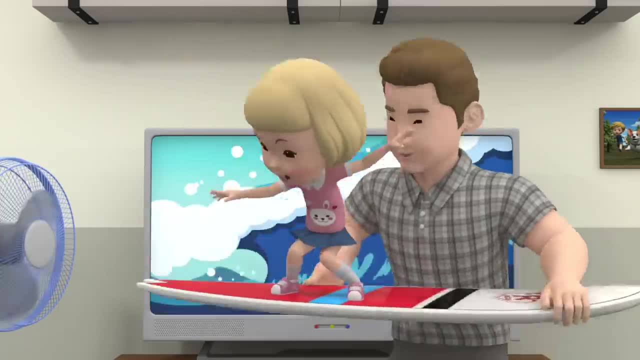 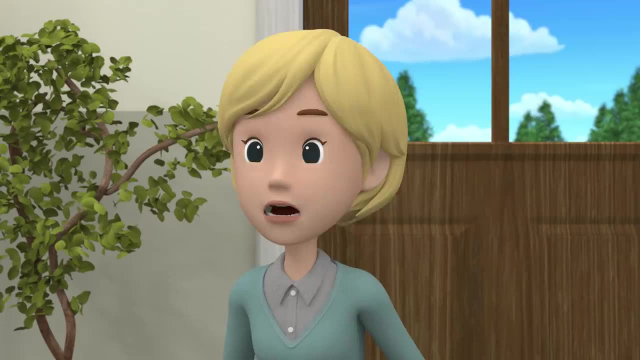 Hmm, Whoa, What are you doing, Hey? Oh Whoa, Oh, Whoa, Whoa, Oh, Whoa, Whoa. What's that? Whoa, Whoa, Whoa, Whoa Oh. 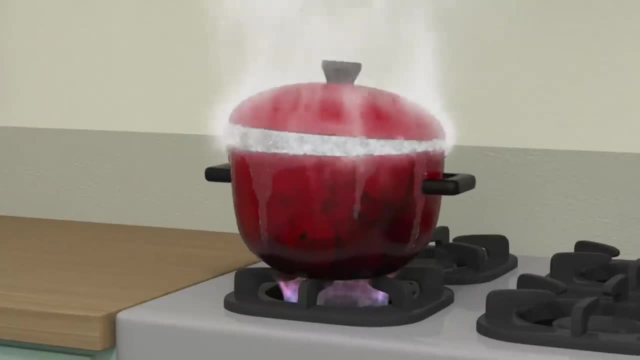 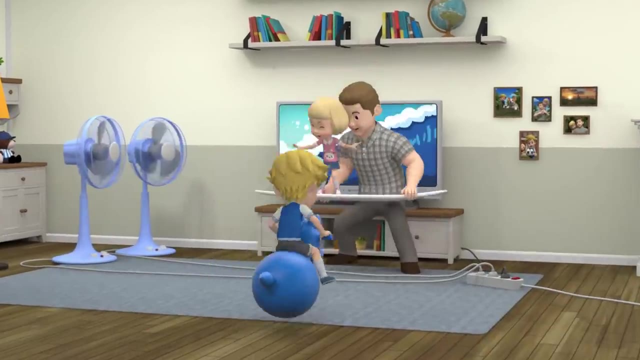 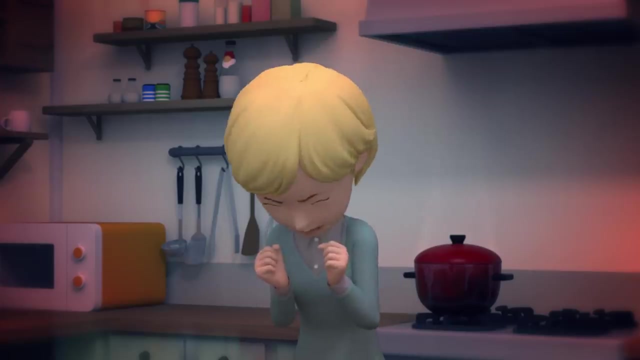 Whoa, Oh, Oh, Oh, Whoa, Oh, Oh, Oh. Goodness, what's going on? No, No way I have to straighten this mess out. Oof, Oof, Huh, Huh. 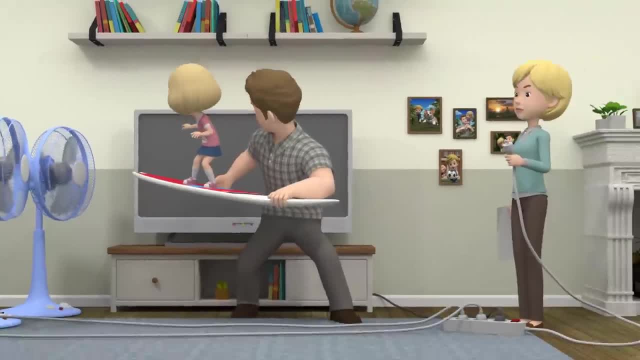 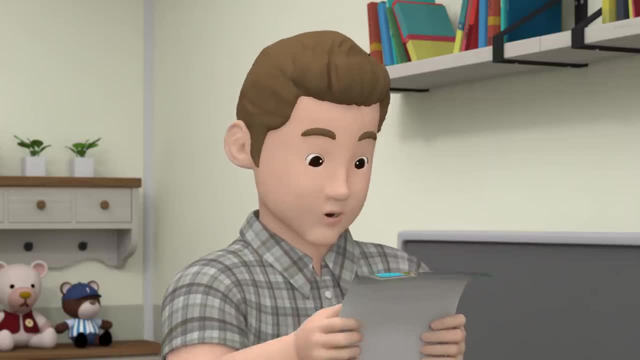 Honey, you came home Here. look at this: Huh, Family fire evacuation. Wow, what's that? Seems like a lot of fun. Shall we do it, Yeah, Yeah, I wanna go too. Oh, So everyone agrees. 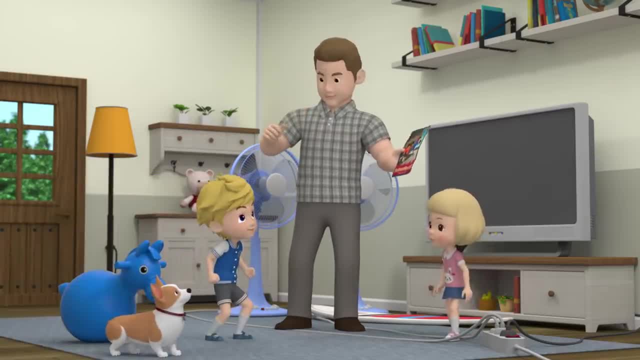 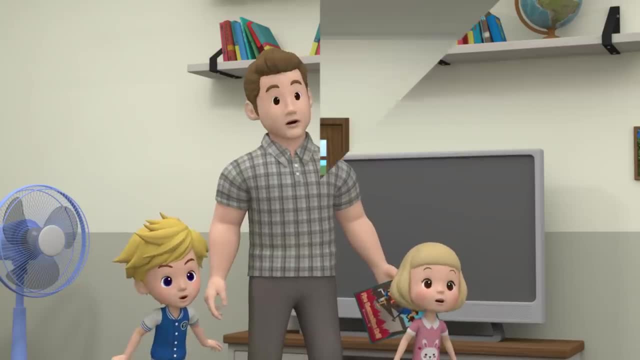 Yeah, I wanna go too. So everyone agrees: How great Drill. start now. Huh, In one week we'll be participating in this drill program. Let's do our best to try and stay safe in the event of a fire. 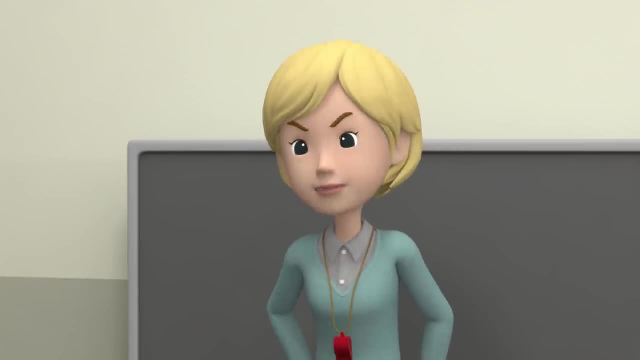 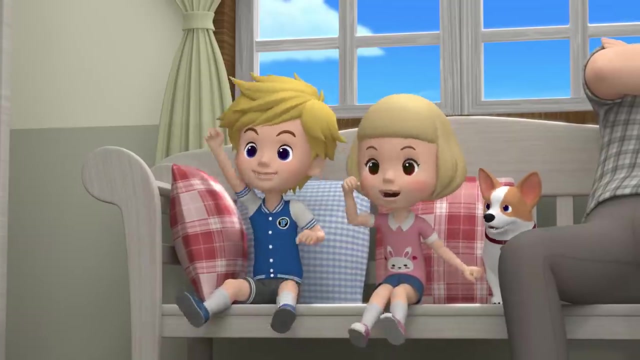 Let's do our best to try and stay safe in the event of a fire. Got it, Yes. So everyone, look at this map here. Who can tell me how many exits our house has? I can, I can, Huh. 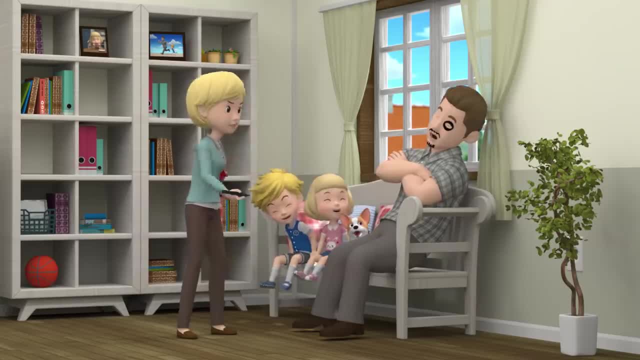 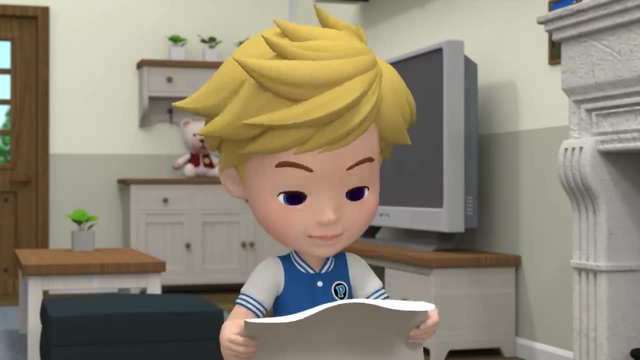 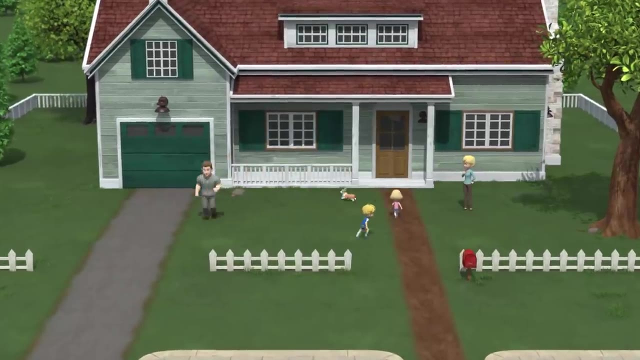 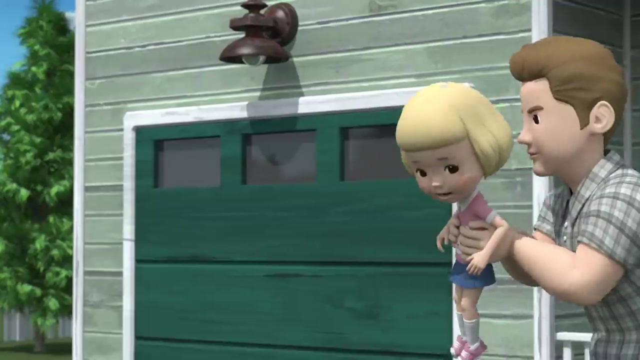 Huh, Hahaha, Okay, what's next? Okay, what's next, Don't know, I think Ah, Back door, Lucy. Okay, Ah, Ah, Ah, Ah. Ah, Daddy, Don't worry, Dad will always be there to save you. 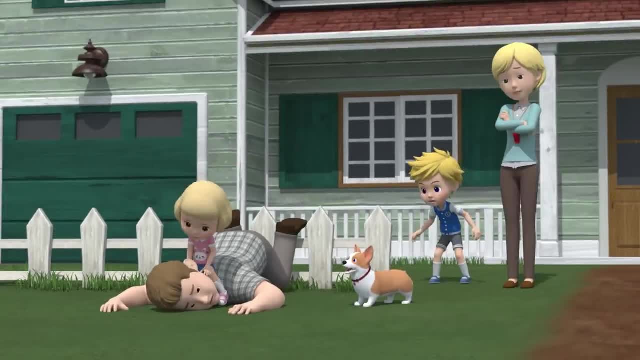 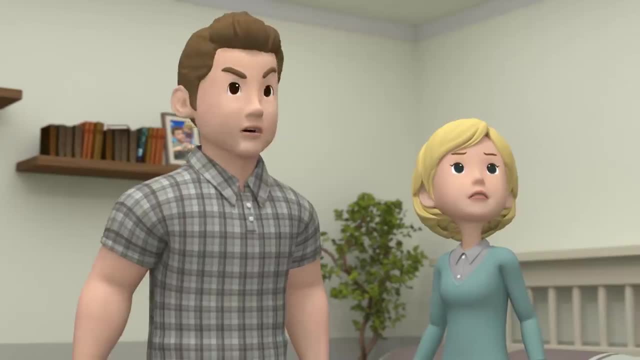 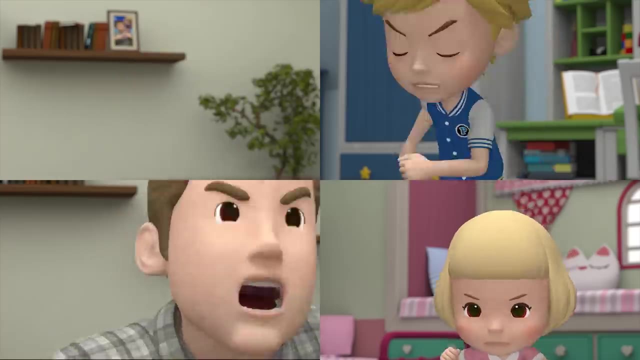 Ah, Oh, Ah. Okay everyone, The test will begin shortly. When the fire alarm starts, you have three minutes to get out of the house Ready Set. Ah, Ah, Huh, There's smoke, Get down. 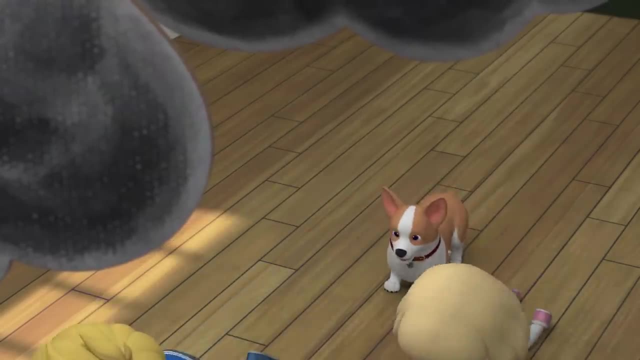 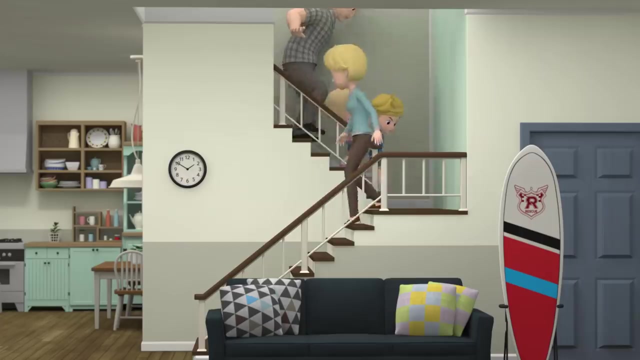 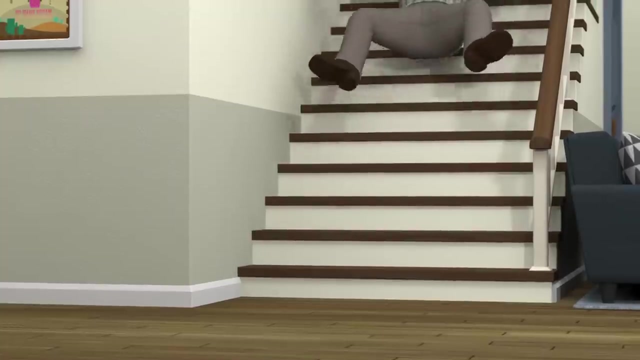 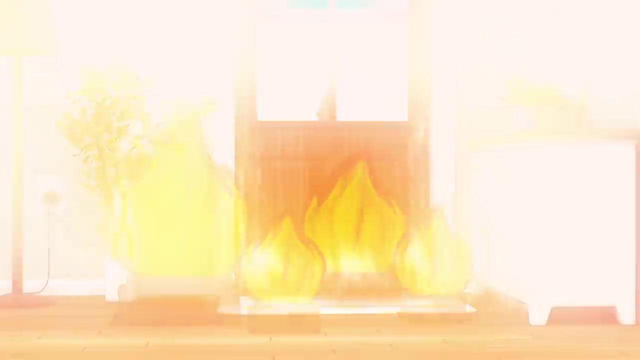 Huh, Huh, Don't be nervous, you two Just do what we practiced, Got it? Yeah, Go to the first exit. Uh, Uh, Uh, Ah, Oh Daddy, Front door's on fire, No good. Option two: 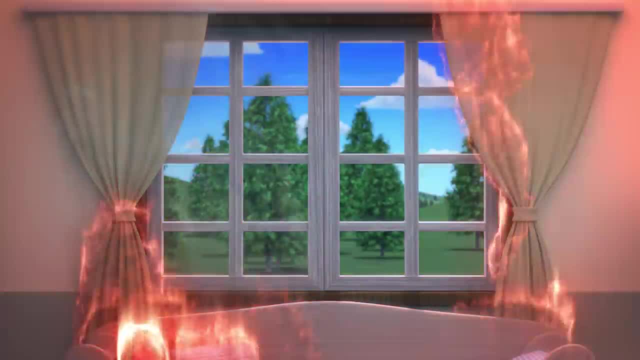 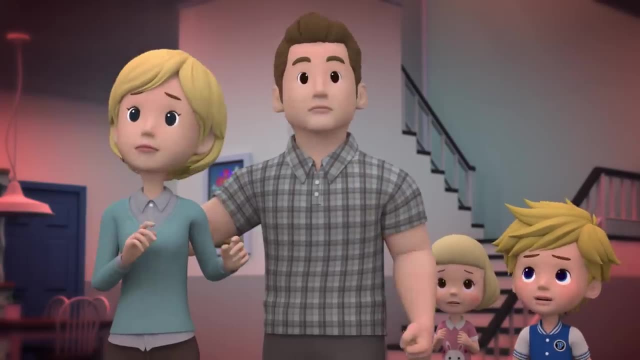 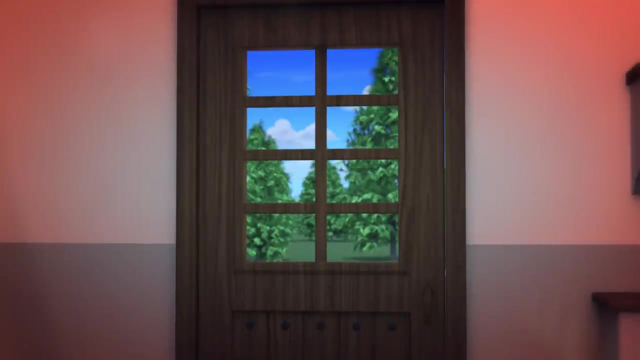 The window, The window. Ah, Honey, The window's blocked too. It's all gonna be fine, We'll find a way out. Thirty seconds remaining. Ah Mom, The back door, The third exit. That's right, The back door. 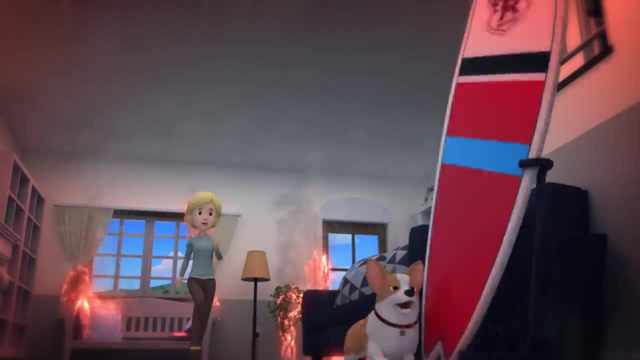 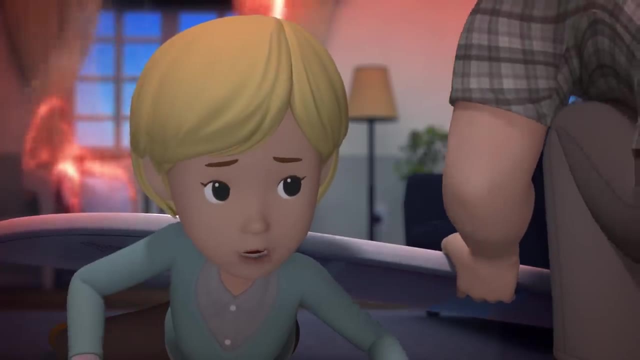 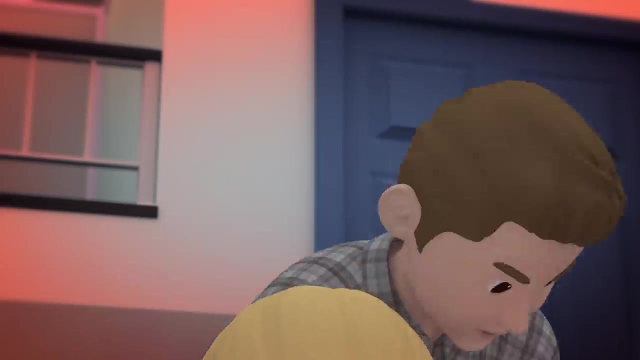 Okay, Come Hurry. Okay, Ah, Huh, Sarah, Ten seconds, I don't think I can make it. Leave me, Take care of our children. Don't be ridiculous. I'll never leave you behind, Ah. 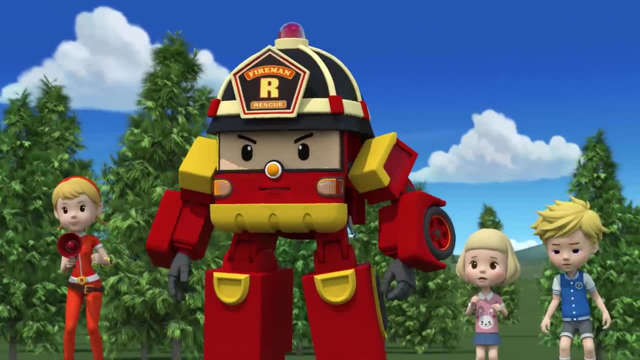 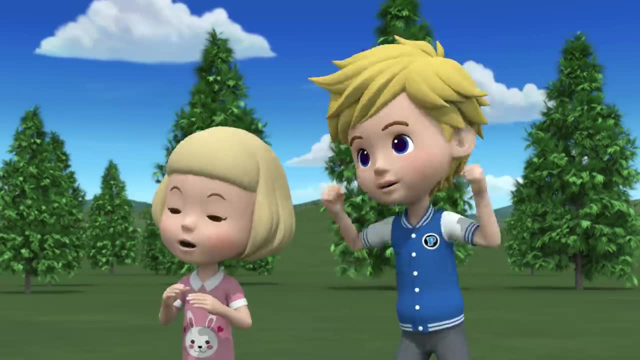 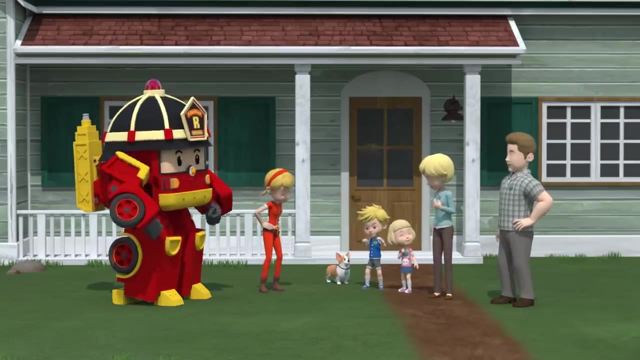 Ah Ah, Three, two, one Congratulations. You all made it. Wow, Awesome job, Dad. Phew, There you go. Wow, You were able to react quickly with every situation that arose, Often when there's a real fire. 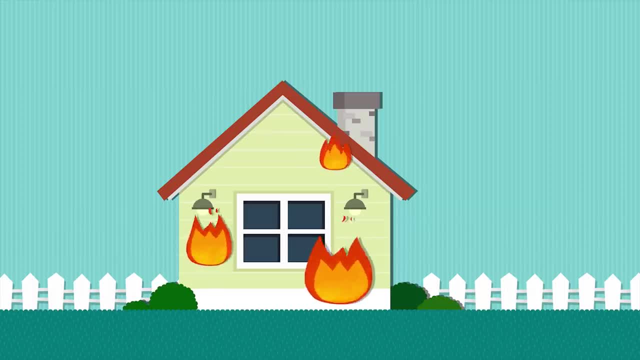 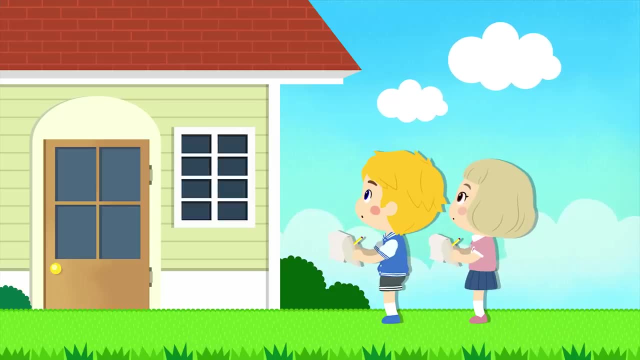 people will panic and forget their safety rules. It only takes five minutes for a fire to spread to dangerous levels, so always remember your evacuation plan. Make a map for your family that clearly marks all emergency exits. Everyone should pick a safe place to meet after evacuating. 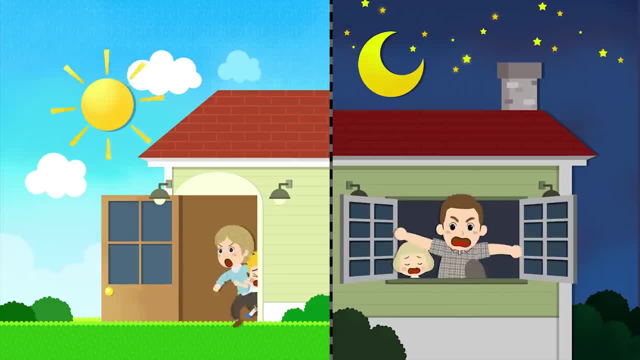 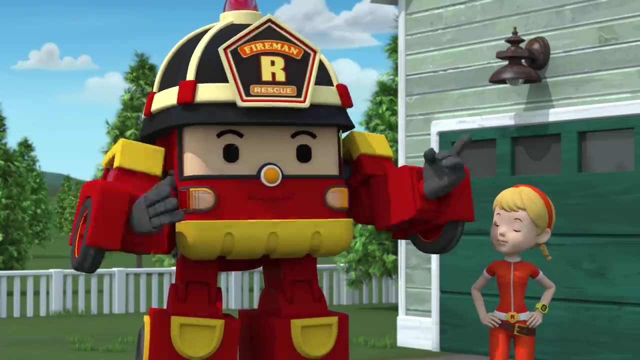 Twice a year you should have an actual fire drill with your family. It's good to try it both during the daytime and at night. That way, if a real fire broke out, you know you'd be able to get everyone out of the house safely. 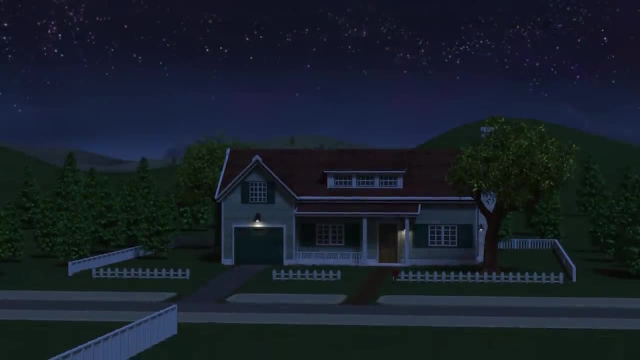 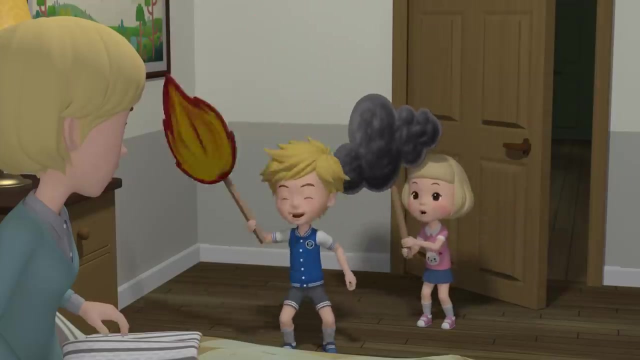 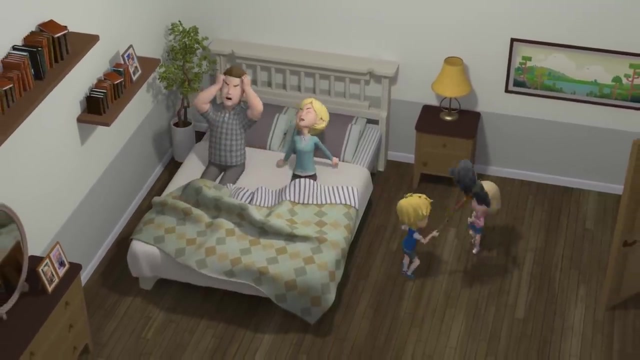 Good to know. Ha-ha, Oh, Fire, Fire, Fire. Where Fire? drill time again. Roy said we need to do a drill at night too. Let's go. No, you didn't mean right away. Hmm, Hmm. 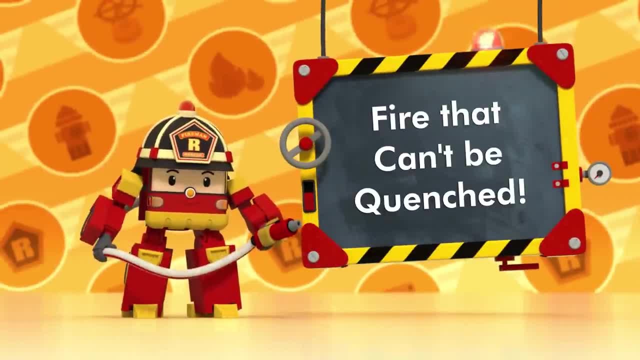 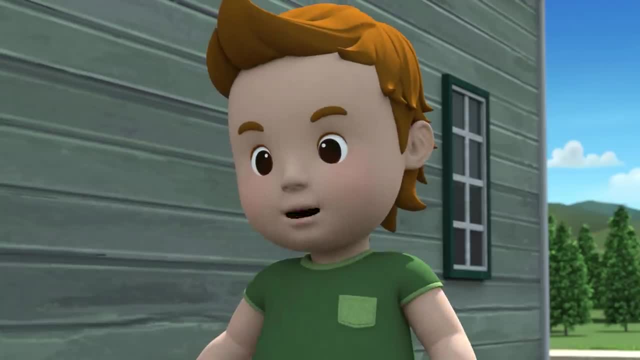 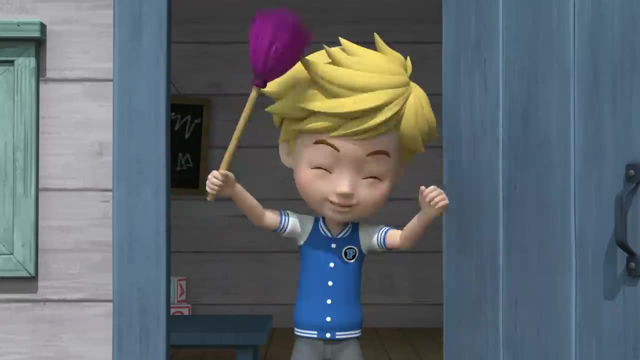 Hmm, Fire, That Can't Be Quenched. Charles, looks like I'm all done. How about you? Yeah, I'm just about done. It's all clean. What's with you two? This is your fault. Yeah, My bad. 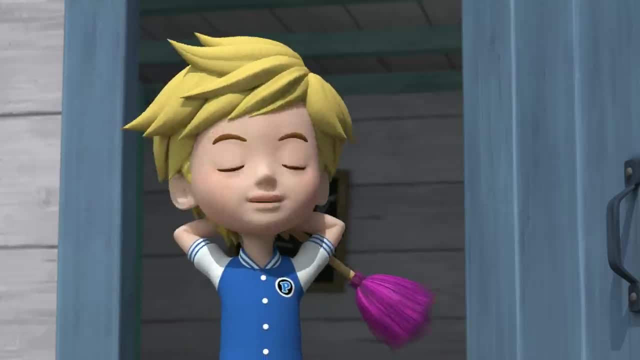 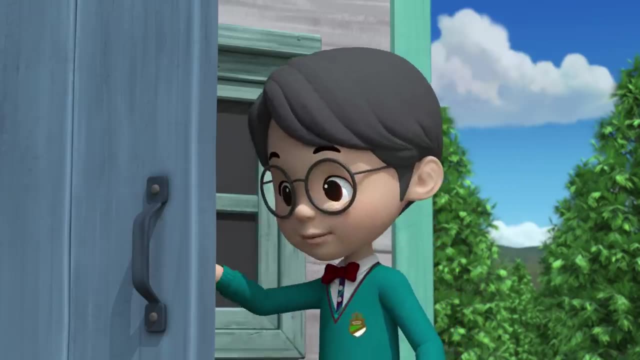 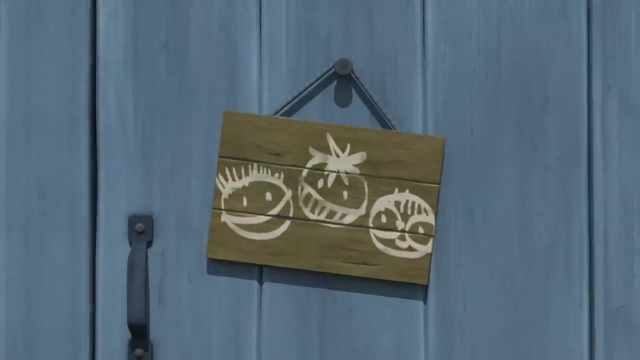 Anyway, I'm all done cleaning. Come in, Yahoo, Hang on. One last thing: Finished Ta-da, All seven episodes of the newest Super Dragon series. Hmph, That's cool, but Ha-ha, It's only the best. latest ninfrendo. 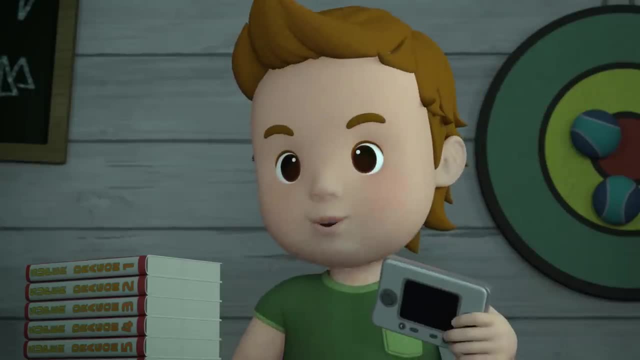 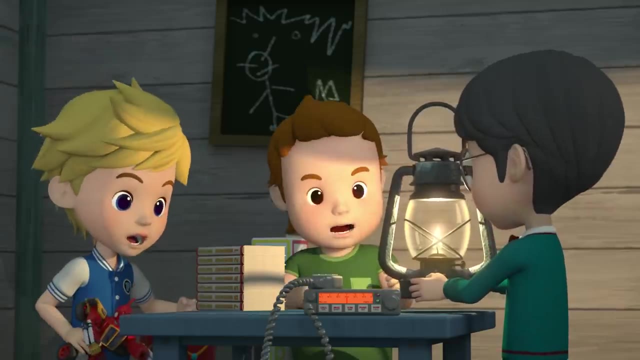 Ow, Beware my Super Dragon fist. Huh, Wow, What's that, Charles? It's called an oil lamp That looks super old and studded. Oh yeah, It's a little bit old. It's a little bit old. 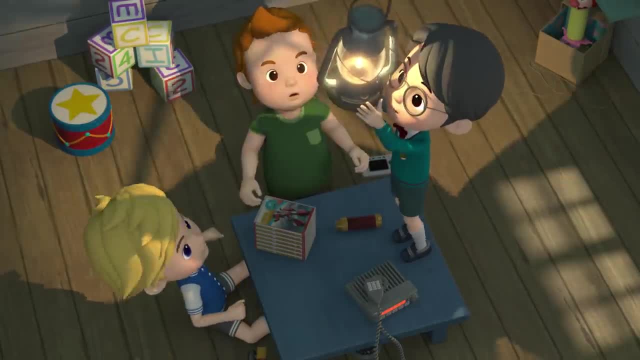 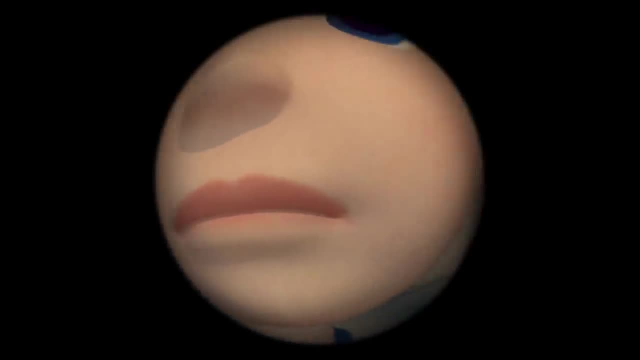 Yeah, My grandpa used it a long time ago. What's this thing? A telescope? Wow, Huh, Hmph, Whoa Wait. What's this? My personal favorite, A ham radio. Ham, It's great. 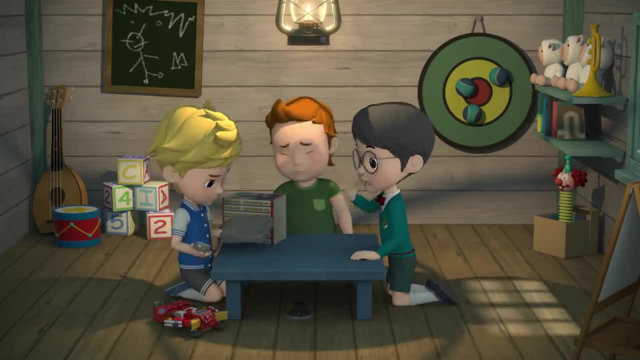 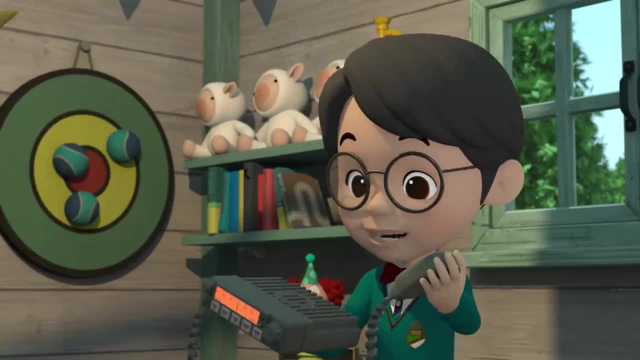 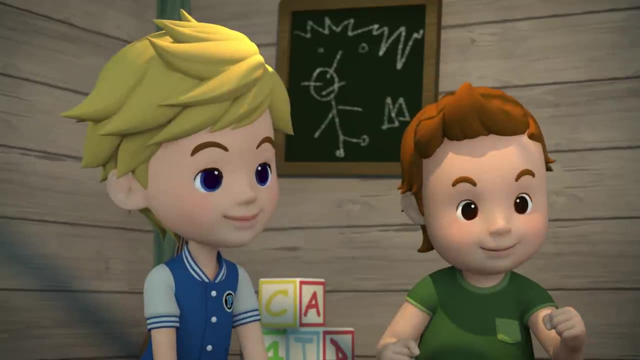 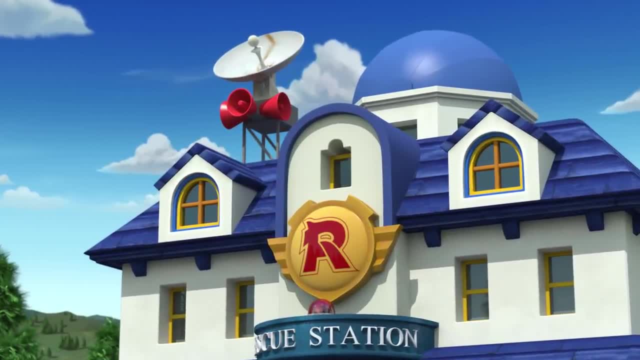 Let's try it. Let's try it now. Let's try it, Let's try it now. Hello aliens, Do you hear me? Beep, boop, beep, Um, aliens, This is for the rescue squad. Aw man. 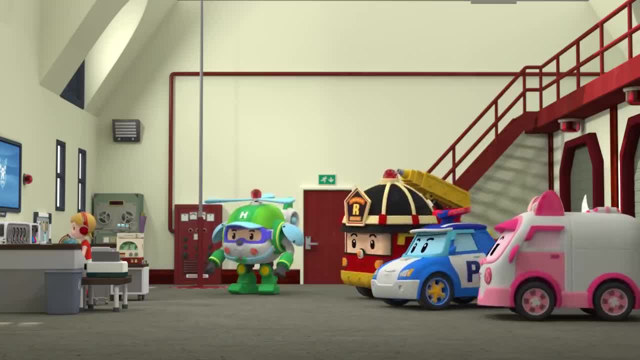 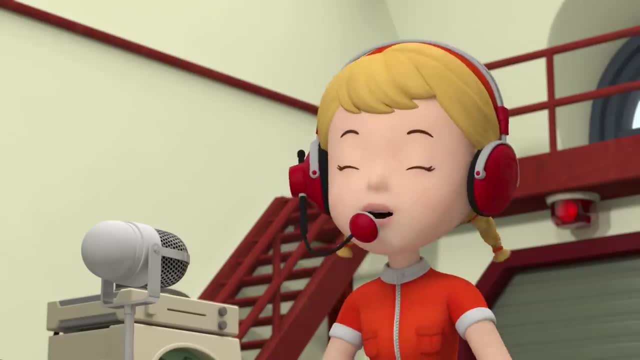 It's just the rescue squad. Hey, is that Charles I hear? Sure, is? We made a secret clubhouse at Peter's place? Wow, Clubhouse. Yeah, You guys should come over and say, hi, Ha, Sounds good. We can't turn down an invitation like that. 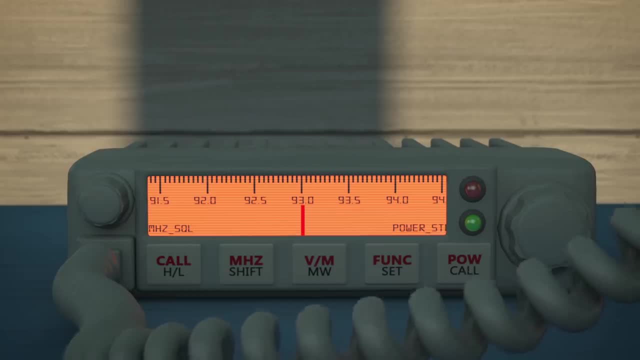 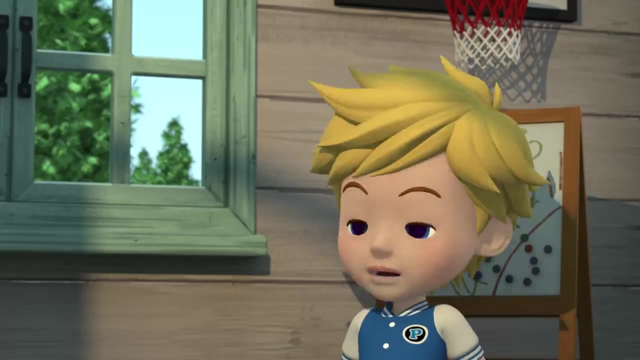 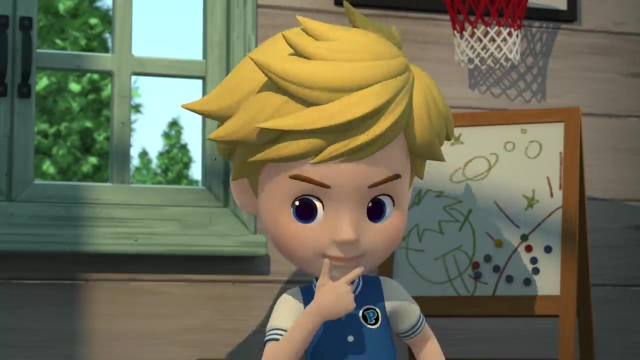 Of course, Aliens, do you copy? Hello, Hello, Do you copy? Oh man, It's not working. Huh, Aliens, That was just me needing food. I'm hungry too. Yeah, Maybe we should eat my super food stash. 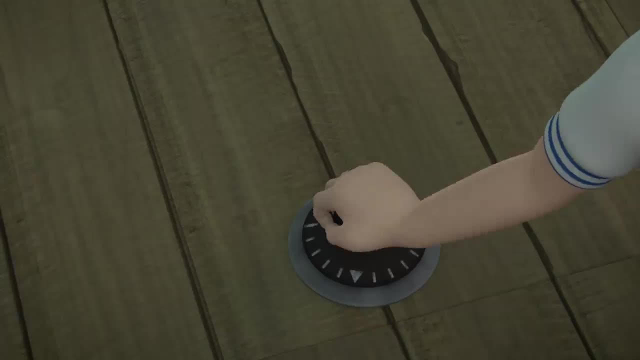 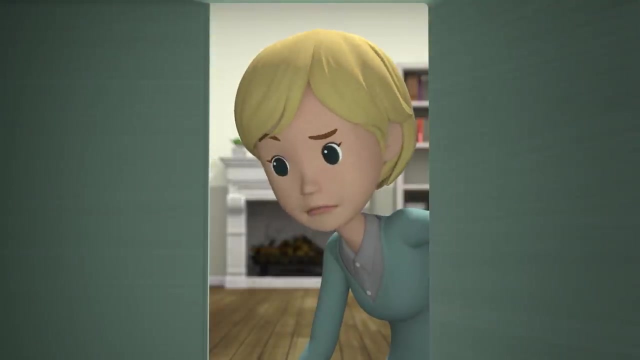 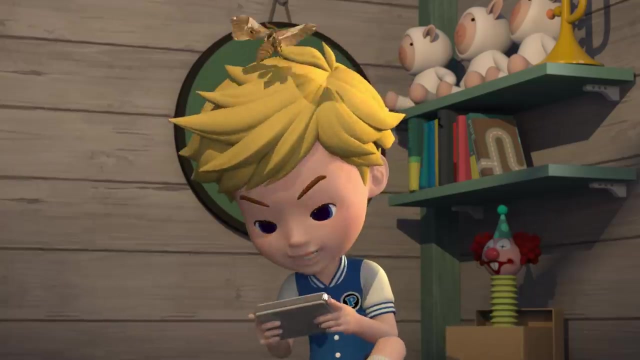 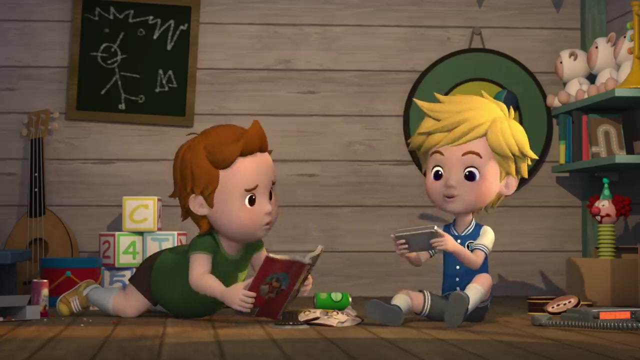 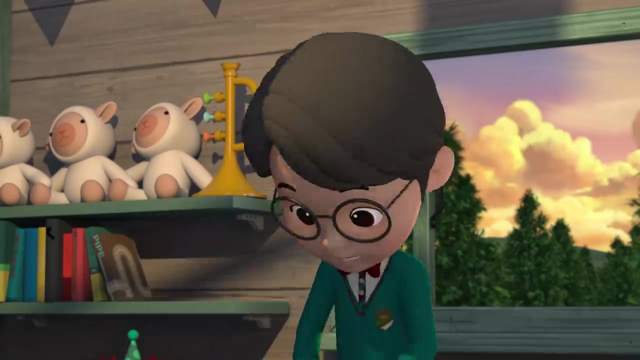 Food stash. Hmm, Awesome, Huh. Where are all the snacks? Mm, uh, uh, huh, Huh, Peter, quit messing around. What, Who me, Huh, Whoa, Is it aliens? But I turned the radio off, you guys. 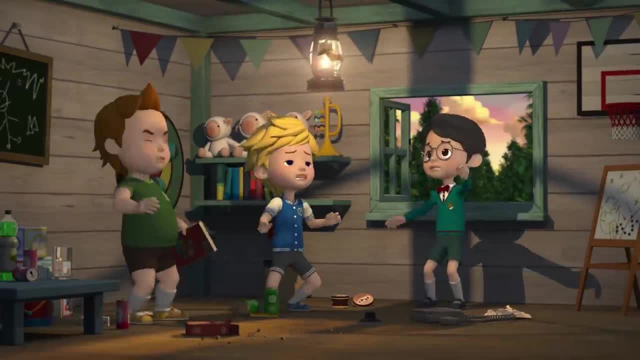 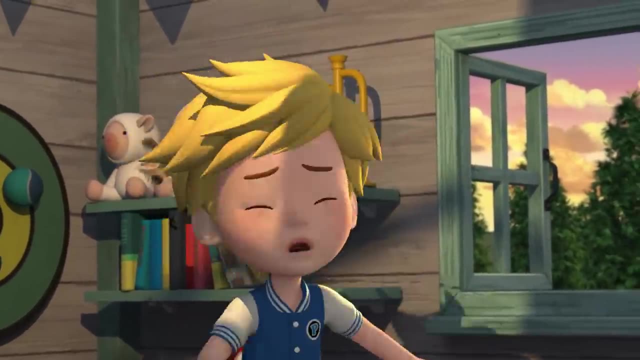 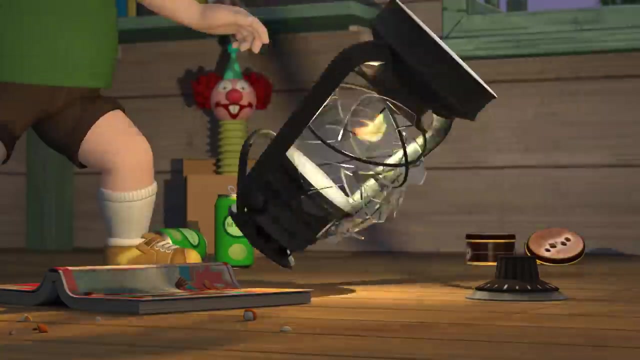 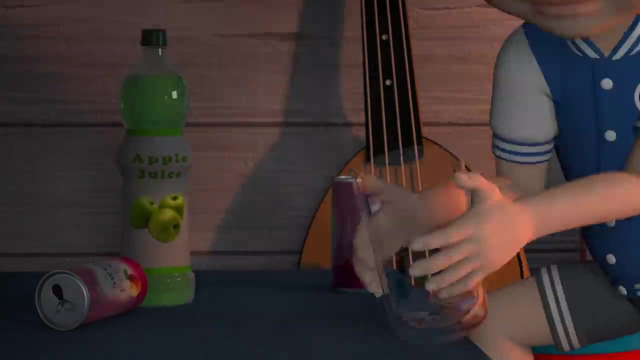 Ah, Get away, Ah, Get off, Get off. Whoa Whoa, Ah, Whoa, Whoa, Ah, Ah, Huh, Ah, Fire. No, It's on my comic book Water. I'll put it out with water. 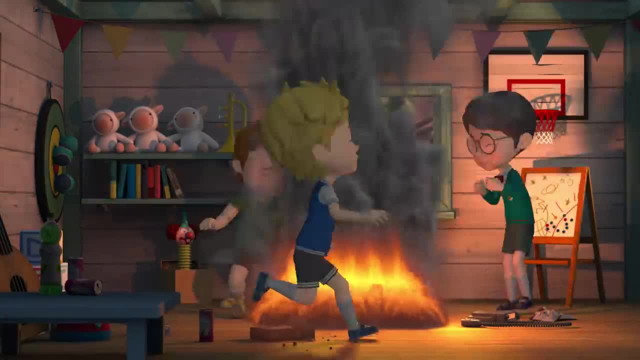 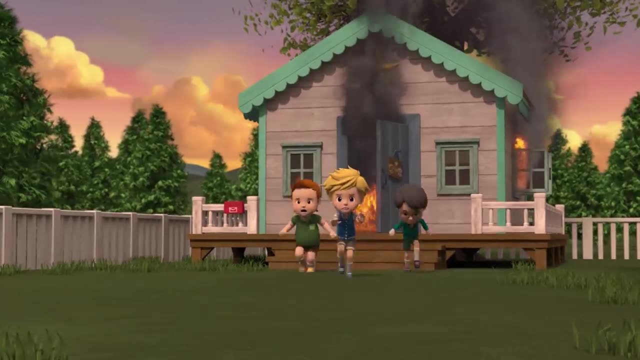 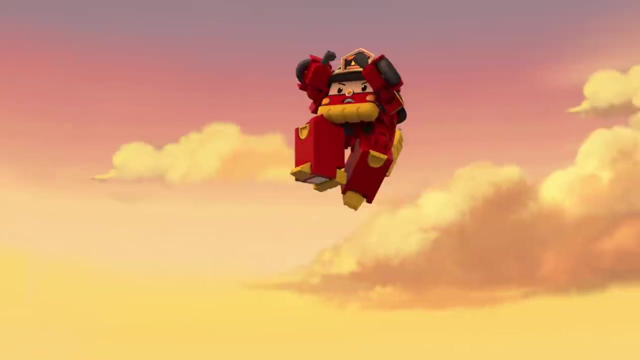 Ah, Whoa, Ah Ah Ah, Hey, kids, Dinner's ready. Peter, Ah Ah, Fire, Huh, Is that smoke coming from Peter's house? Oh, Huh, Hmm, Ah Ah, I'm here. What happened? 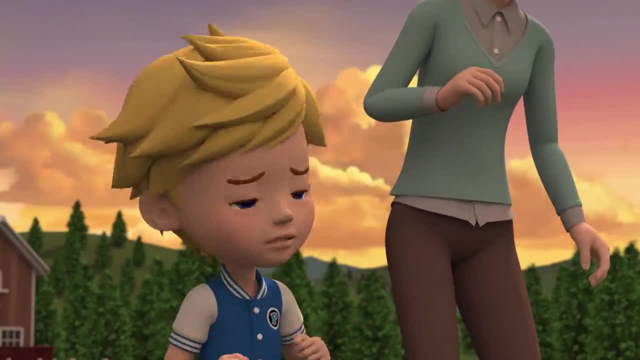 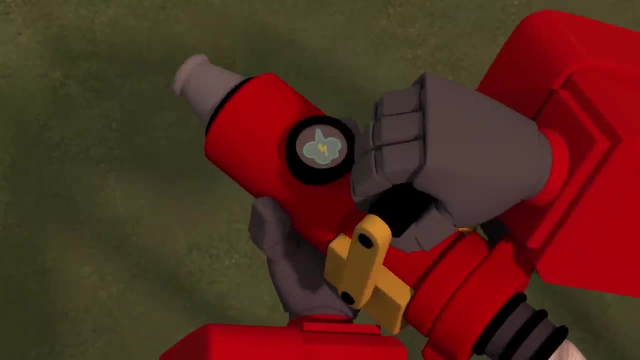 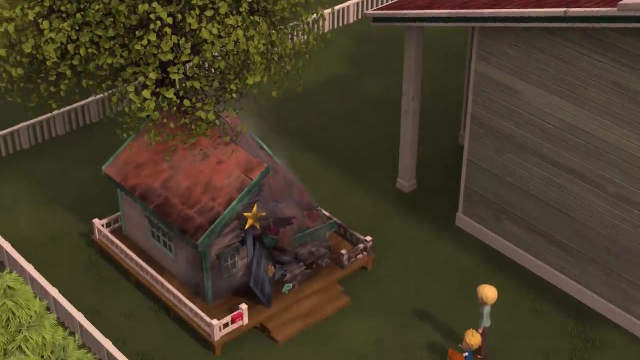 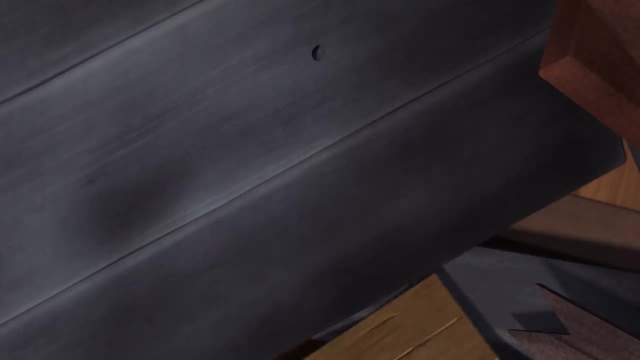 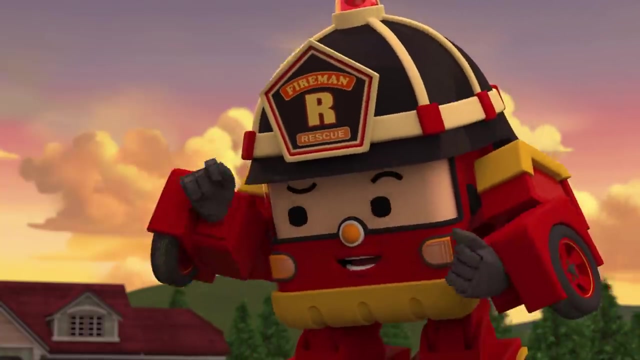 Ah, Ah, Ah, Ah, Oh, Ah. Uh, What's going on? I'm going to pay for this, but you're all safe? Listen: if a fire starts from oil, you should never pour water on it. Why? 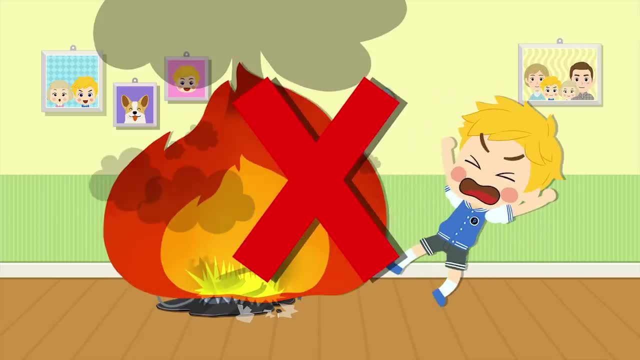 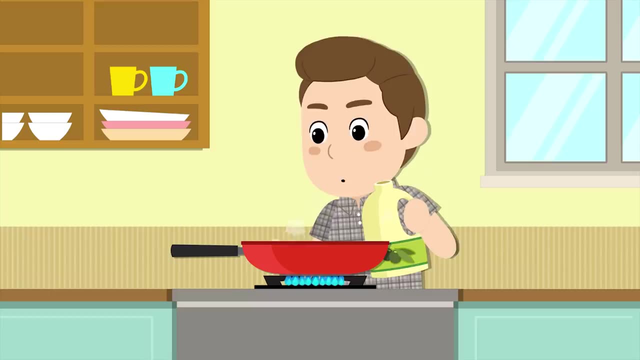 Ah, Fire from oil can't be put out with water. Putting water on burning oil can spread the oil and make it even more dangerous. Instead for grease fires, use a fire extinguisher or sand to put them out safely. These type of fires usually start when we're cooking. 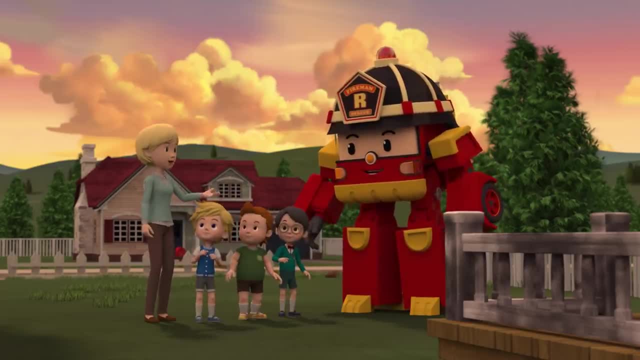 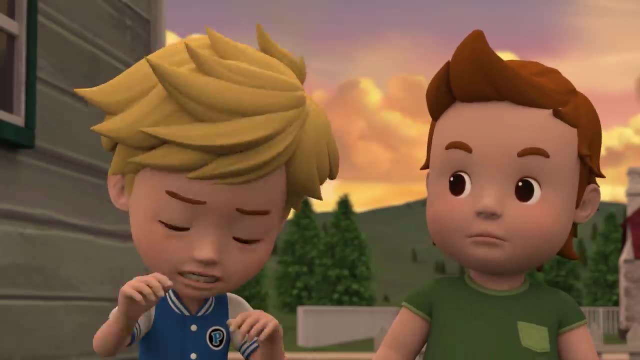 or using indoor heaters. so always keep an eye out. Uh, Thank you, Roy. Thanks Roy, We'll be careful. Aww, We put so much work into that clubhouse. I lost my porn-in-friend-o, My ham radio too. 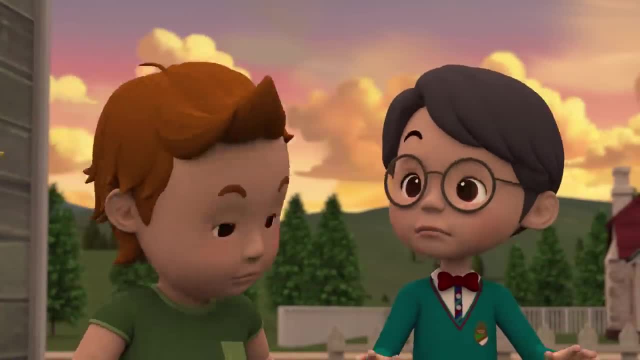 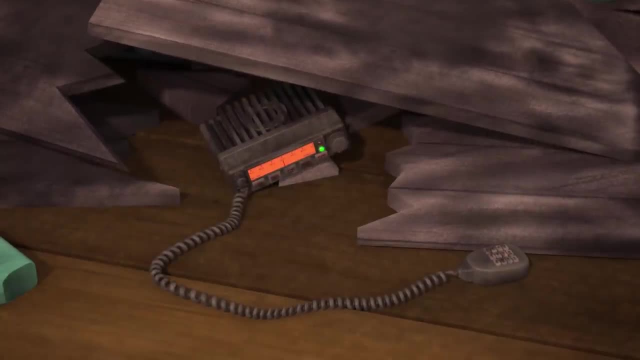 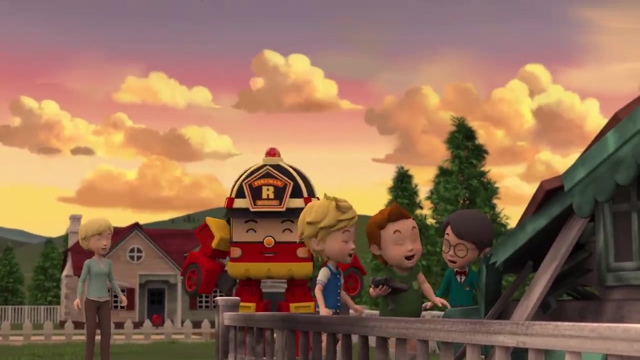 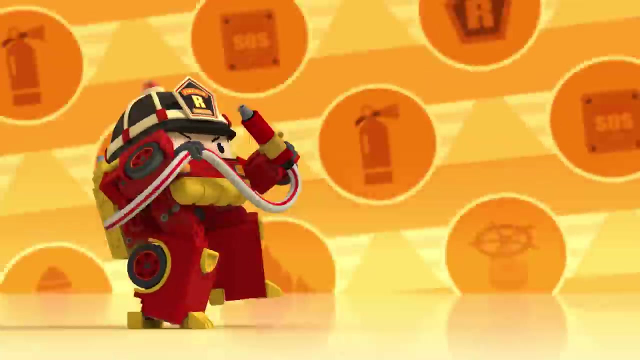 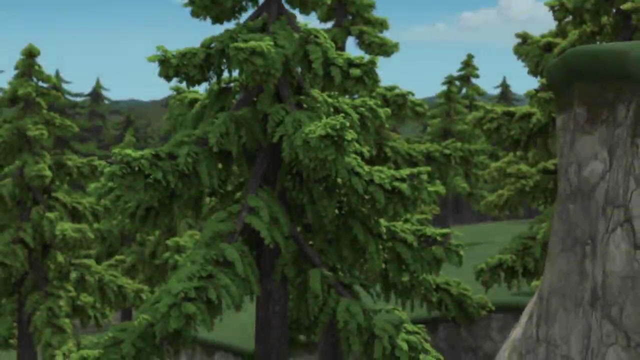 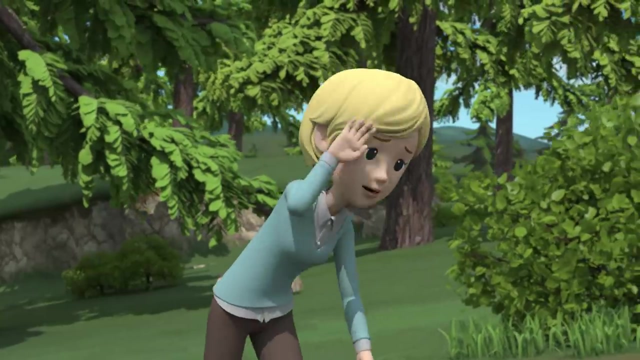 Huh, Whoa, Could it? No way. Wow, That's definitely aliens. We've totally made contact, Alright, Yay, A Fire in the Forest. Hey Dad, Are we almost there? Just a bit more. You said that an hour ago. 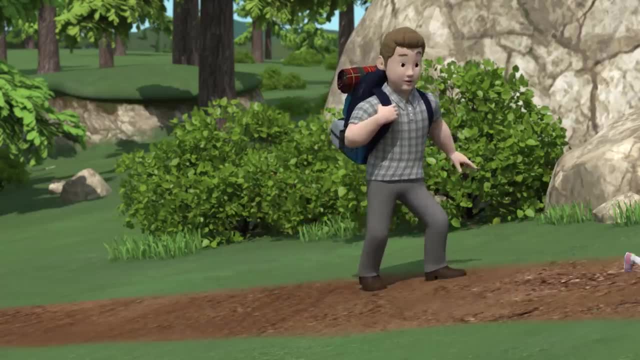 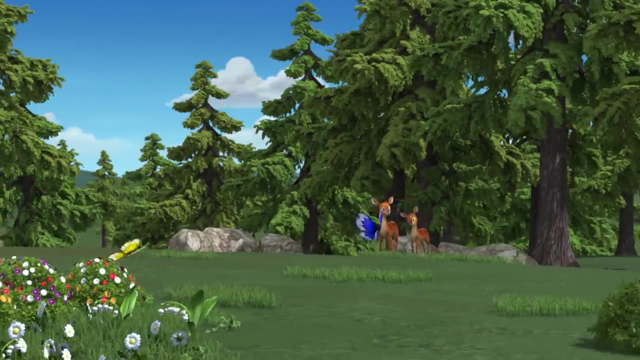 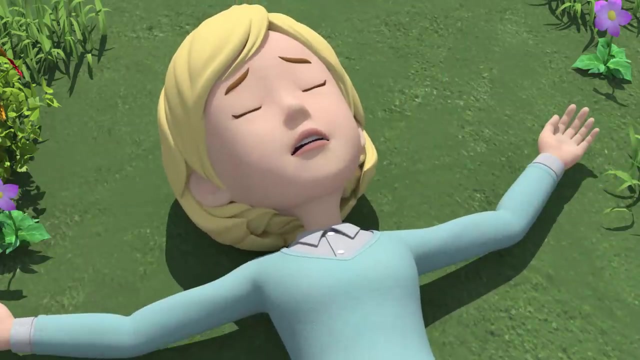 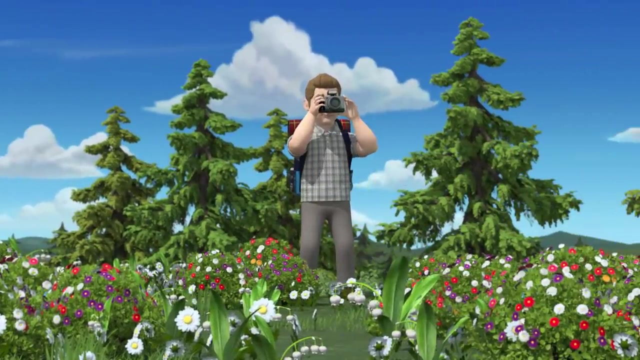 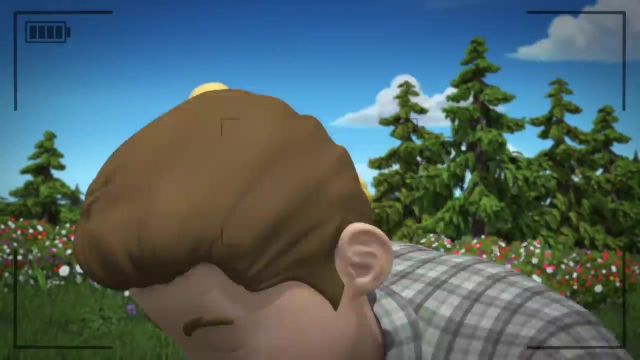 Dad, There was a deer over there Where Whoa So cool. Awesome, I'm done, Mom, Huh, Check it out. Uh, No, That's okay. Ahhh, Shh, Hey Say cheese. 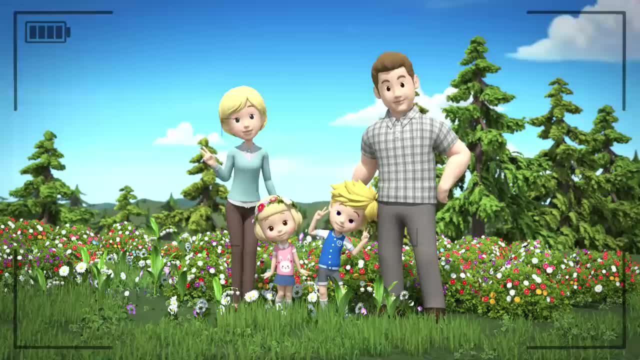 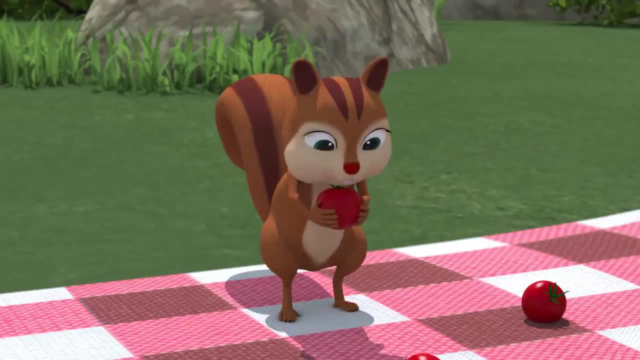 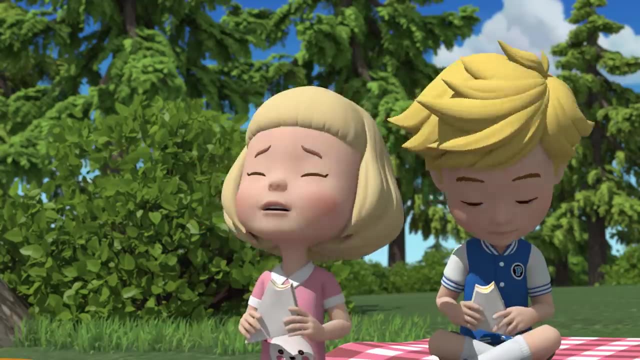 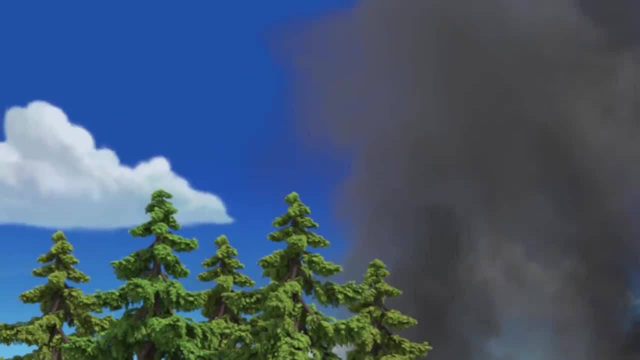 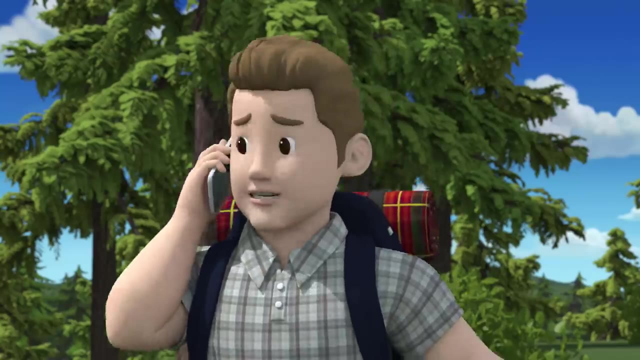 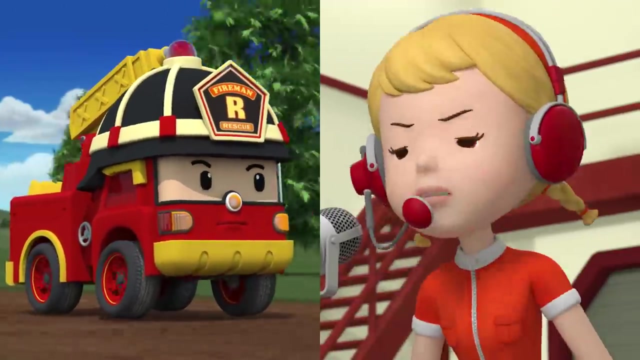 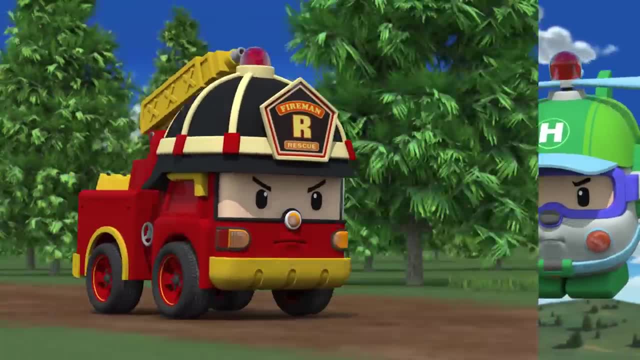 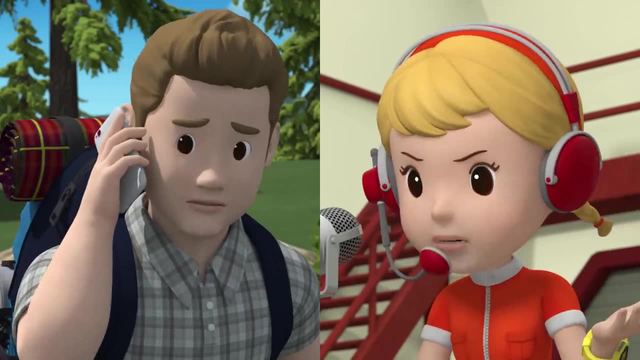 Oof, oh, oh, God damn. So another until we get a baby. Come on The sun. What are you saying? Oh, our baby, Super sharp, Wow. I had an experience. I had to do my homework. 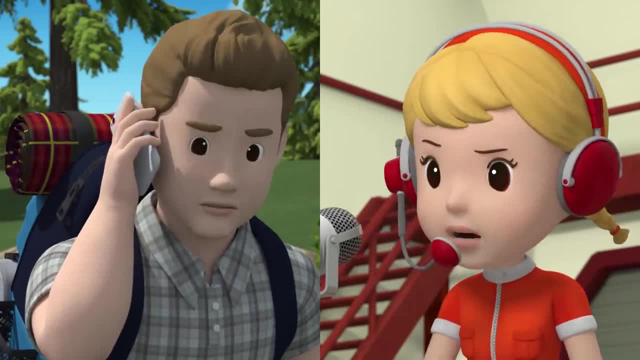 I got so much ugly stuff for Easter hat and disgrace hat stuff yesterday. There should be more lights on the roof. Oh, We are so close. Try to get upwind of it if you can. Thanks Jin, Now which way does the wind go? 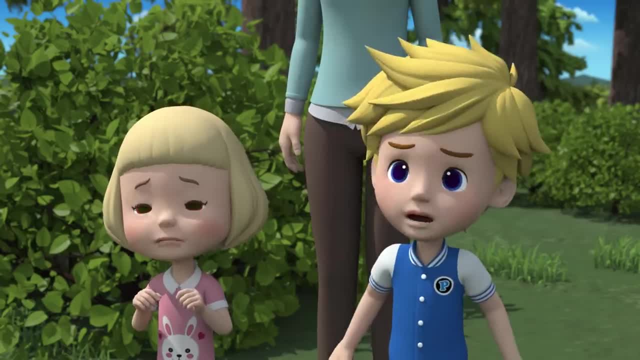 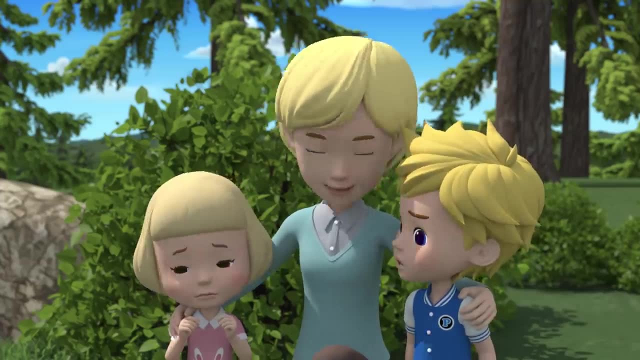 Which way is it blowing? Uh, But Dad, what are we supposed to do? Are we in super huge danger? Don't worry guys, Dad will lead us to safety and we'll all be fine, Right, honey, Uh? 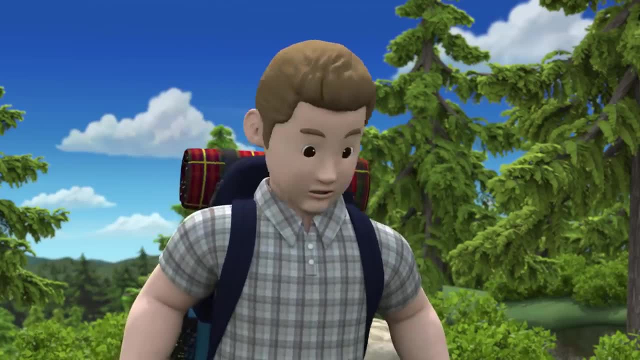 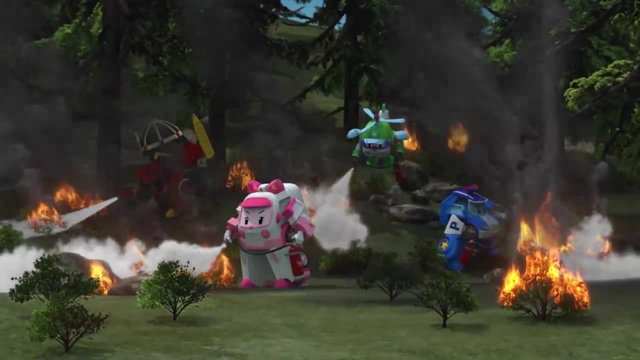 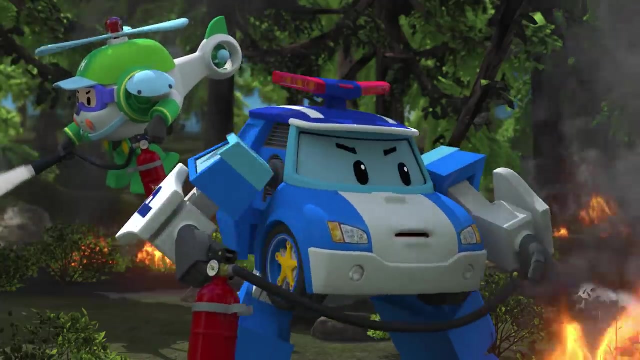 That's right, We're fine, Just trust your pop. Uh, Hmm, Uh, This way, Let's go. Uh-huh, Uh-huh. This wind is making it hard to stop the fire. We got this Just a little more. 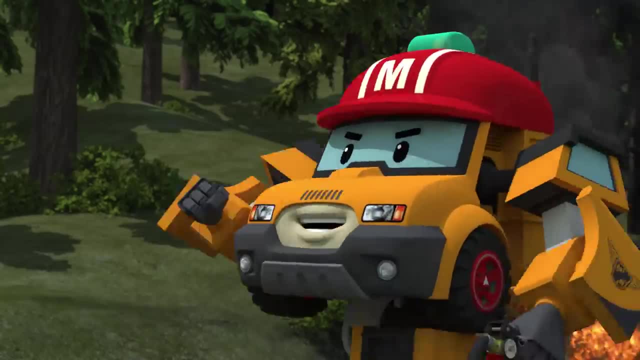 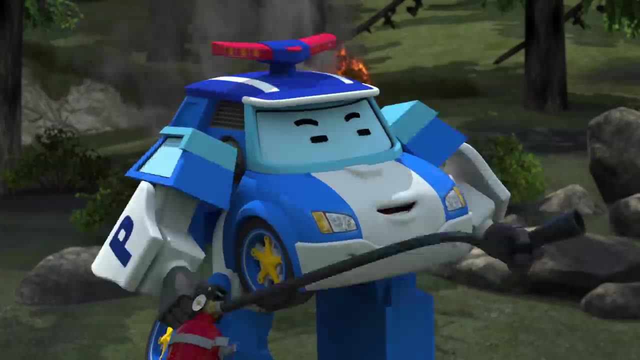 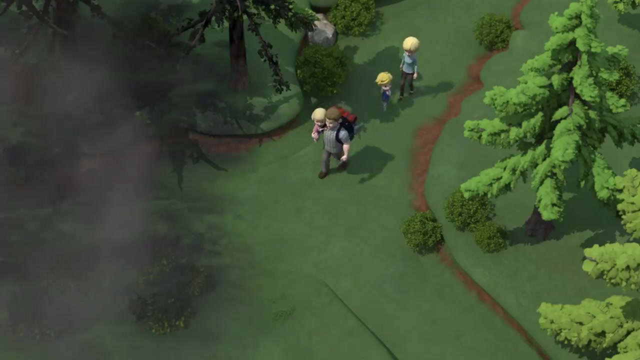 Hey Huh, Mark Bucky, Thought we might give you guys a hand. Luckily we got four Awesome. Hey, Heli, look for Peter's family from above On it. Uh Uh Huh, Oh no. 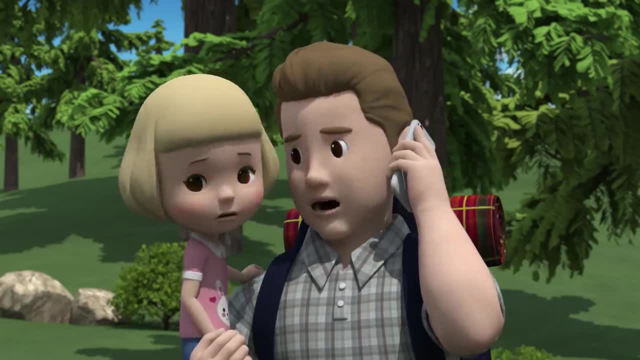 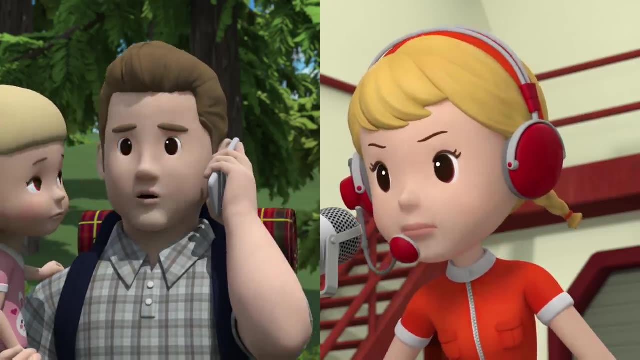 There are two roads, Jin. one road's been burned by the fire and one looks clear. Which one do we take Right now? take the road that looks like it's been burned. Are you sure that's where we should go? If it looks burnt now, the fire has already passed through. 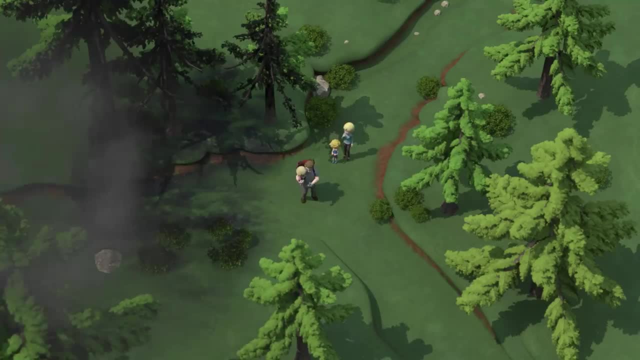 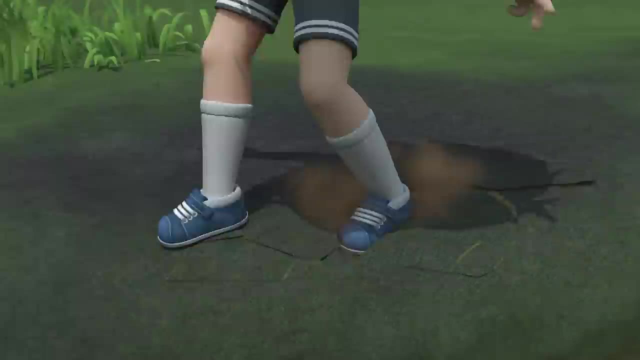 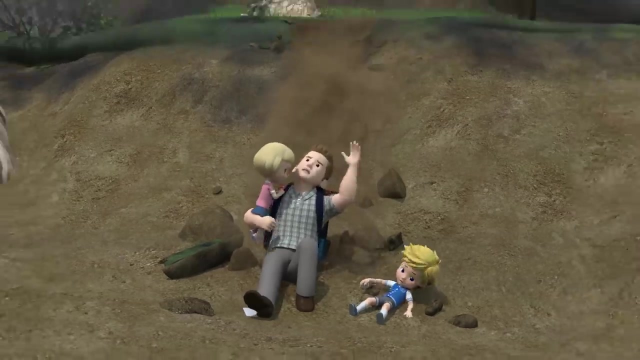 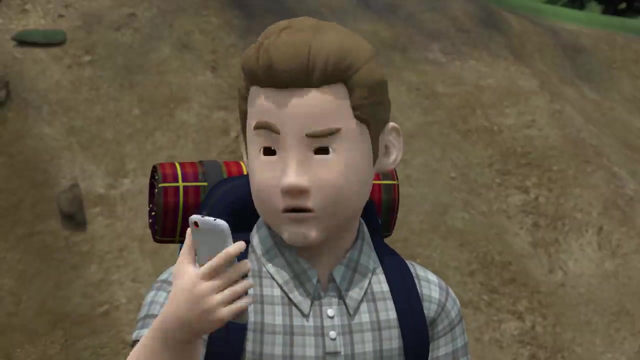 I promise it'll be safer. I understand All right this way, Peter. Oh no Kids. Oh, Are you okay? Yes, we're all good. Jin Jin, Huh, My phone broke. Oh no Dad. 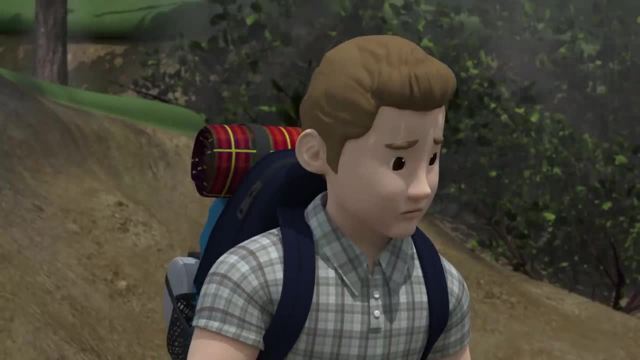 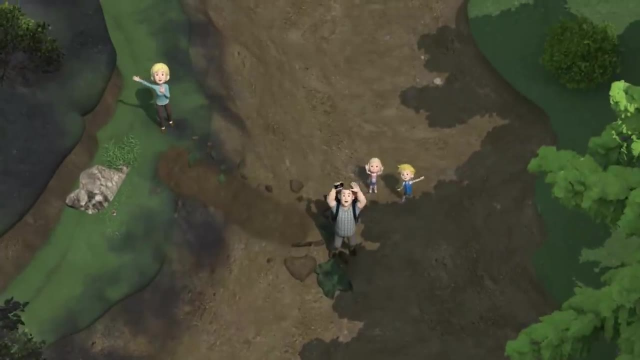 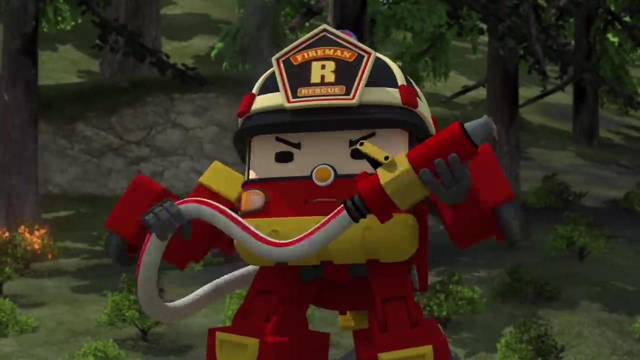 What do we do now? Ah, Peter Lucy, Oh, hear that Heli Huh Down here. Ah there, you are Right, I found them Great. Take them to a safe place. Let's finish this up. 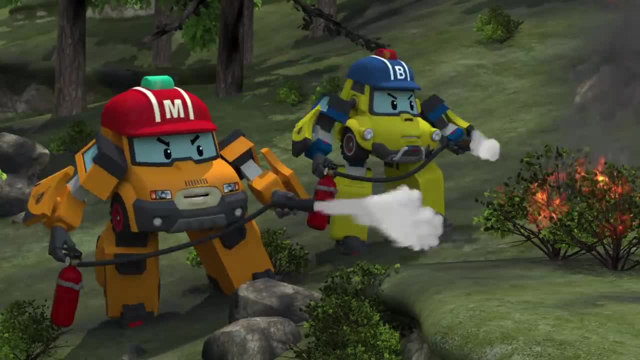 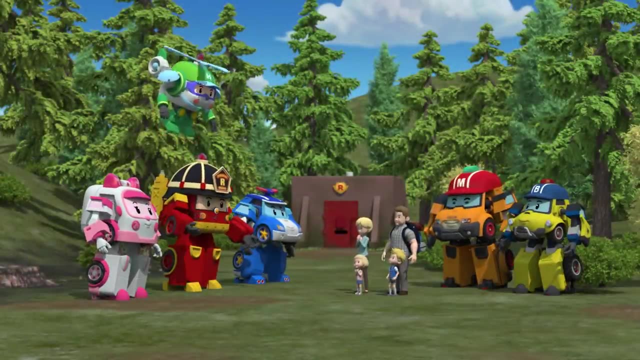 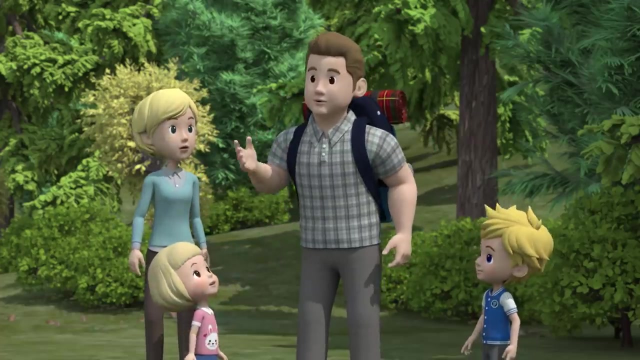 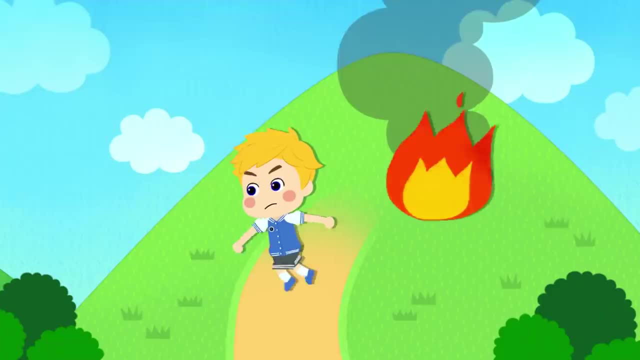 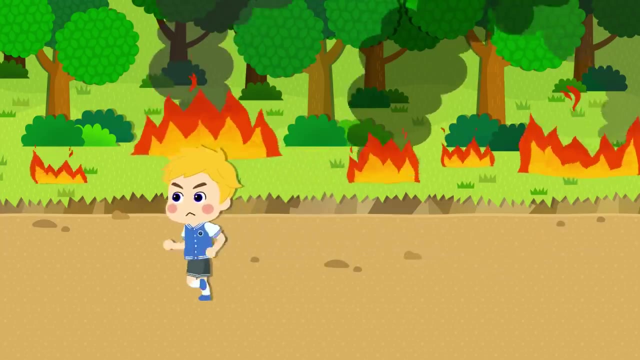 Aw Well, don't thank me. We're going to make the forest fire get as quiet as you can. Get to a lower area, not a higher one. Fire will spread with the wind, so go in the opposite direction of the wind. 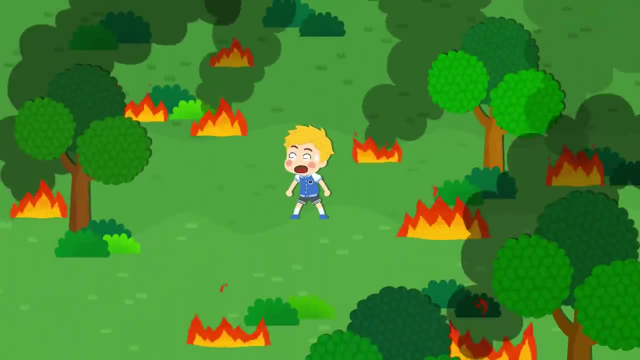 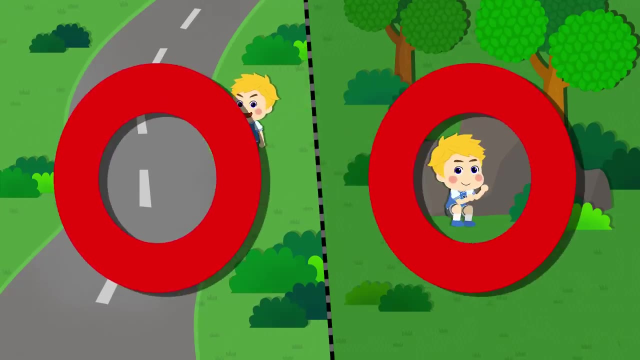 If you find yourself in a forest fire, remember not to panic. Go to a place that looks already burned or with fewer trees. Open roads and rocky areas work too, But mostly always remember to stay as calm as you can. That way you can be rescued. 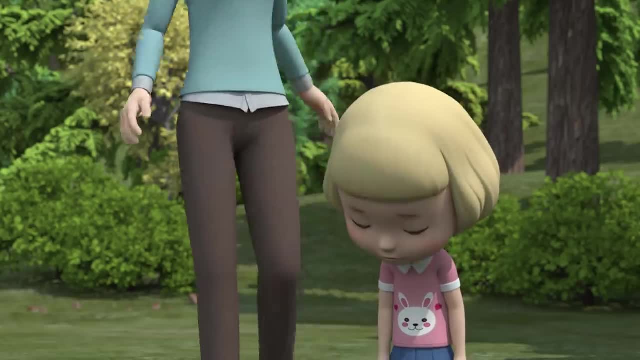 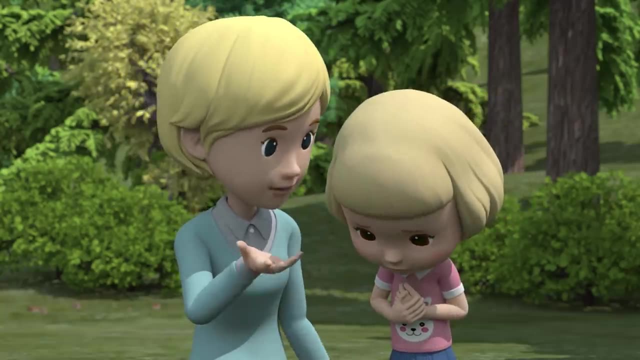 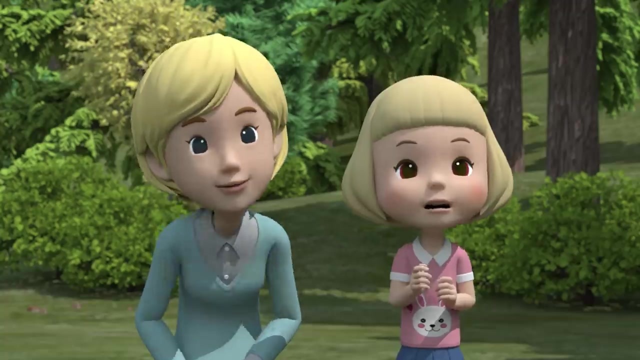 We got it. Ah, What's wrong? Oh, Mom. but what about the squirrel? Don't worry, I'm sure he got away safe and sound. Whoa, Over there, The squirrels did get away safe, You see, Lucy. 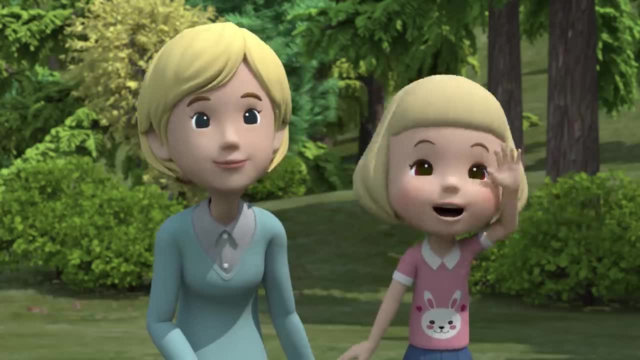 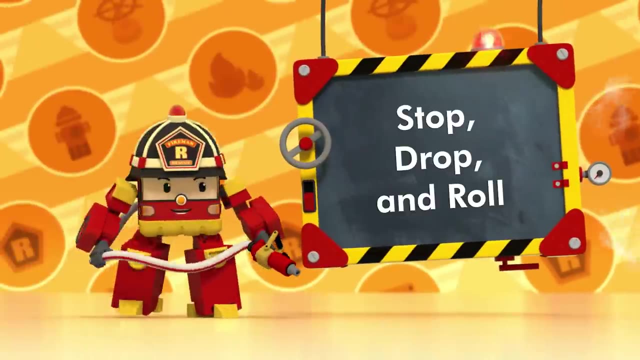 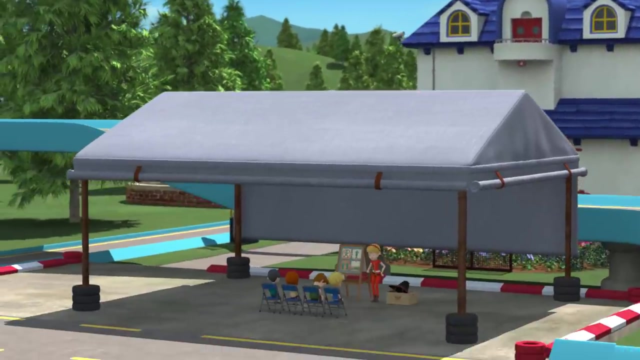 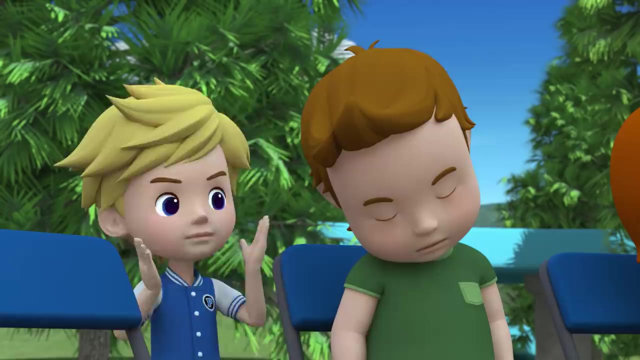 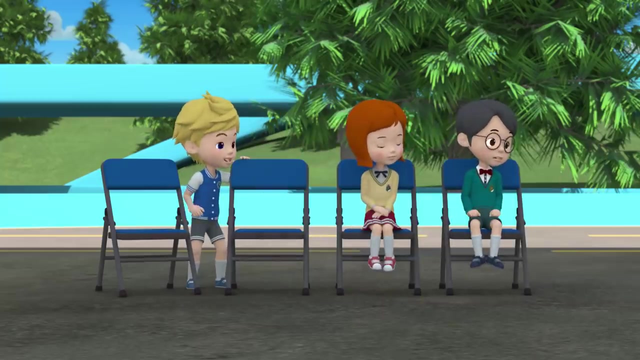 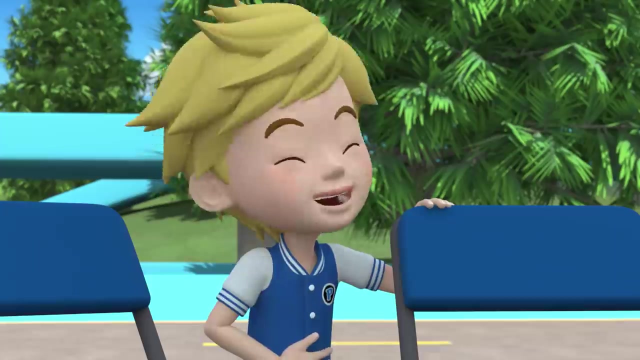 Yay, Bye-bye, squirrel family, You know what to do if your clothes catch on fire, right? Yes, Johnny, wake up Your shirt's on fire. Huh, Put it out. Put it out, Peter Johnny. 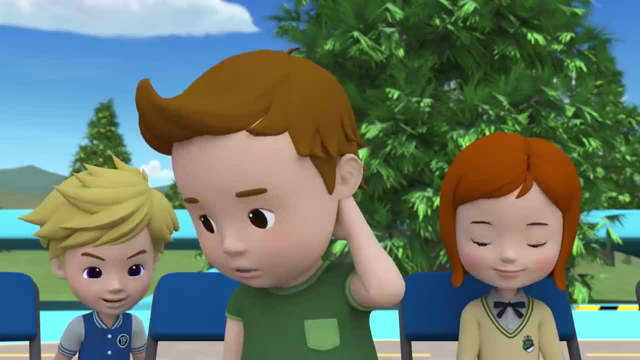 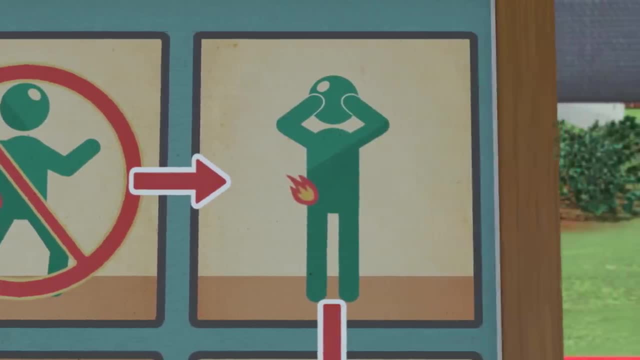 Huh, What if your clothes catch on fire? Um Well, I Johnny up there First, stop, Don't run. Then cover your mouth and nose and drop to the floor. Last roll back and forth, Got it? 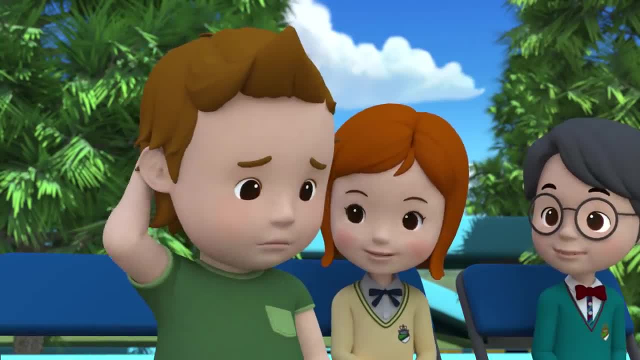 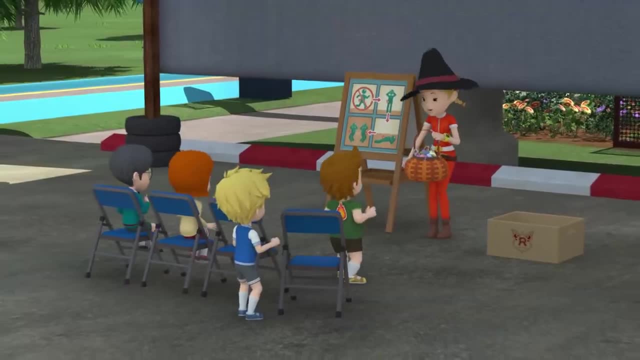 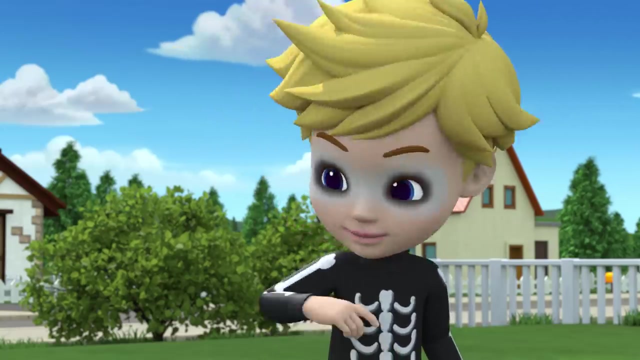 Don't forget. okay, I won't forget. Huh, All right, everyone. Whoa, That's it for today. Happy Halloween, All right, Thank you, Gin. Wow, Johnny, You make a great vampire. Cool idea. 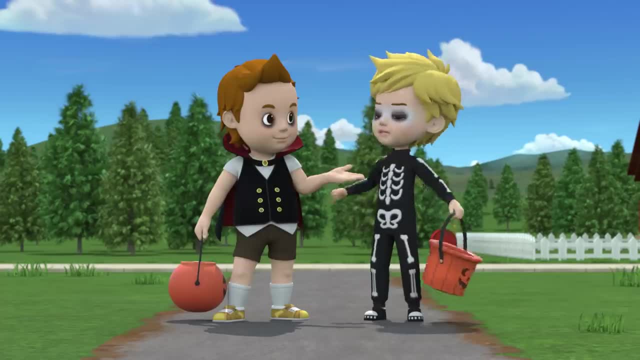 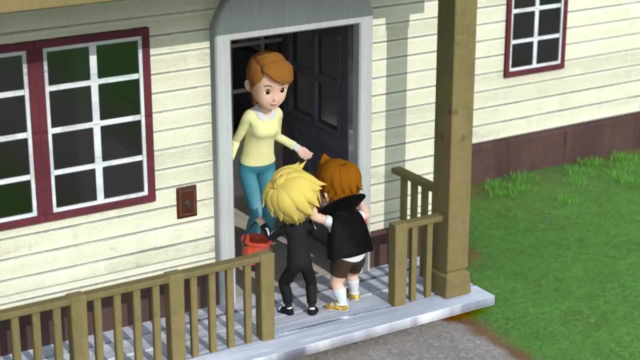 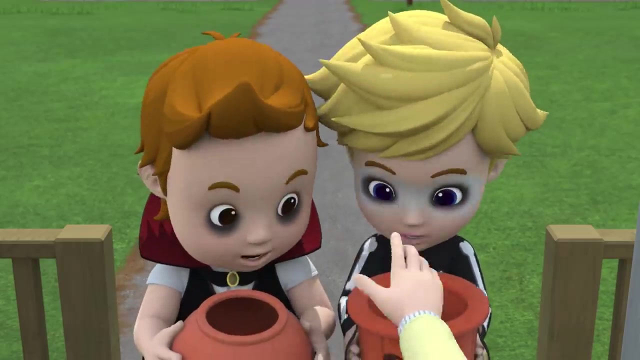 And your skeleton's awesome. Then let's get to it. All right, Trick or treat. Oh, my Peter and Johnny, You guys look really great. Here you go, you two. Happy Halloween. Oh Wow, Thanks a lot. 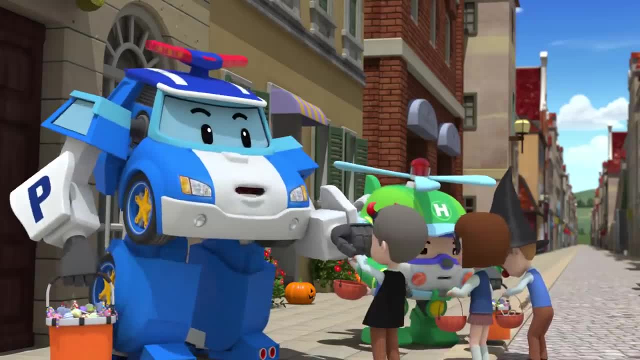 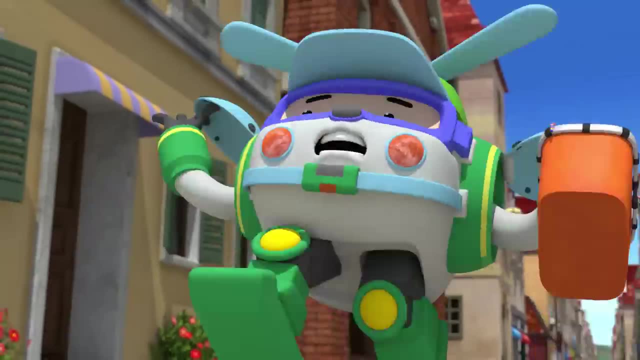 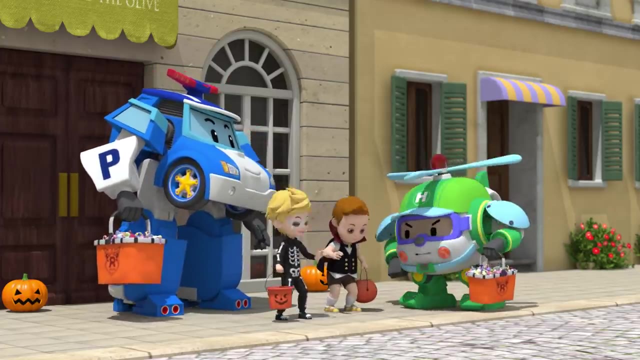 Trick or treat. Happy Halloween. Wow, Thanks, Thank you. Oh, Trick or treat. Hey, Hallie, it's me, Peter, That wasn't nice. You guys really scared me. Can we have some too? Happy Halloween, Pete and Johnny. 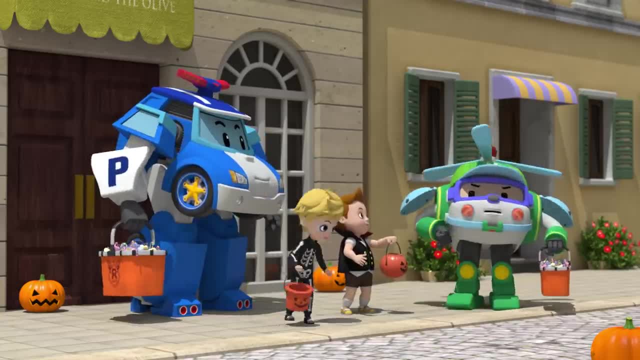 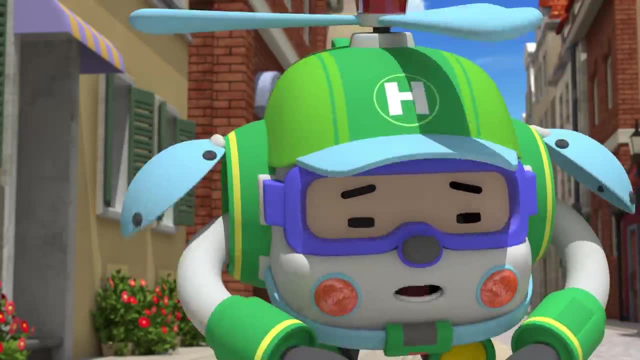 Ah, thanks, Polly, Hallie Hm. sorry, I just ran out. If there are no treats, then there's gonna be tricks. Ah, Oh, don't do that. Have some candy Trick or treat. Ah. 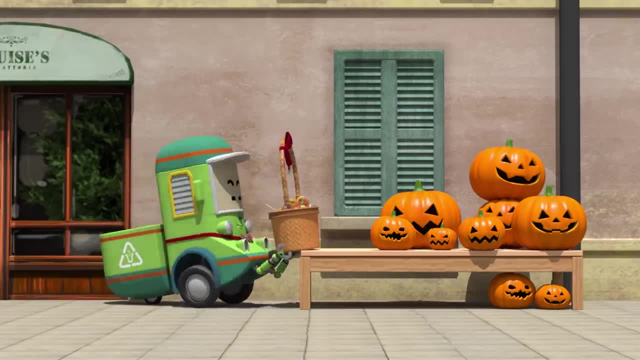 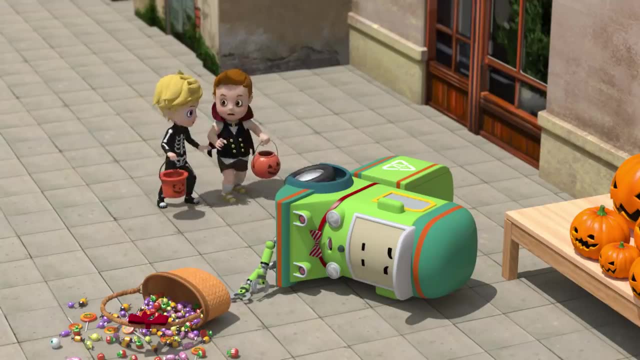 Oh Oh, Kleeney, Kleeney, Trick or treat. Wow, Those costumes are great. You choose trick or treat, You choose trick or treat. How funny are you guys. How about a treat? Oh, Oh, Oh. 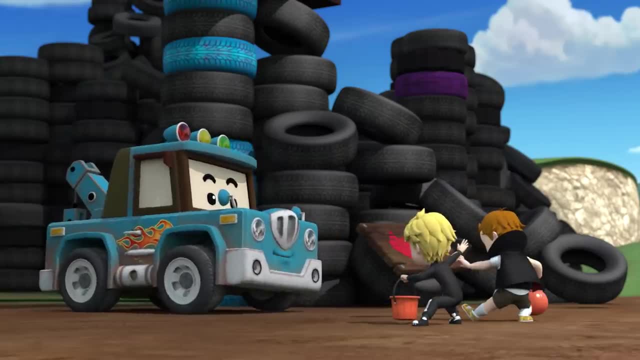 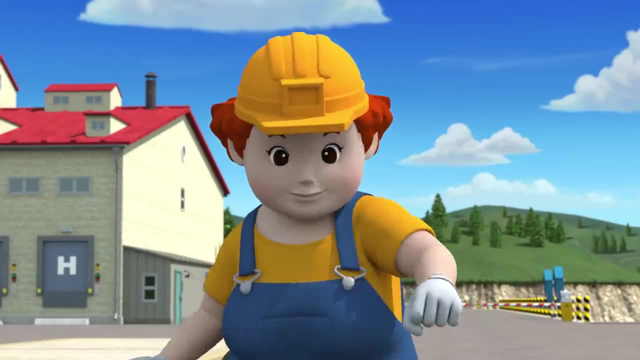 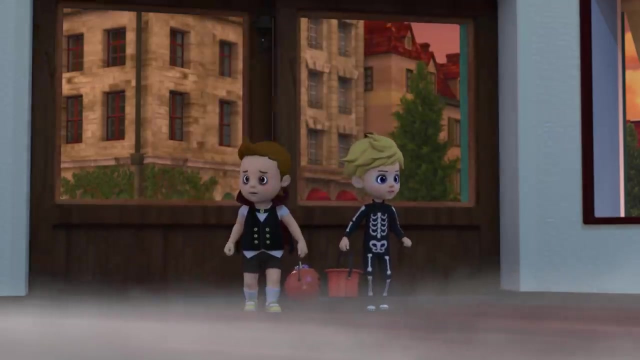 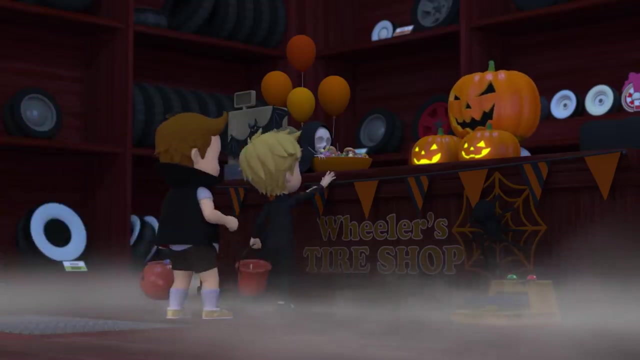 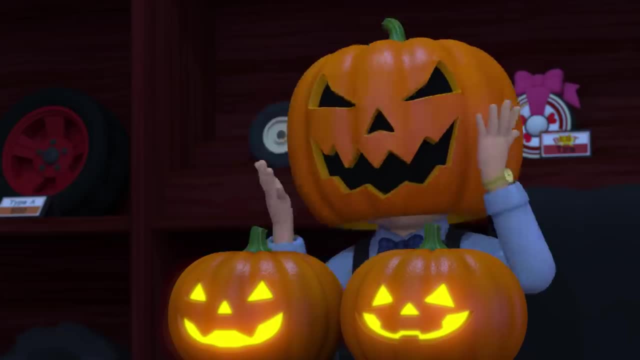 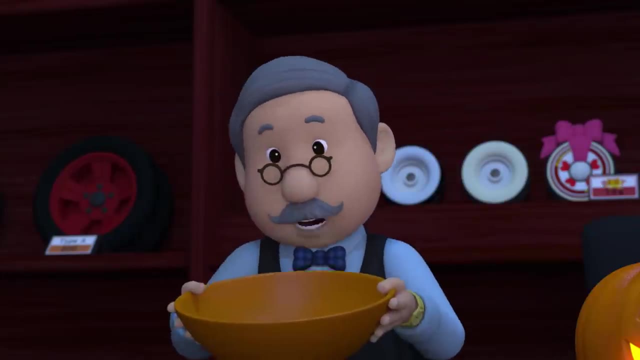 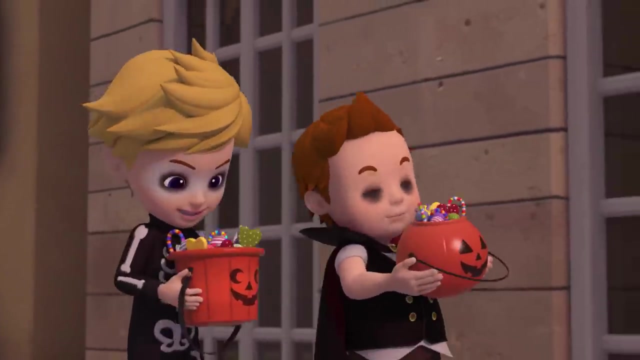 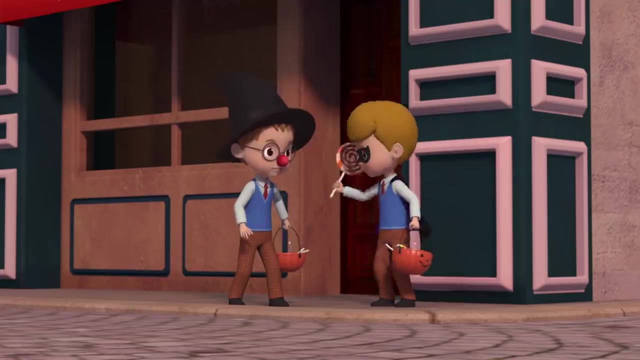 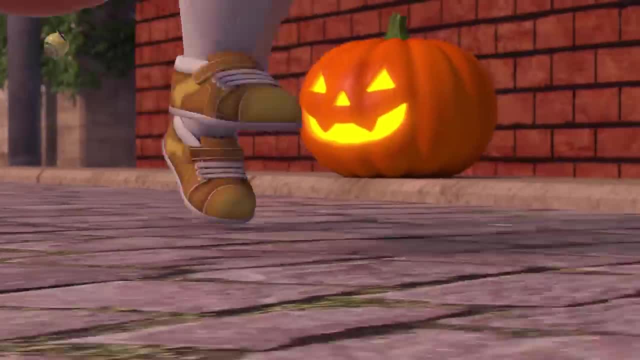 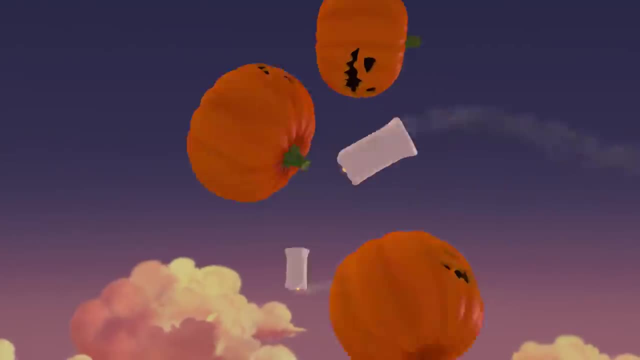 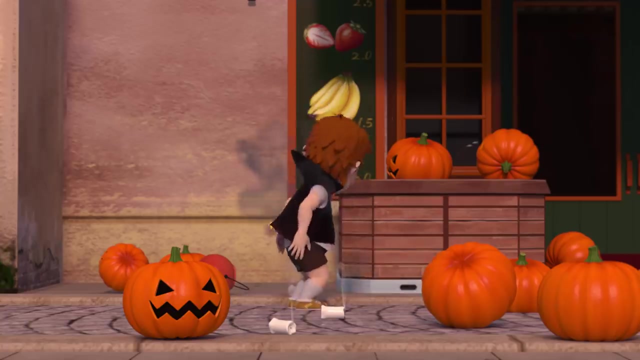 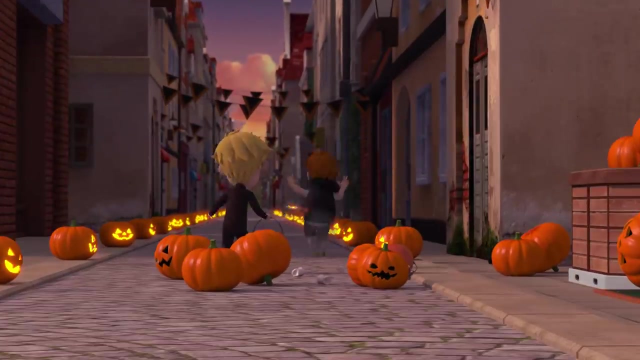 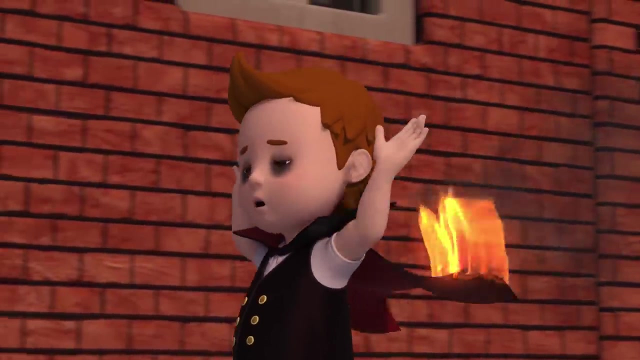 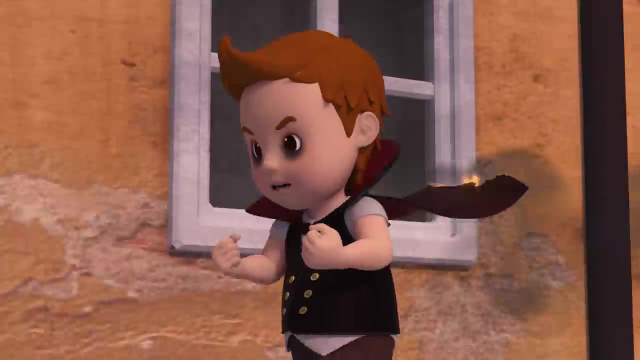 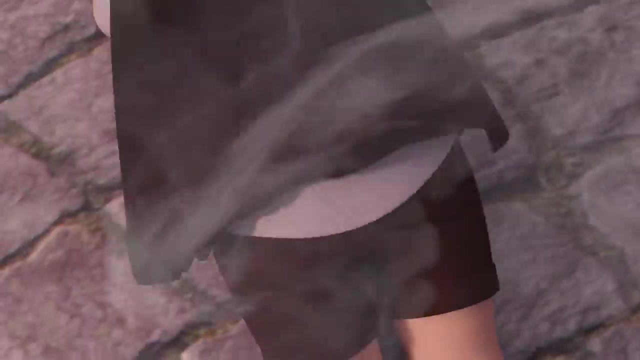 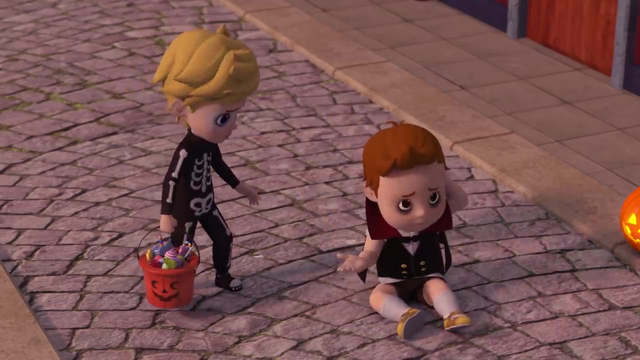 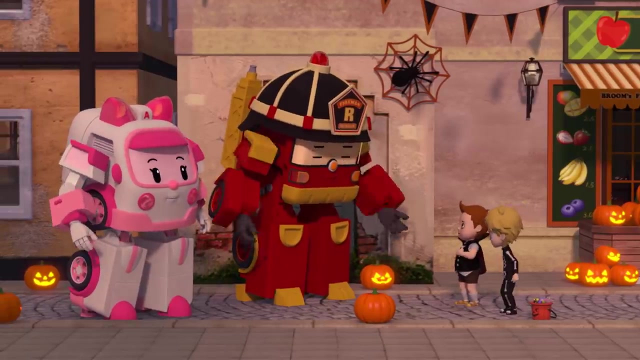 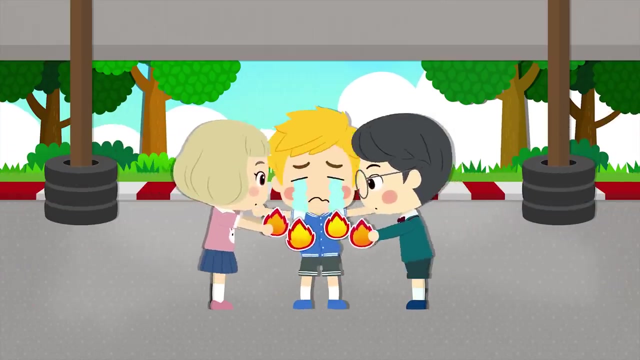 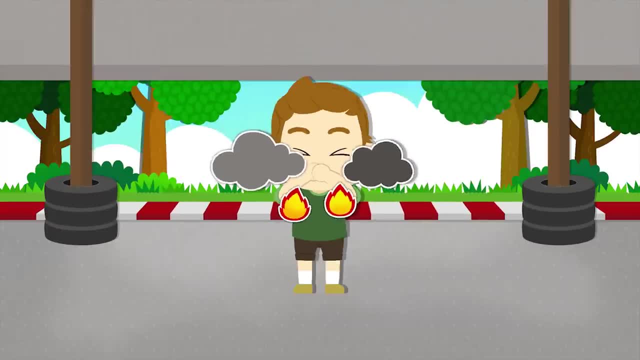 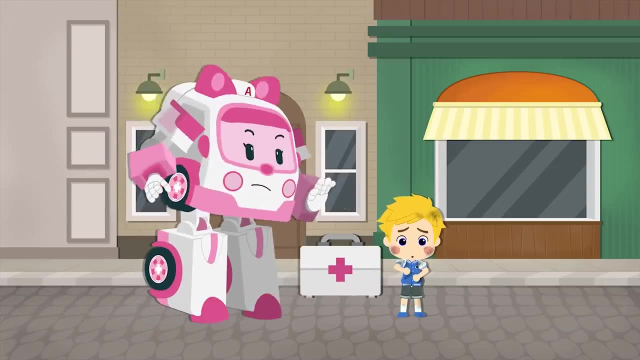 your nose and mouth to avoid inhaling smoke into your lungs. Then drop to the floor and roll to put out the flames. Burnt clothes may stick to your skin, so be careful when removing them. If that happens, ask a grown-up for help. 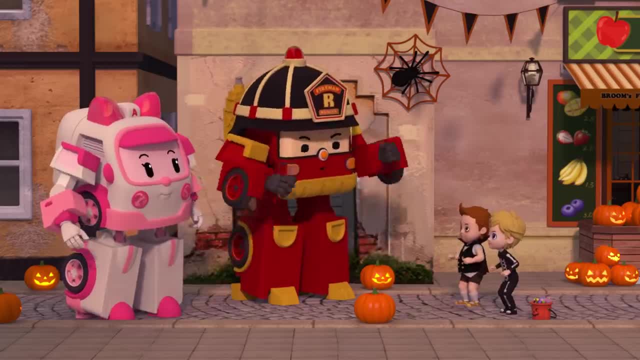 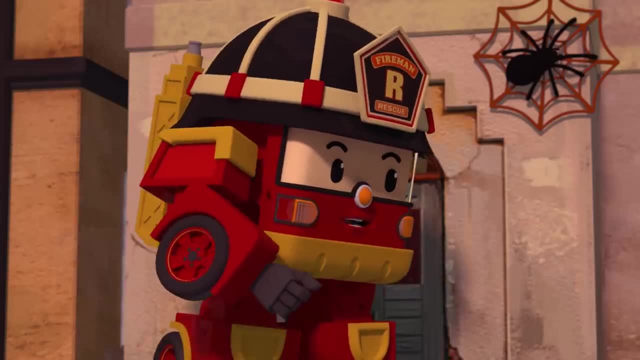 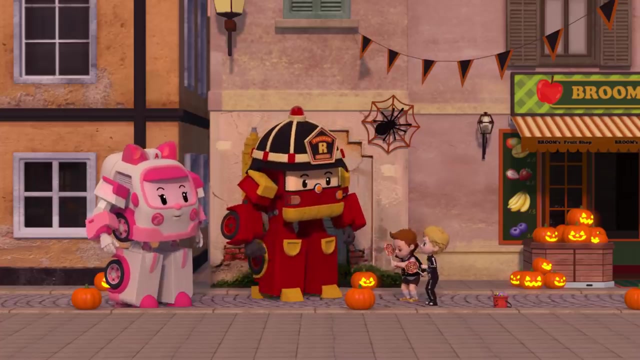 Alright, we got it. You think What happens when your clothes catch on fire. You stop and then you drop and roll. Good work Here. these are for you, for doing what you learned. Wow, They're massive. Thank you, Roy. 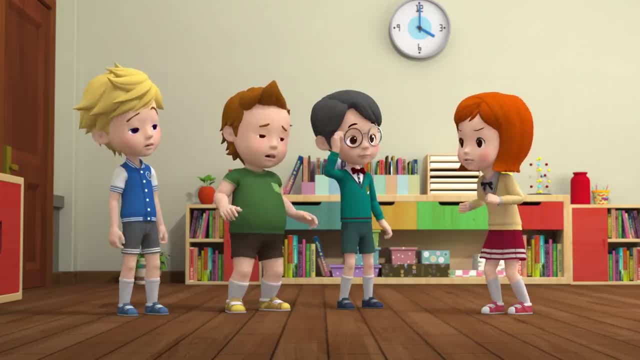 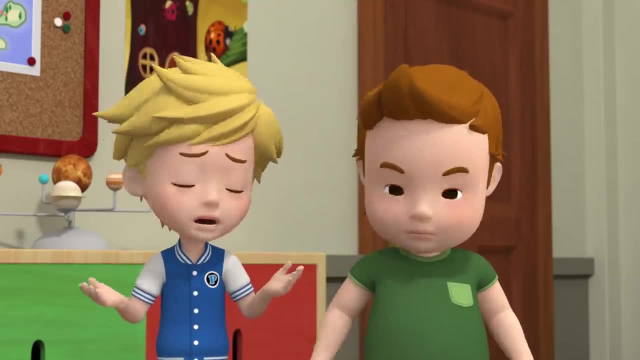 What For real? For real, I really can't dance. I feel so bad. We'll lose the dance contest because of me. So now what? I had no idea you couldn't dance. Don't feel bad about it, I'm happy to help. 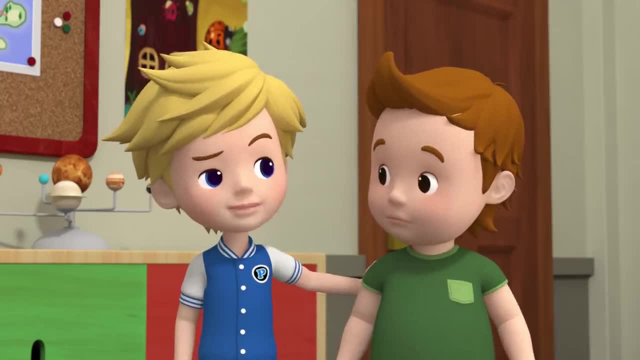 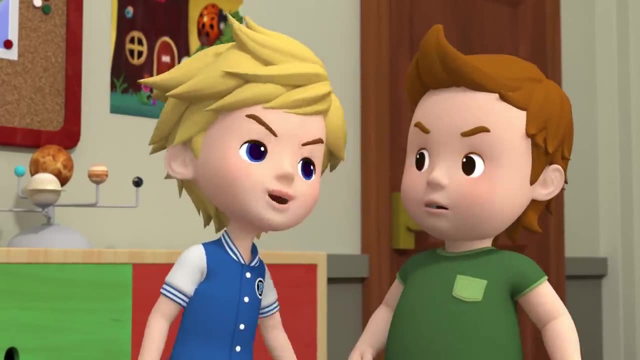 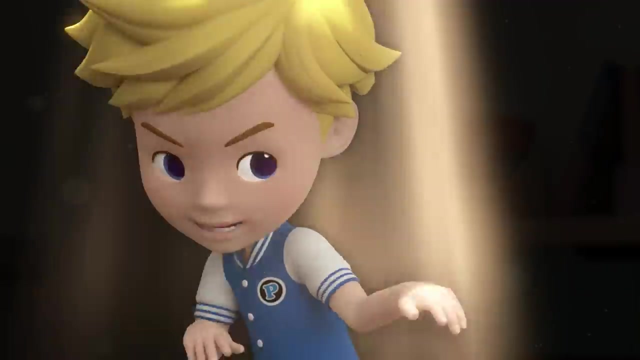 Come on, Johnny. I'm sure Cindy would rather be taught by the town's most legendary dance machine ever. What If you're the dance machine? then I'm the king of dance. Are you challenging me? Bring it on, Not bad, Johnny. 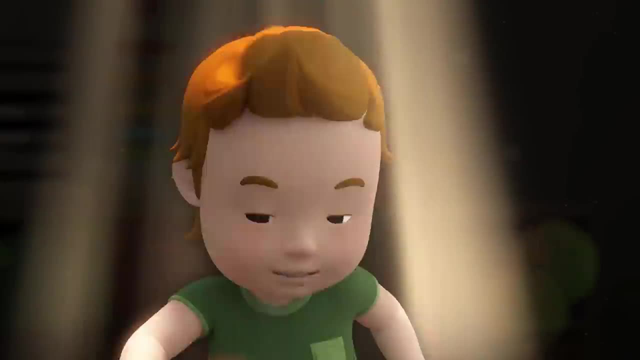 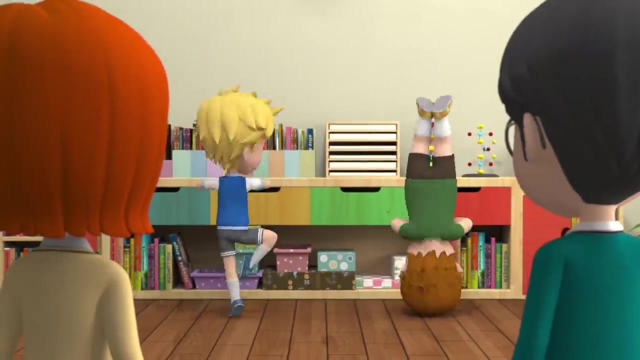 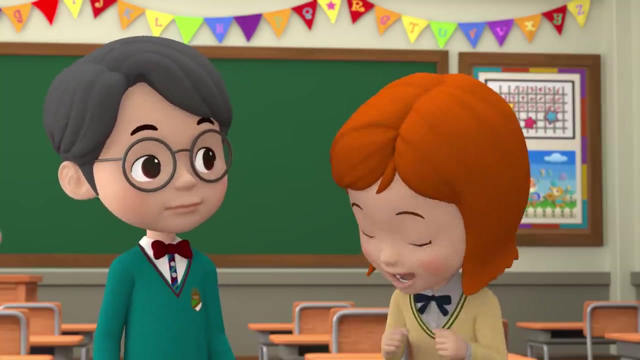 I know you're not bad either. Hey, check this movie out. Watch this. You know I couldn't dance either, but then these two totally helped me get better at it. They did, So we might not come in last place. 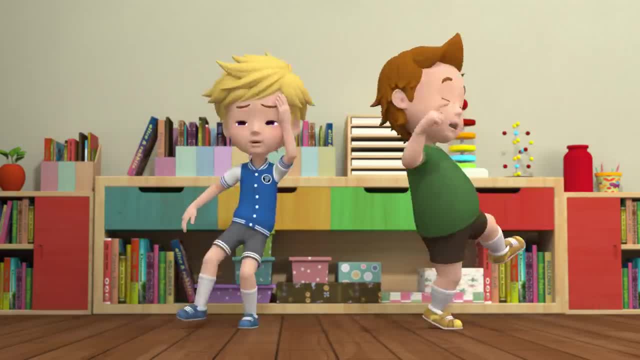 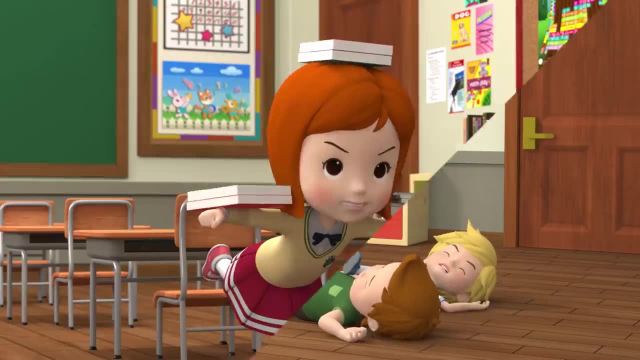 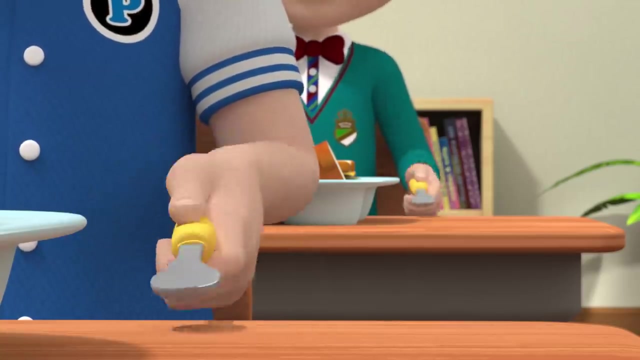 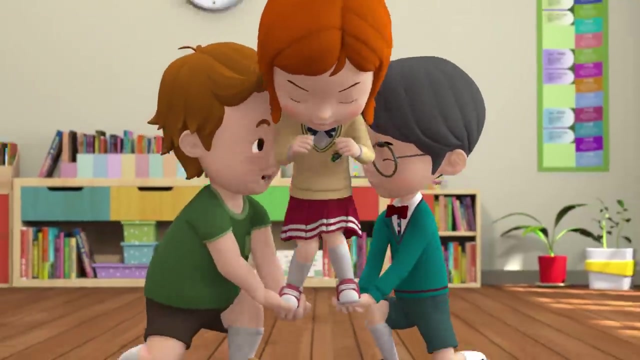 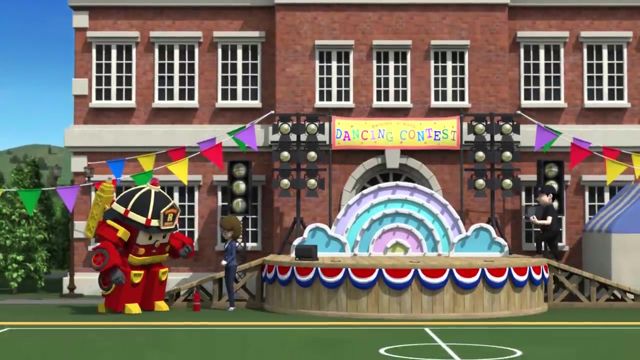 Last place? No way We're coming in first In first place. Yes, Awesome job, We did it. Let's put one here too. It's important to have enough fire extinguishers and to know where they are in case you need them. 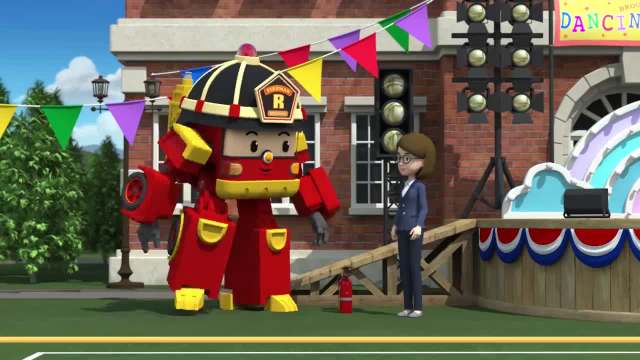 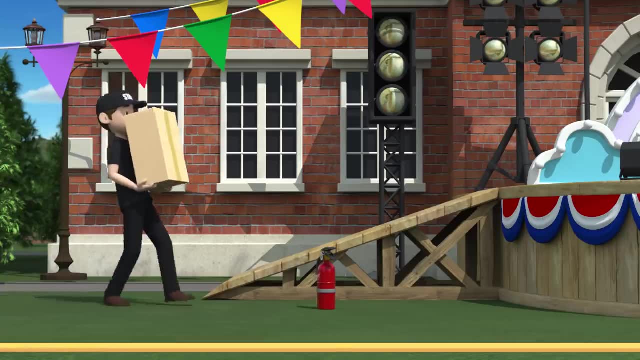 Alright, Thanks for taking care of it, Roy. Of course I'm sure it'll be an exciting contest. The kids have been working so hard You should come. Oh, I'd love to. Ugh, I can hardly see where I'm. 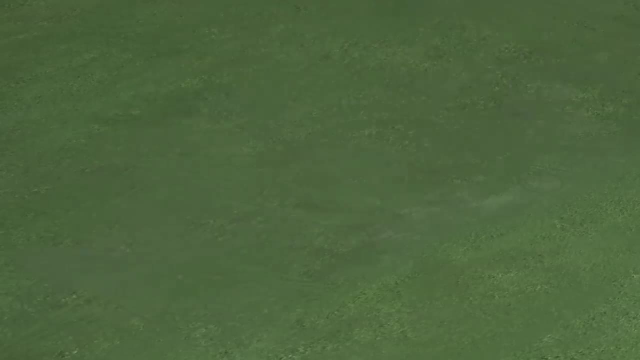 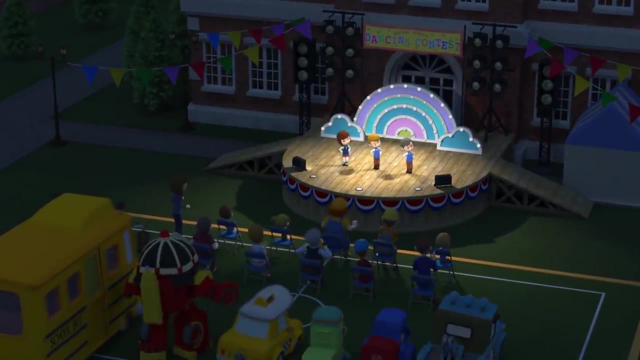 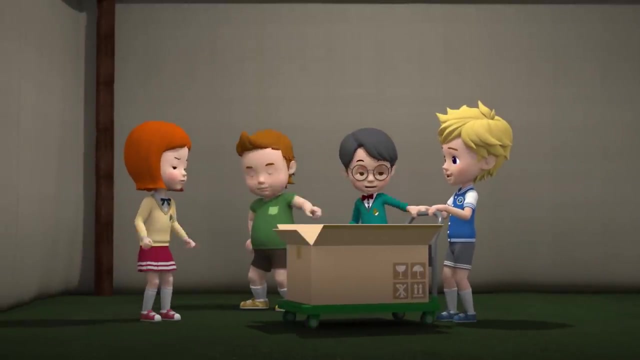 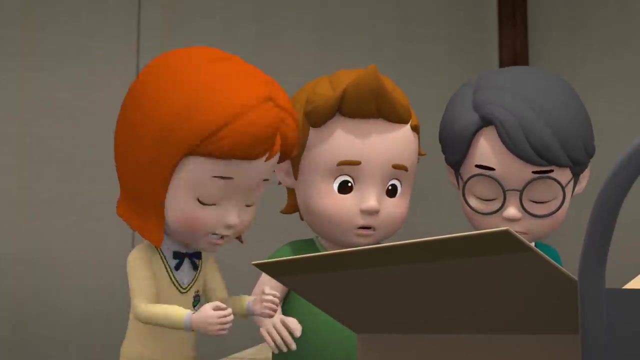 This is definitely not a good place for this. I think I might be sick. Hey you guys, Peter, where are the next ones to go? Listen, I got us a secret weapon. Check it out. Secret weapon, Woo-hoo. 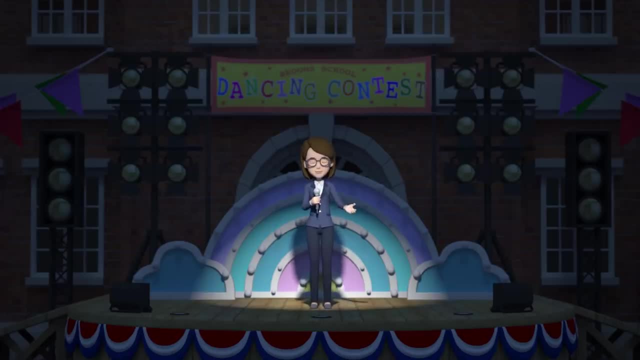 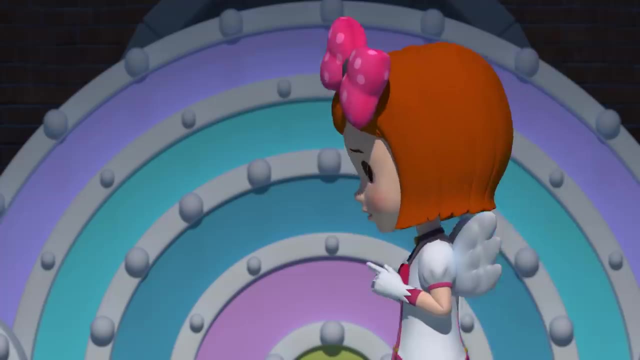 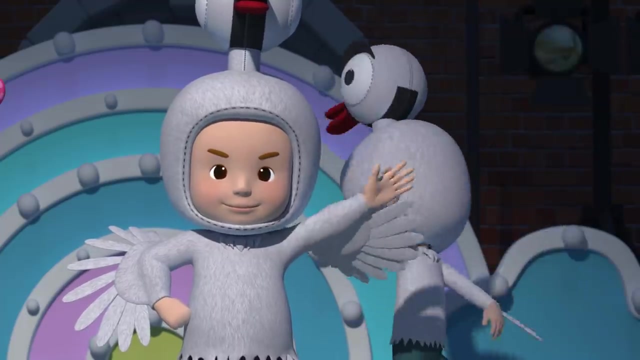 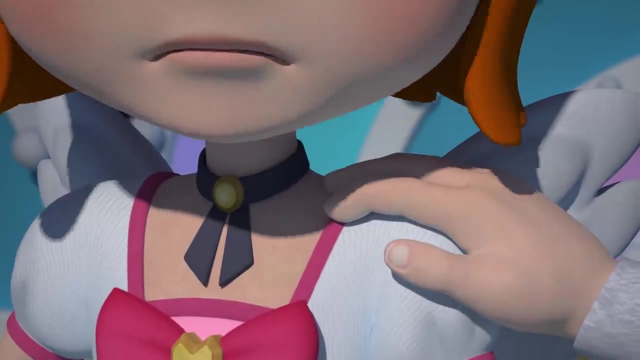 What is that? And now we have our next team. Please welcome Cindy and the Broomstown Boys. No way, How humiliating. Come on, Cindy, With these on, we gotta win. Hey, you'll be fine, Leave it to us. 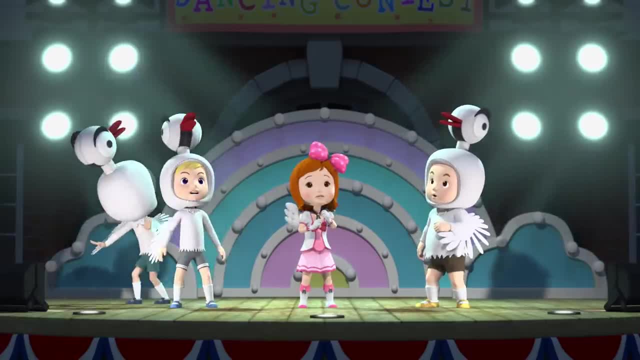 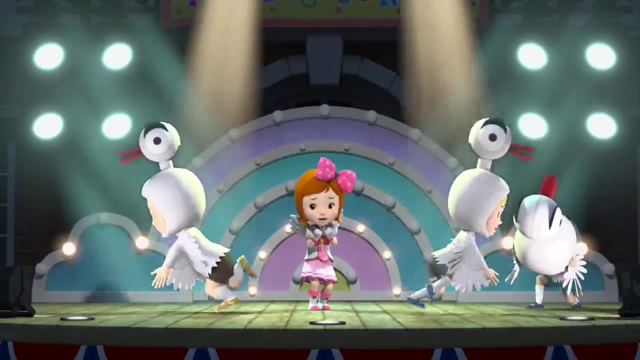 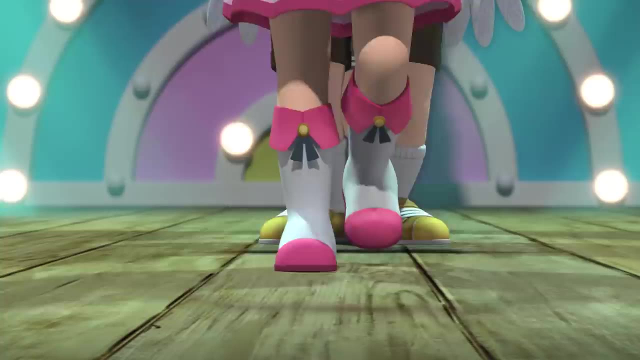 That is so not comforting. What's happening, Roy? I can't see a thing, But scary things can happen And where and when they do, Roy will be there for you. This is awful: When we need him, he's always around. 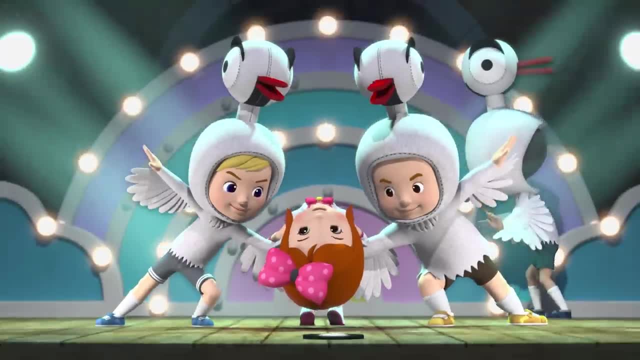 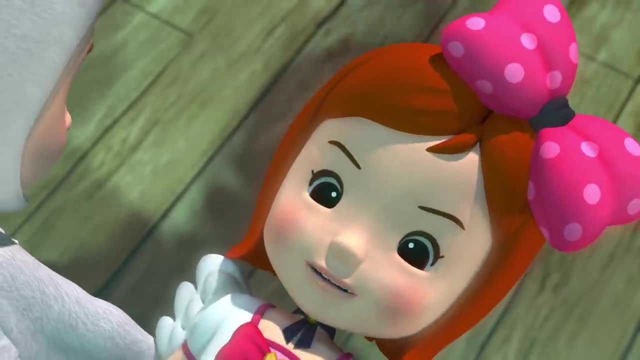 He keeps our hearts safe and sound When the flames endanger the air. Now, do you trust us? I know that there's no need to fear. Are you ready? Cindy Roy will appear. Yes, let's do this. We are learning fire safety. 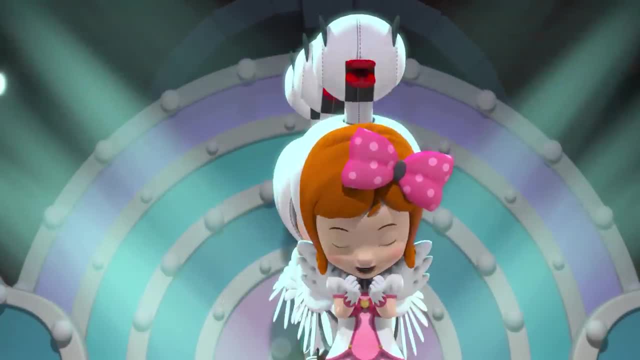 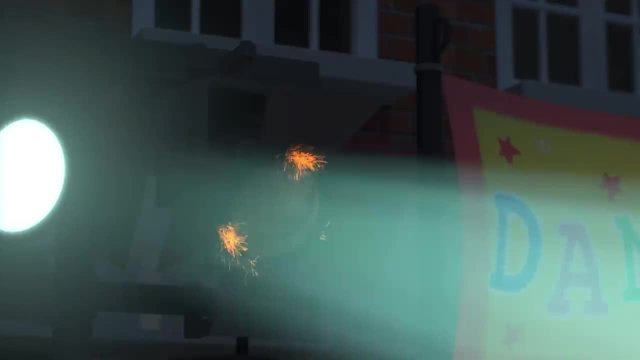 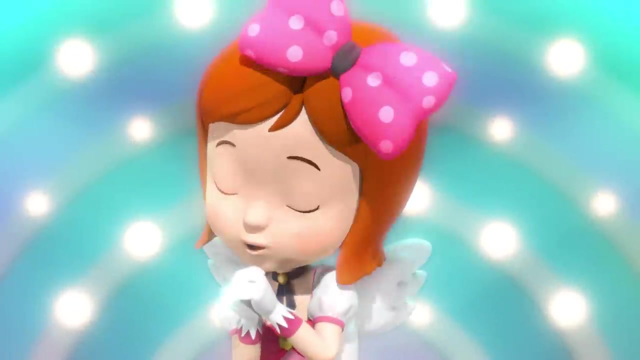 From a super awesome teacher. He's strong and he's courageous And he'll teach us all to be safer. Together we are learning What to do if something's burning. We are learning fire safety. Roy wants us to be safe as we can be. The fire is burning. 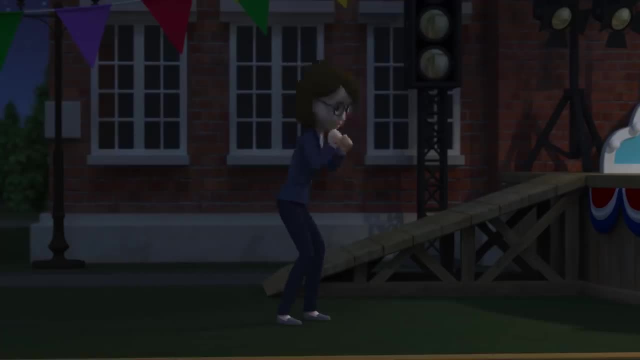 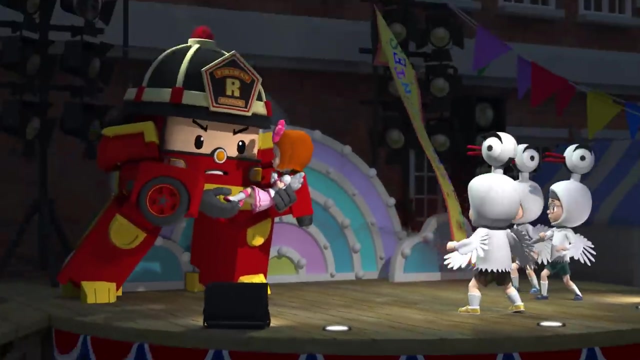 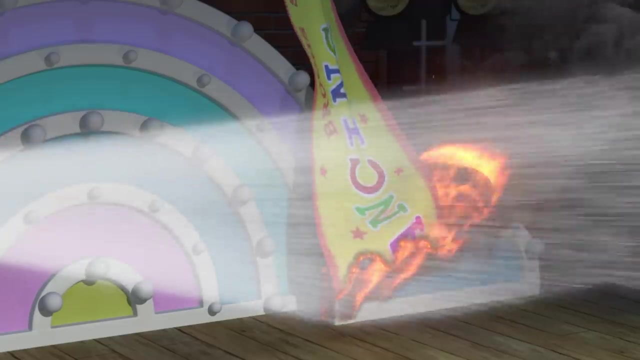 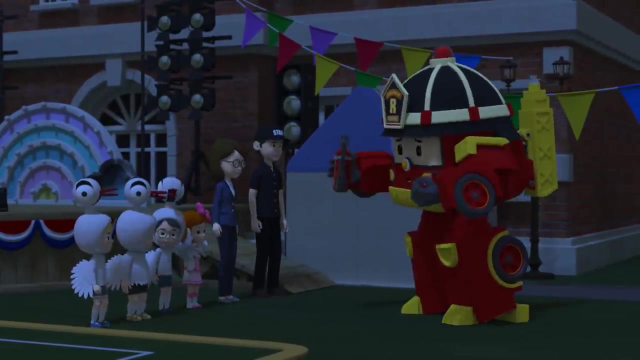 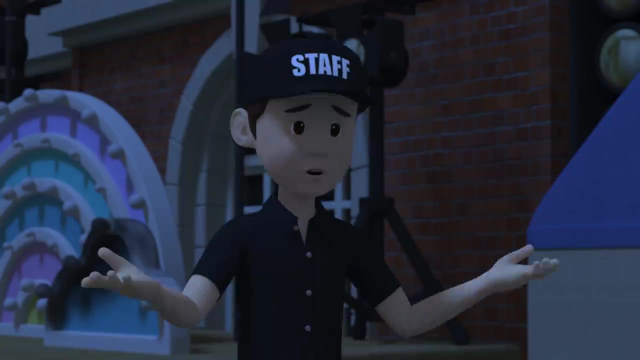 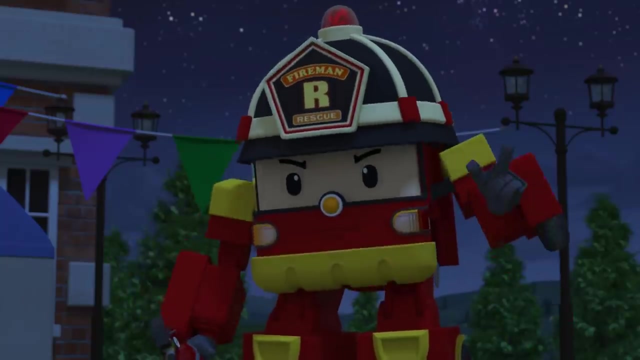 I'm really sorry, Roy, To think I could have caused a much bigger accident. I had no idea we even had one of those I know. Then everyone listen up- Fire extinguishers can be just as effective as a fire hose. 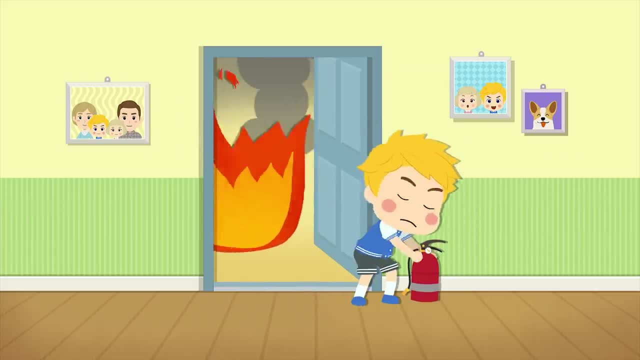 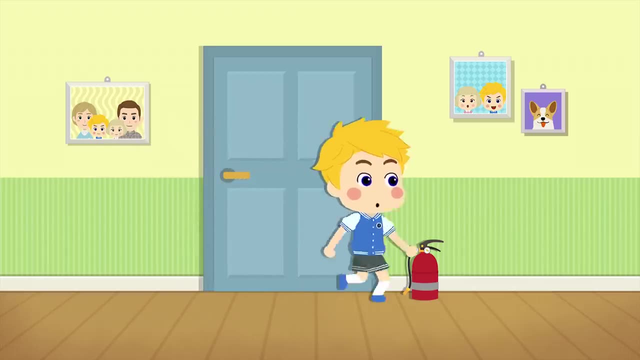 Make sure to keep fire extinguishers in sight and within reach. Always keep them out of direct sunlight and humidity. Check your extinguisher often for broken parts or corrosion. Give it a good shake once a month so the chemicals don't harden. 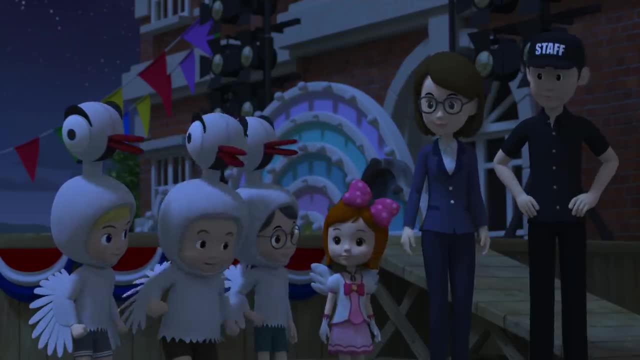 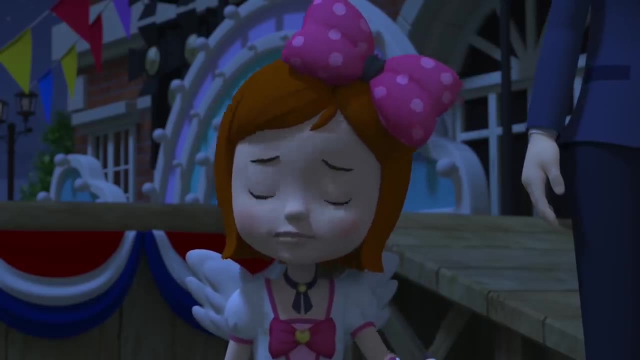 Right, Thank you, Roy. Cindy, Thumbs up on your dancing tonight. Oh yeah, You were great up there, you know. Thank you guys. It's weird that we worked so hard and now it's all over with. 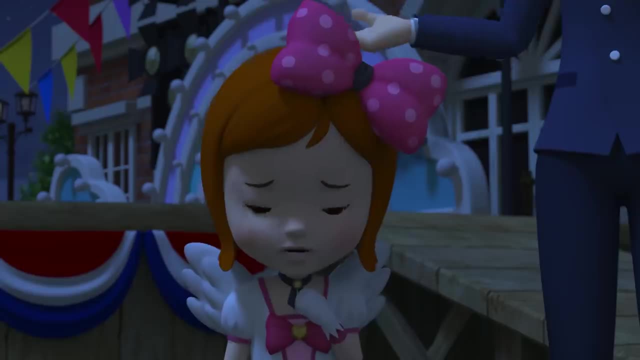 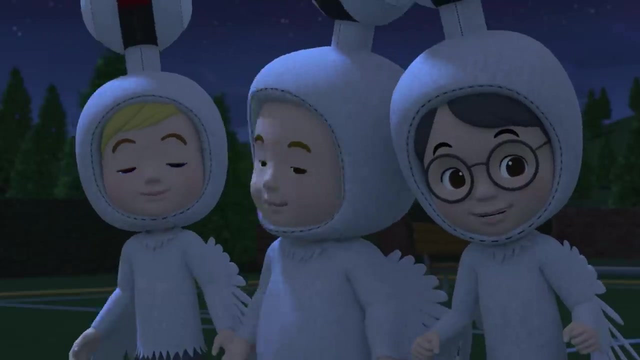 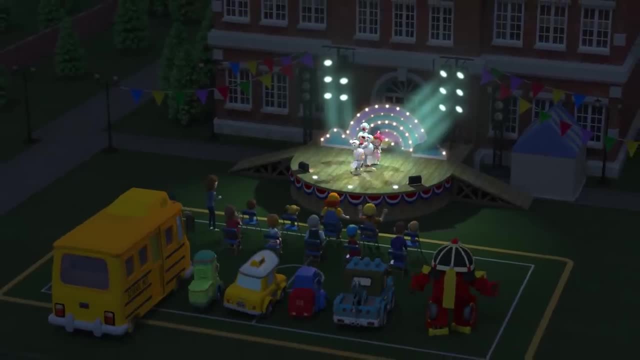 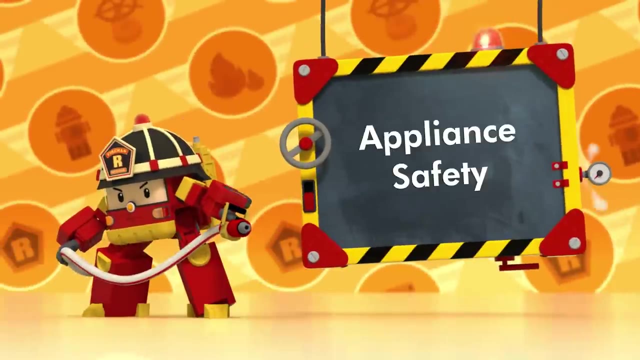 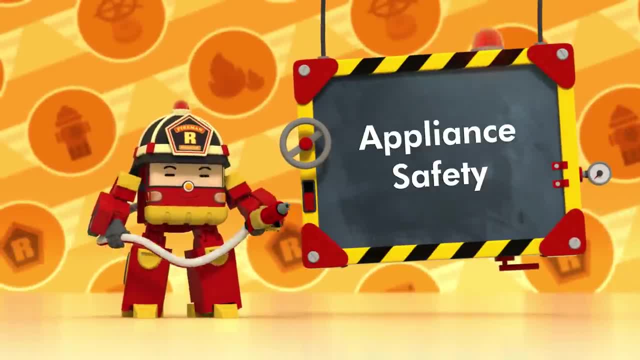 No, We have to see where you are going. We need to make sure the conferencing room won't be scared of you. Let's wrap it up. Oh, that's so funny. I love it. It's what makes us guys. 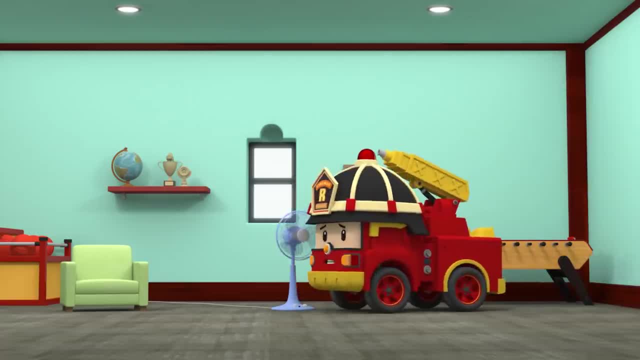 That was wonderful, I did it. We've gotta make the experiential class in the summer. Yay, I'll do that. It looks like you're all ready and ready for class. I'll give you a hand to clear your first Fireball. 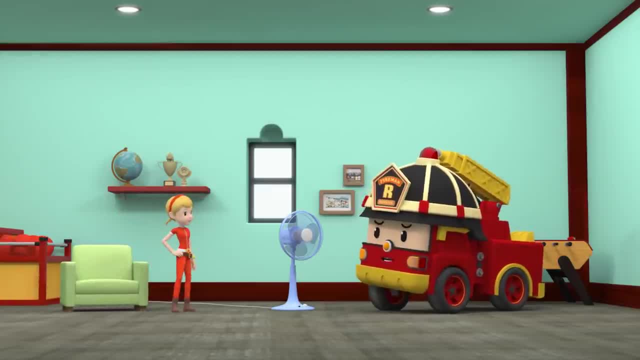 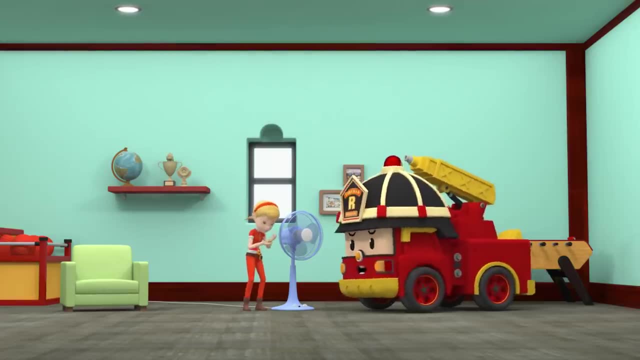 Fireball, Fireball, Fireball, Fireball, Fireball, Fireball. daquiこれは Fireball, Fireball. Ow, it's hot, Are you all right? It's started to overheat. You have to turn it off. 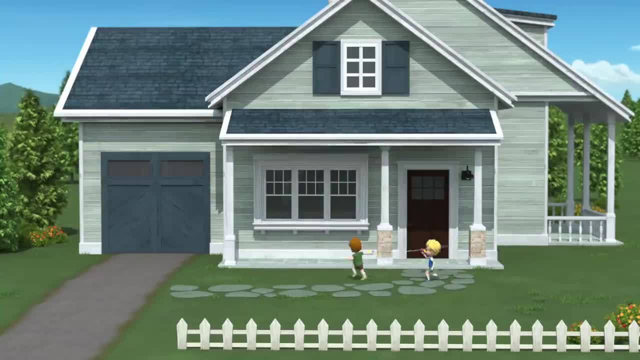 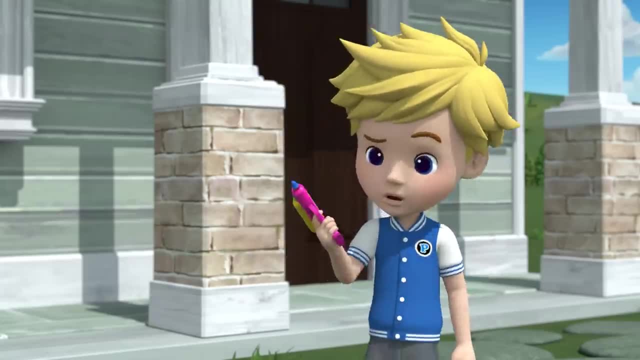 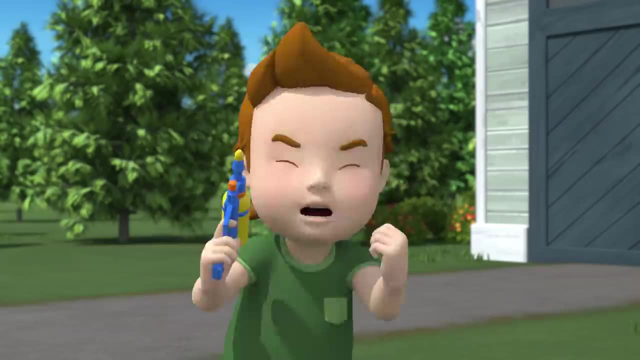 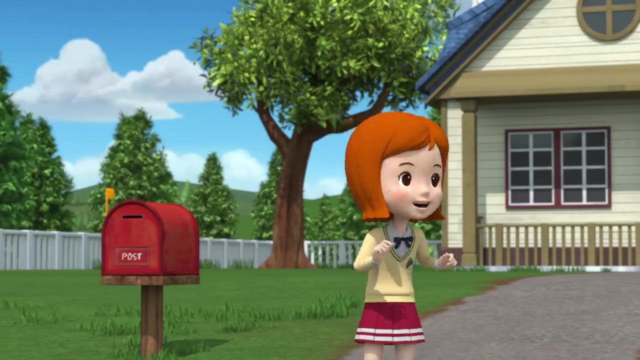 Okay, Roy, Take that All right. Never saw that coming, did you? No water balloons allowed. I got you all wet. Stop right there. Hi Posty, Hello Cindy, You waiting for this. It's here at last. 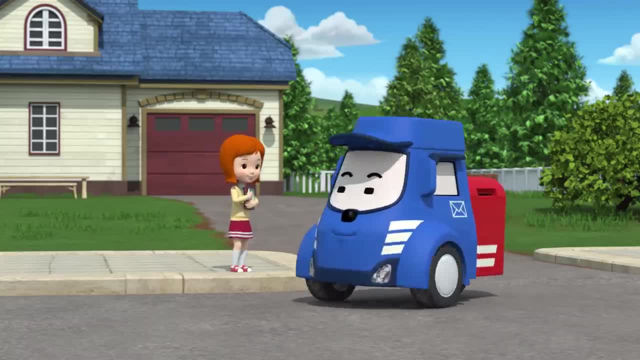 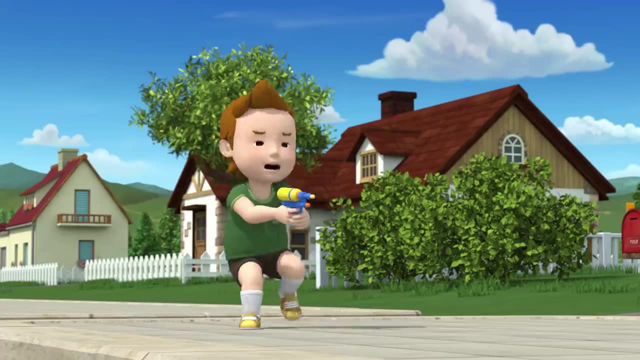 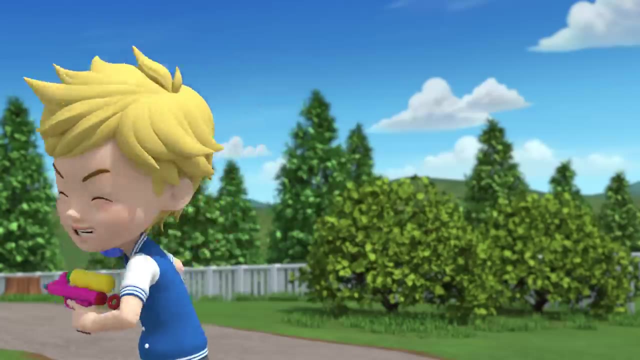 I knew you were waiting for this book, so I came right here. I hope you like it. Goodbye Posty. What Knock it off? Come on, Take your shot. You can't hide behind someone. Please just stop. 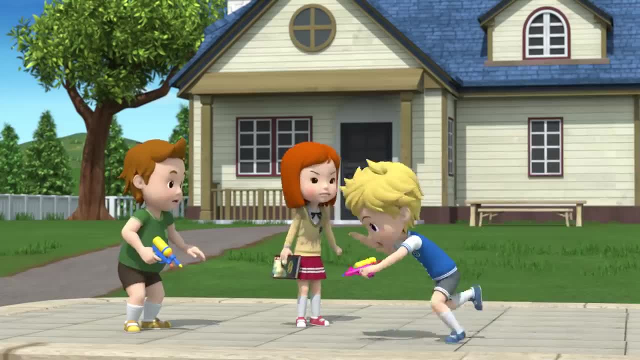 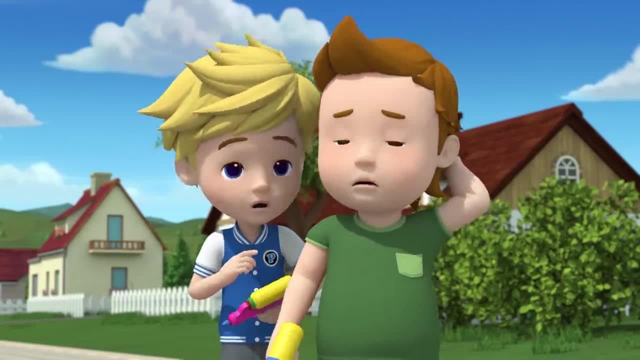 I'll be right back. Oh, Peter, Huh, Huh. Peter, You just got my brand new book all wet. I um, I'm really sorry about that. I know We can take it and get it all dried off. 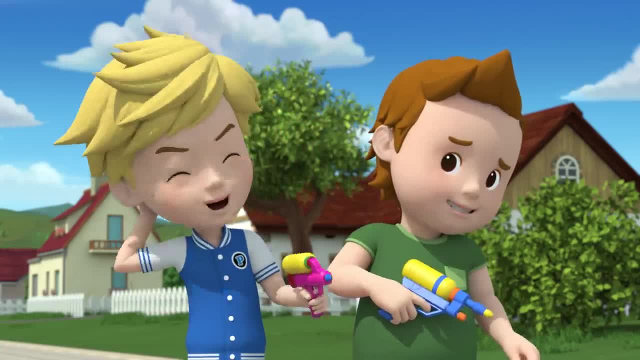 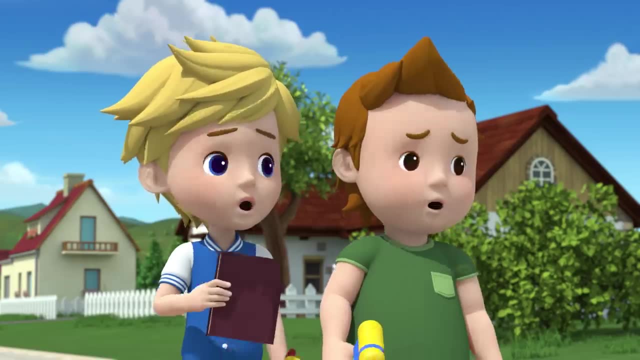 You'd do that? Yeah, Of course we would. Uh-huh, That's right, We'll make sure it's as good as new again. Give it here. You better fix it. Hmph, Hehe, Oh, Johnny. 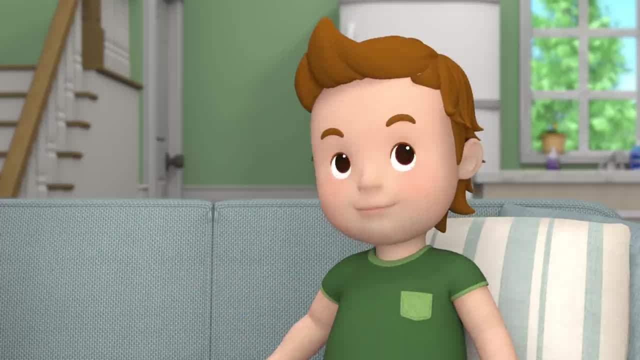 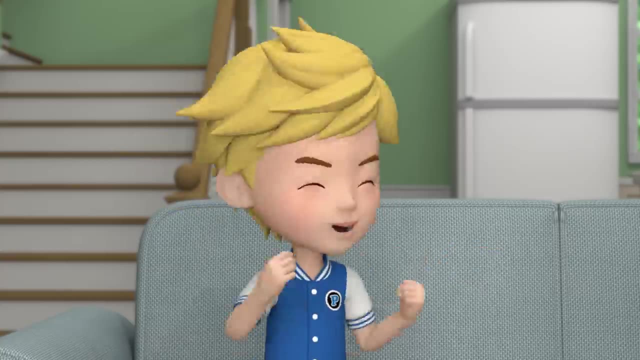 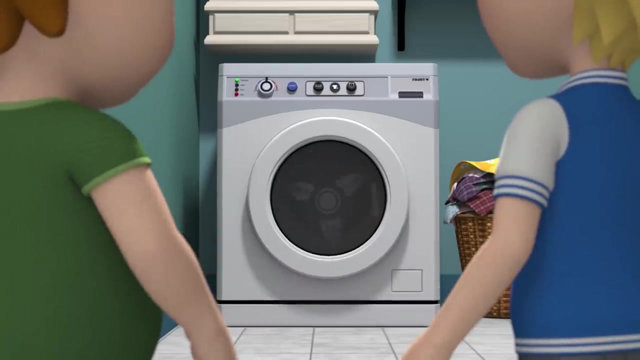 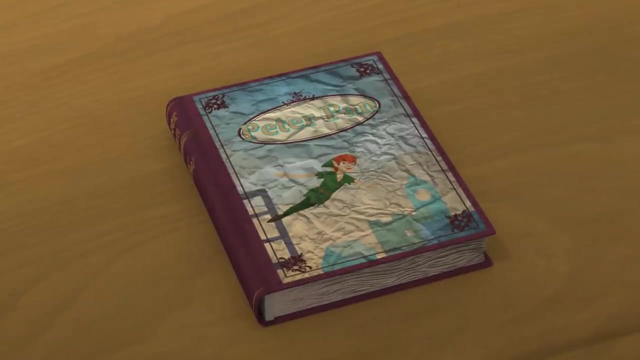 How are we supposed to dry this book? Who knows, Um, maybe the washing machine. How The spin cycle, Johnny, let me think That's it. Let's do it. Turn it off, Turn it off. Well, that was a fail. 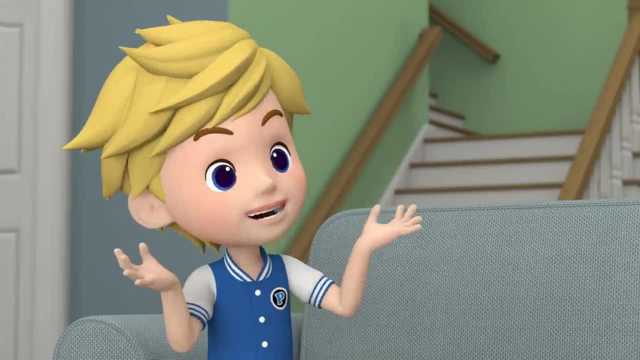 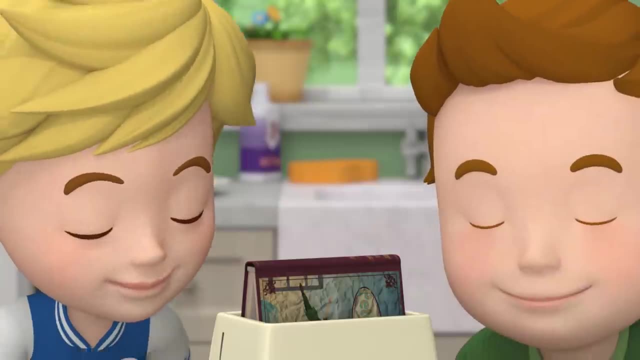 Maybe The toaster might work. It's so hot it'll dry it up. You're right, Peter. you're the smartest kid I know I am, aren't? I Doesn't that smell great? All I want in this world right now is toast. 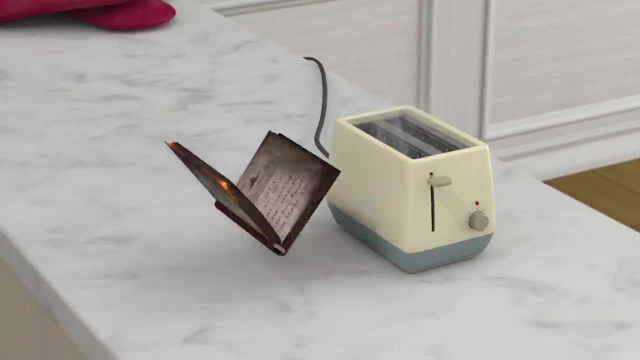 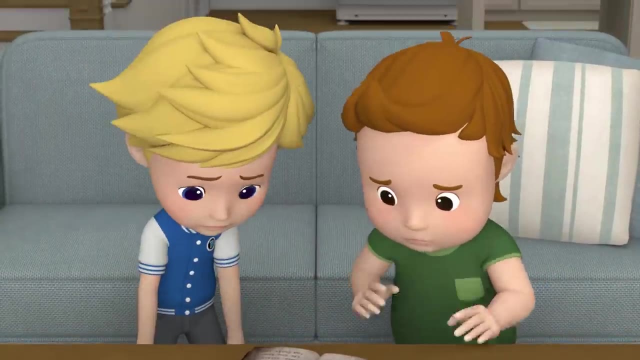 Peter, Look, It's on fire Water. So what should we do? Cindy's gonna be fine. I'll be here soon to pick it up. I got it. The warm air will dry up this book in no time Yeah. 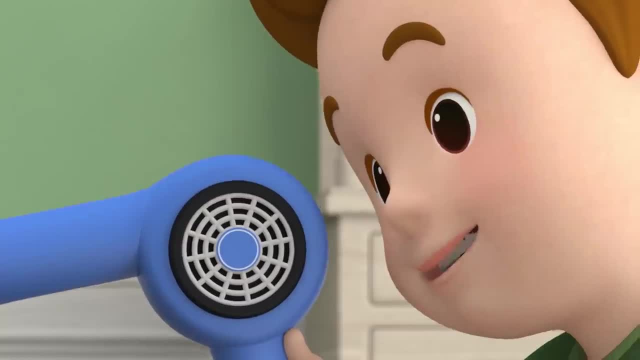 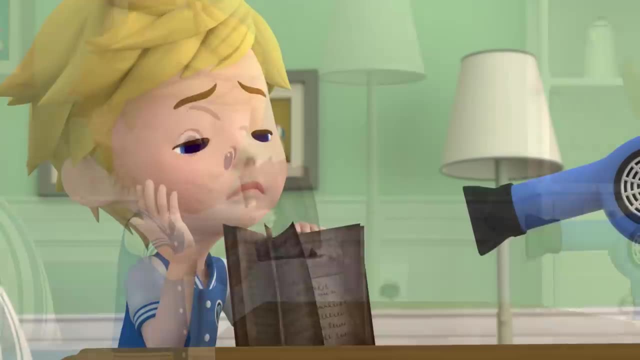 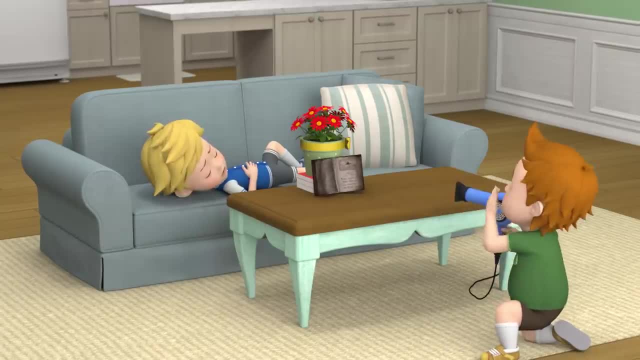 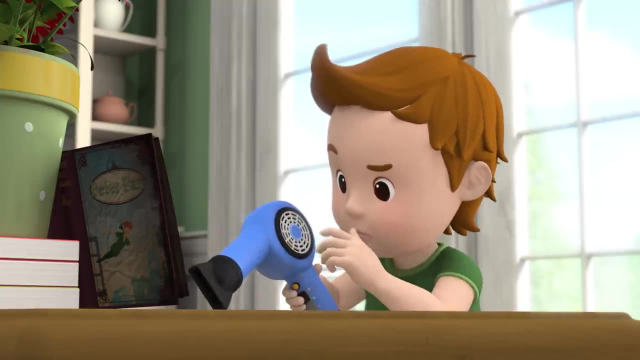 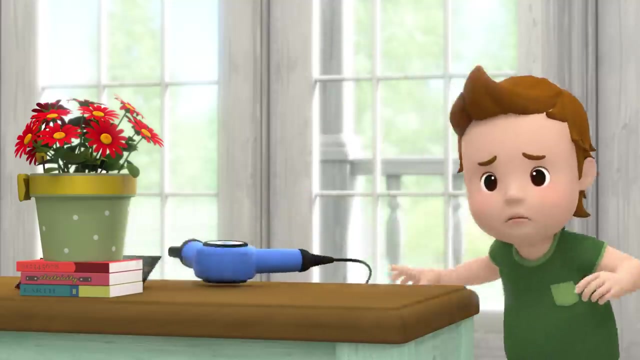 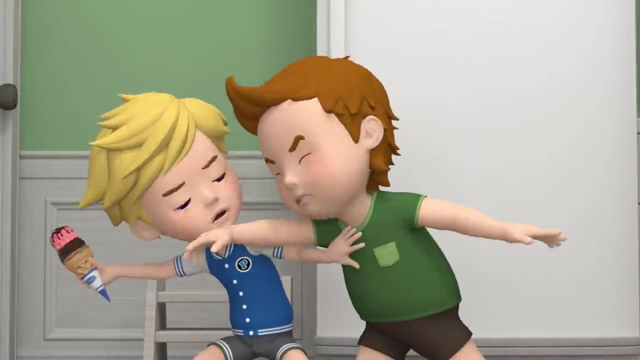 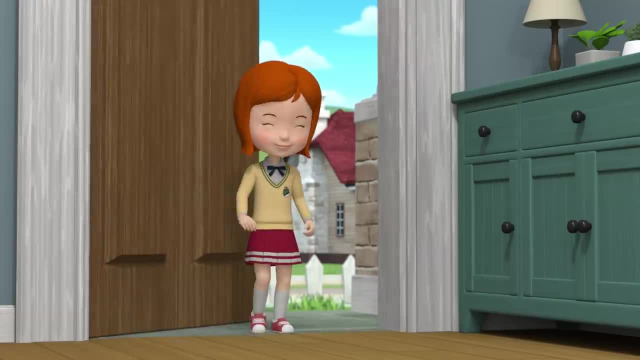 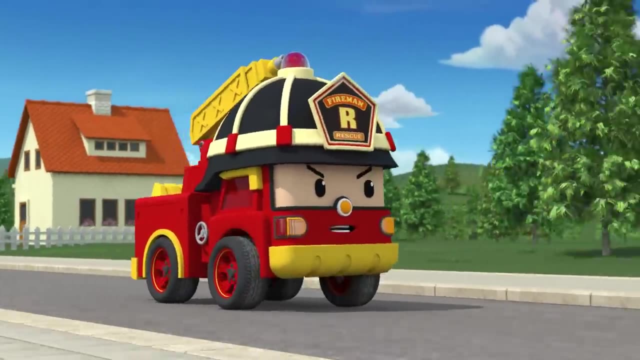 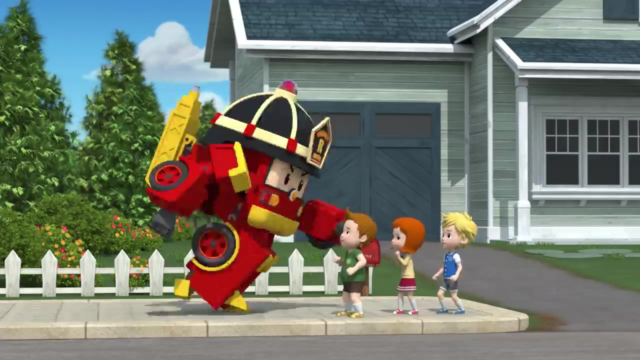 Wait, Why can't I have some? You're in A cicada. Ooh, fire, Fire. It went out. Fire, Fire. Huh, Is that smoke at Johnny's house celebratedbl스가. Hey kids, are you all right? Just stay right there. 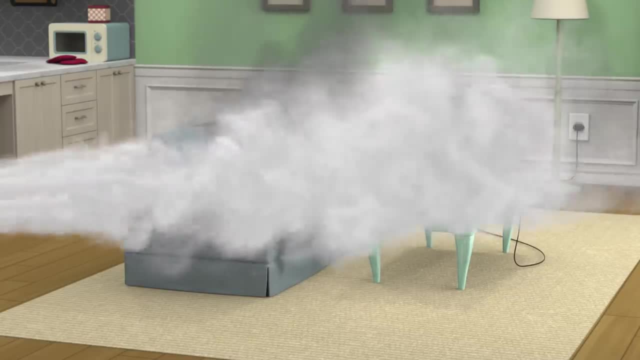 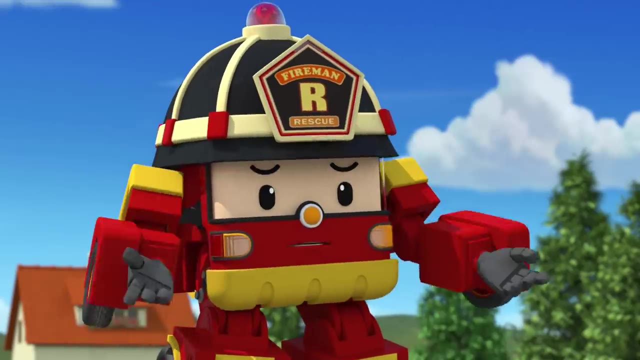 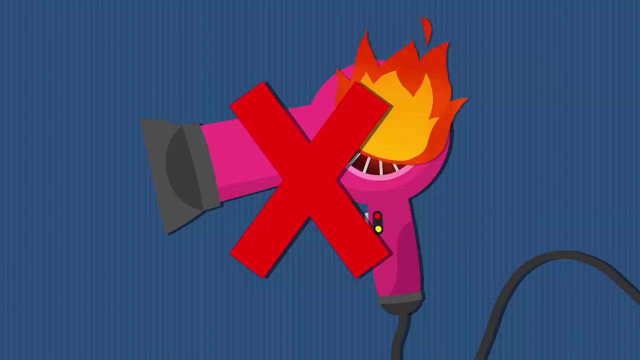 Is everybody okay? We're okay now. all thanks to you, Roy. You guys, you can't leave an appliance on and unattended. Small home appliances can overheat and catch on fire. So even if you're just leaving the room, make sure that they're off. 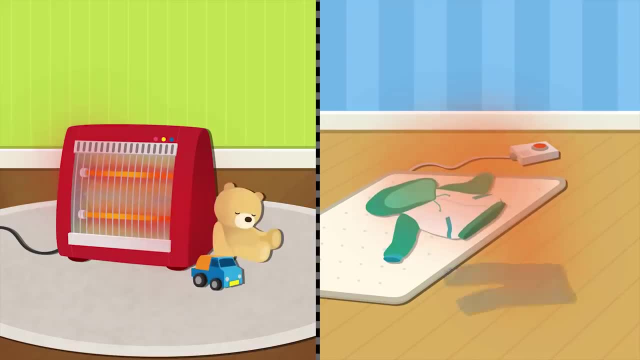 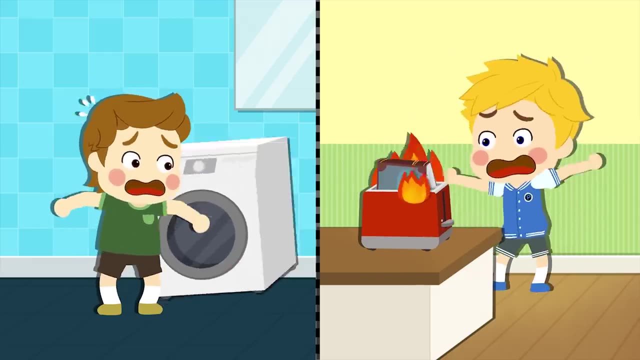 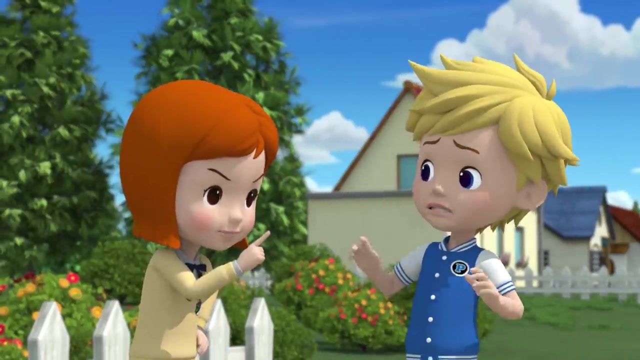 Also be sure not to leave flammable items near electric heaters or blankets. And last, only use appliances for their intended purpose. Okay, we get it now. Hold on. Whatever happened to my book? You better hope it wasn't damaged in the fire. 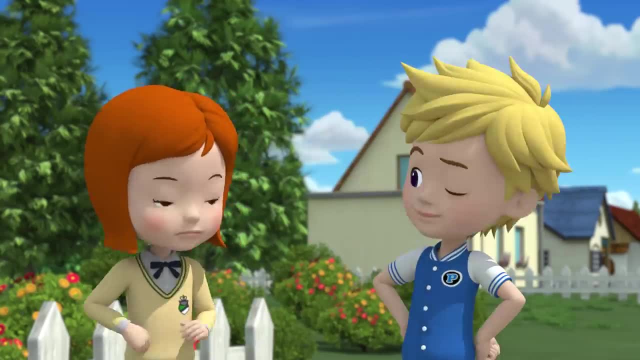 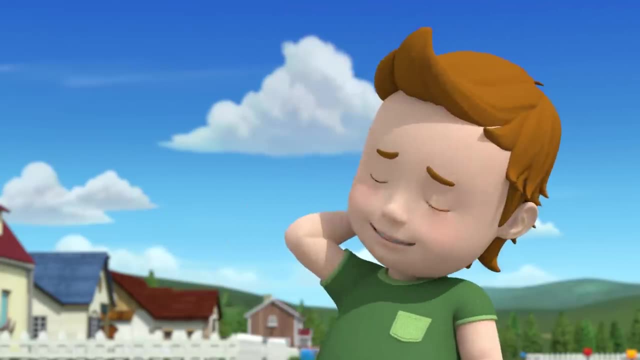 Come on, Cindy, You can always trust me to take care of things. It's fixed, It's not wet. Here you go. What happened? What happened to it? Uh well, a lot of things. We'll have to tell you the story sometime. 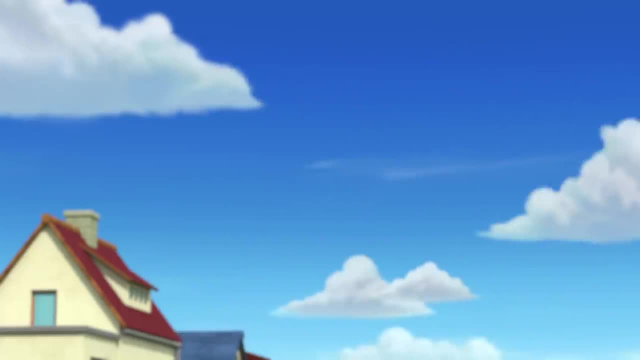 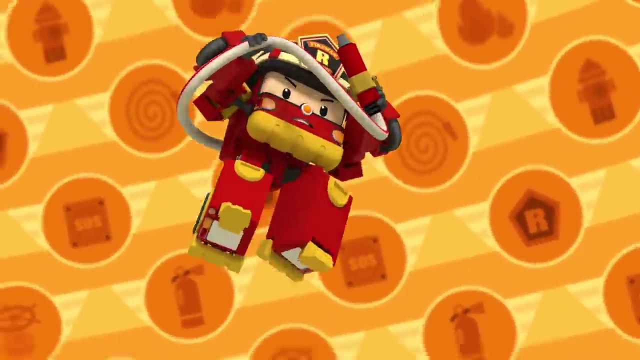 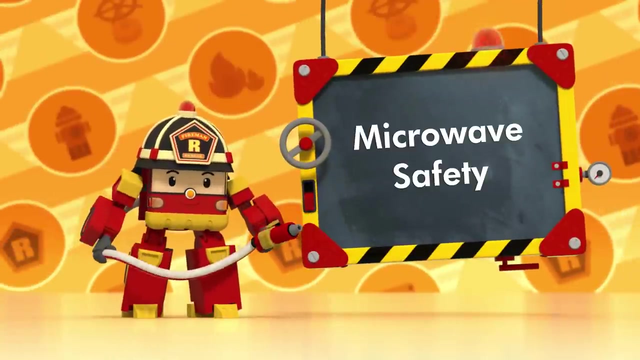 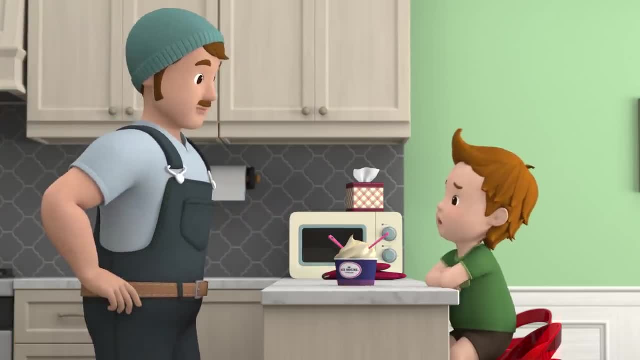 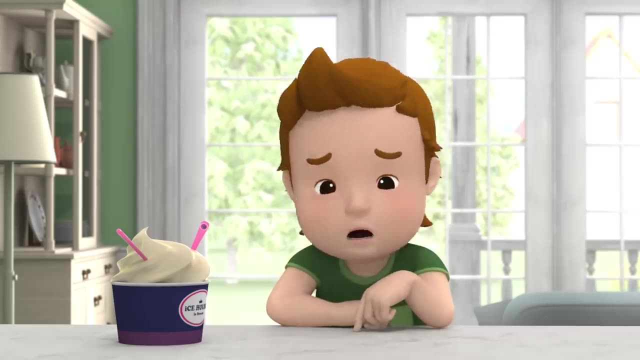 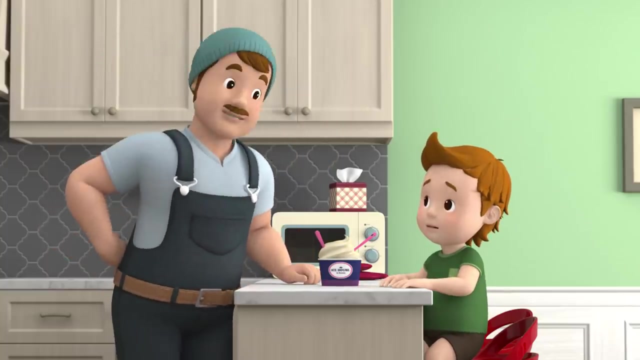 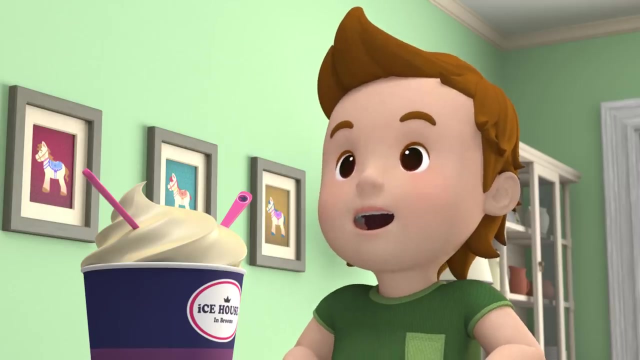 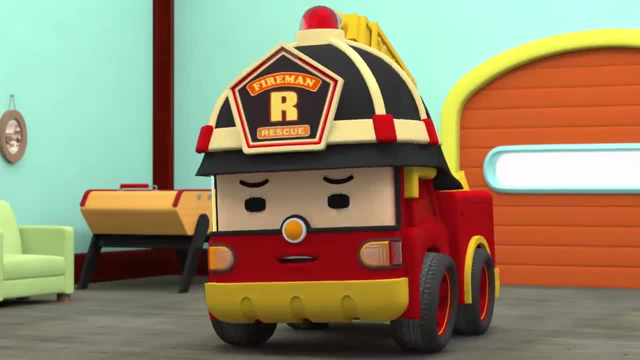 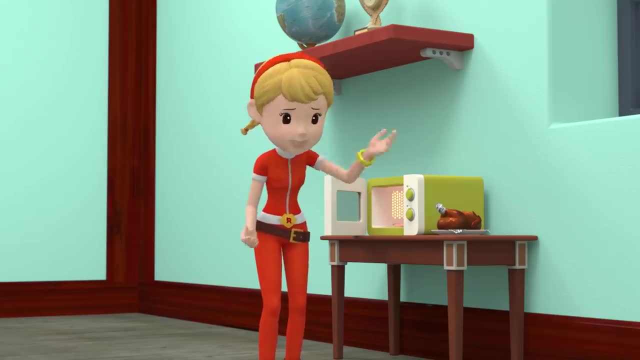 Oh, hi Roy. What is it? Jin, you can't put foil in the microwave, It'll catch on fire. Oh, how did I forget? I use the microwave all the time, so I guess I better be more careful. 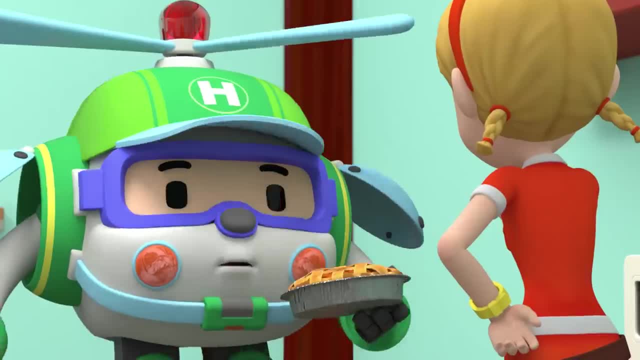 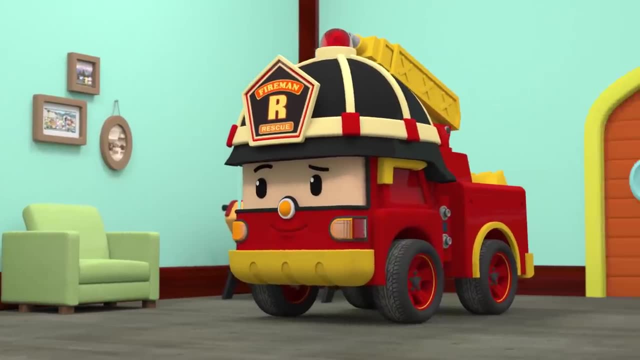 Jin, are you finished with that? Huh, Hallie, stop. Huh. How come, If you put that foil in the microwave, it could catch on fire? It could, Hallie. everybody knows that. Hey, did you pass the quiz. 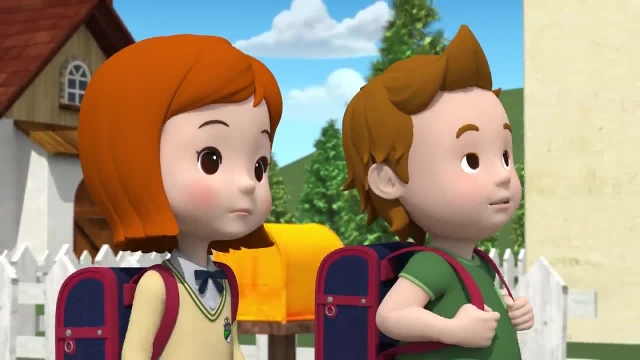 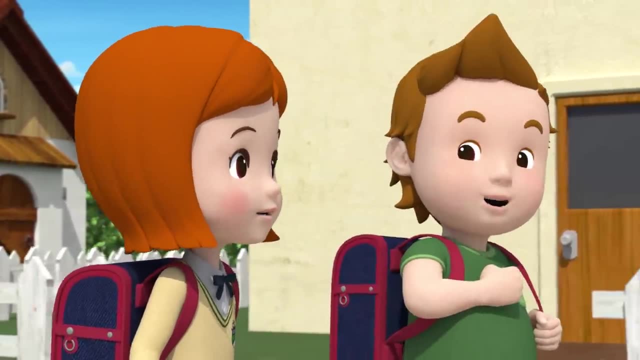 Yeah, I think I did, but I guess we'll find out. All I keep thinking about is an ice cream sundae. Huh, Johnny, I love ice cream. It's good right, I make great sundaes Awesome. 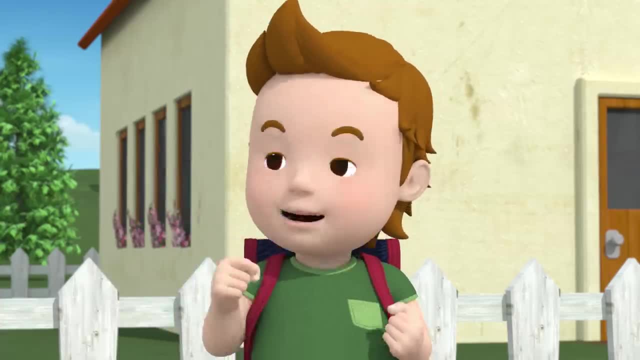 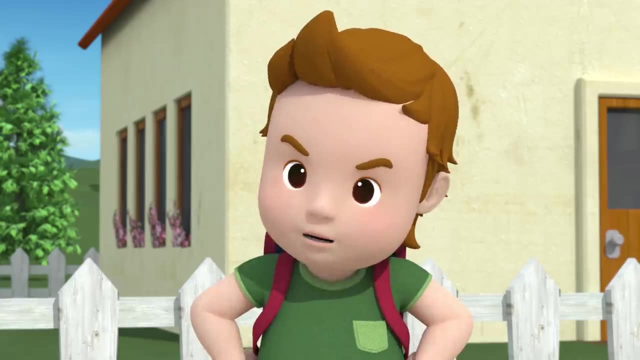 Cindy, come with me, I'll make you an epic sundae. Would you rather have chocolate or strawberry? Well, um, Chocolate, Me too. What I never said you guys could come, You just said you were making sundaes. 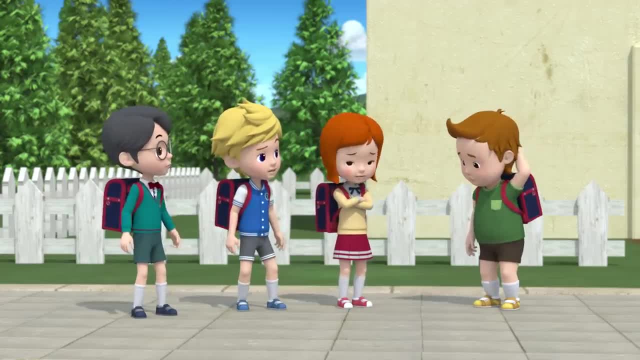 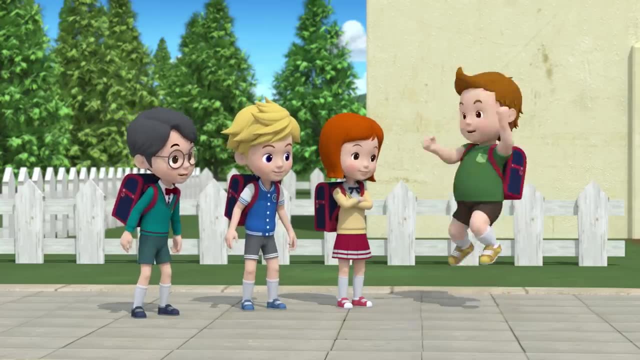 Yeah, but not for you. Come on, you guys. It's annoying when you always argue. And I like strawberry. Oh, great choice. Come on, Sundaes for everyone, All right, Hello, Oh, hi, kids. 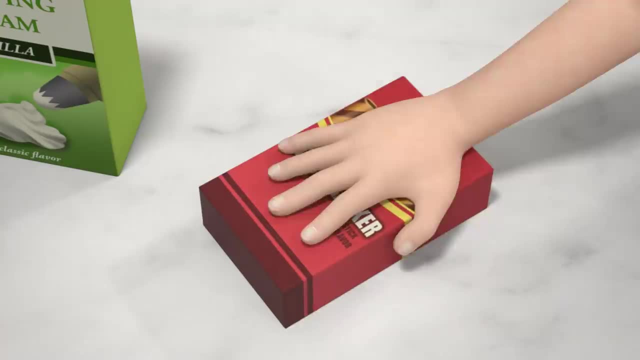 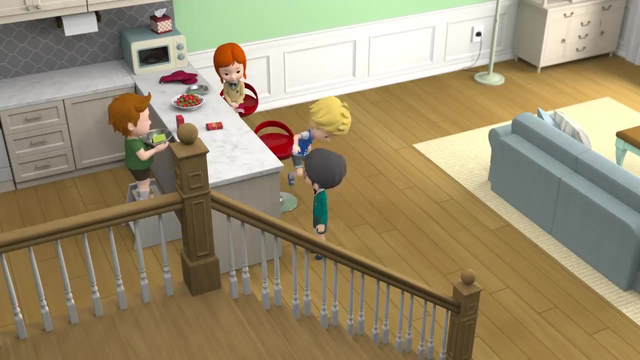 Ta-da, Whoa, Jackpot, Stop it. Those are for the sundaes. Huh, Charles and I are gonna go play games. then Call us when they're done. Come on, Charles, Wait up Huh. 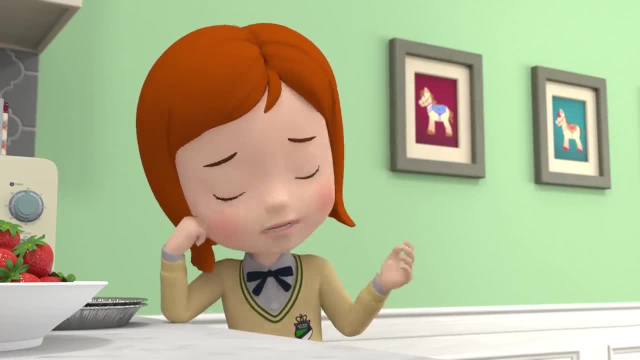 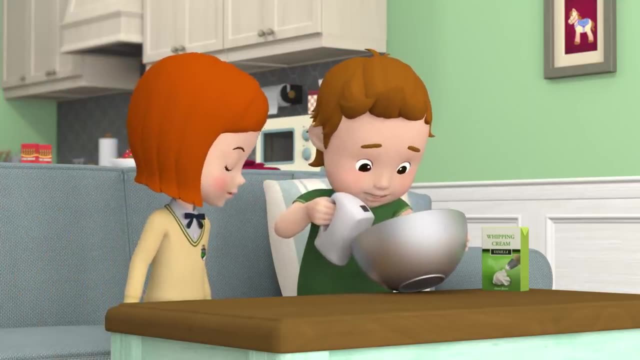 I'll never get why you can't just get along. Huh, Johnny, Huh. What are you making with that? Uh, whipped cream. To make a good sundae you need homemade whipped cream. Ah, Are you all right? 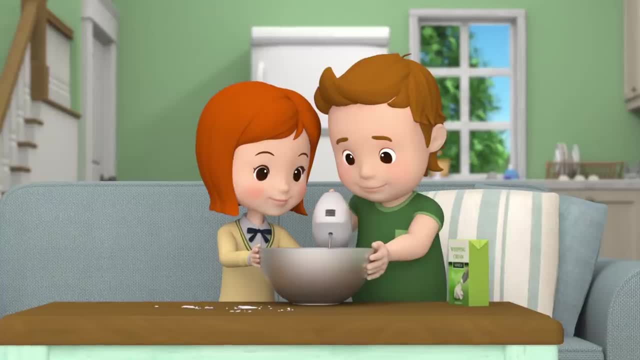 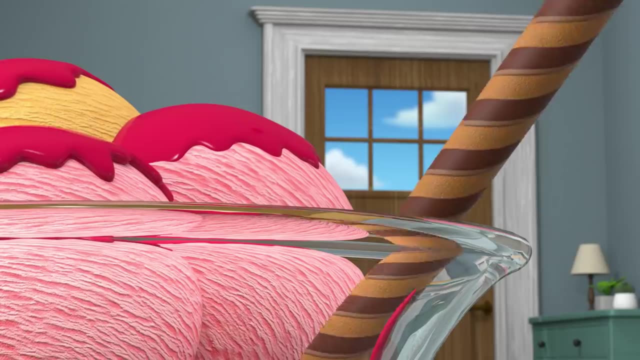 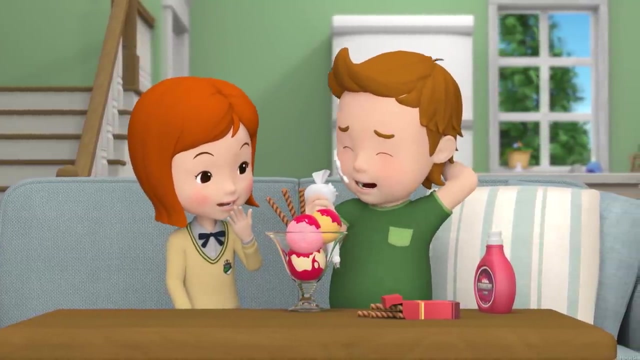 Would it be better if I held on like this. Um, Here we go. Oh, Oh, Ha-ha-ha. Hmm, Mmm, Mmm, Ugh, Uh-huh, Mmm, Hmm, Ha-ha-ha-ha. 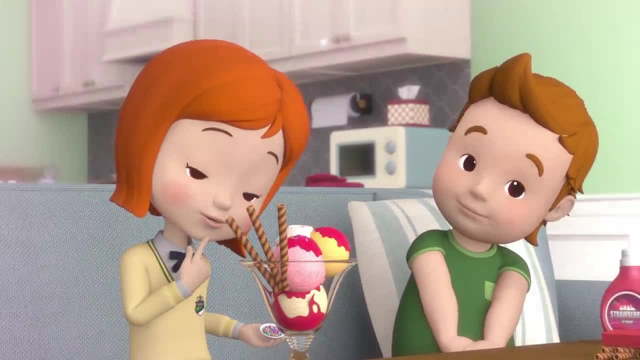 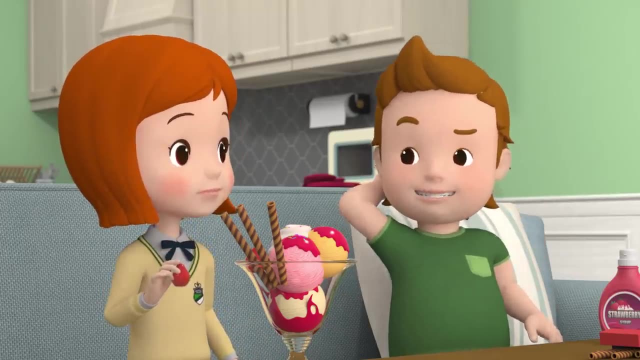 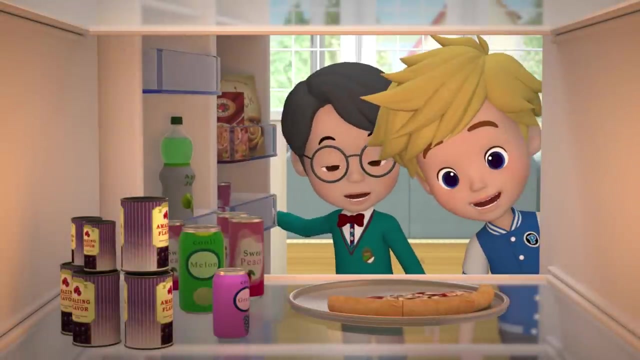 Hmm, Is this a dream? Huh, Uh, Uh, Uh, Johnny. Uh, There was a fly, Johnny, can Charles and I have a snack? You can see if there's anything you want in the fridge. Ah, Pizza time. 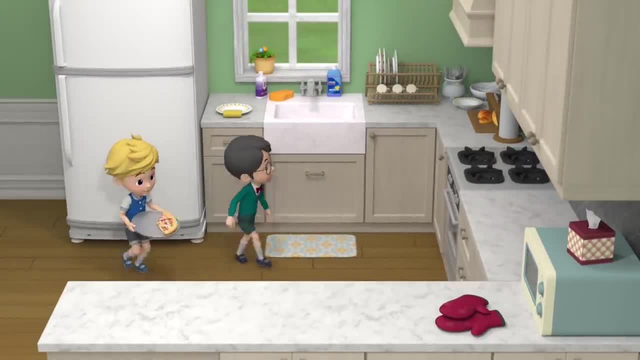 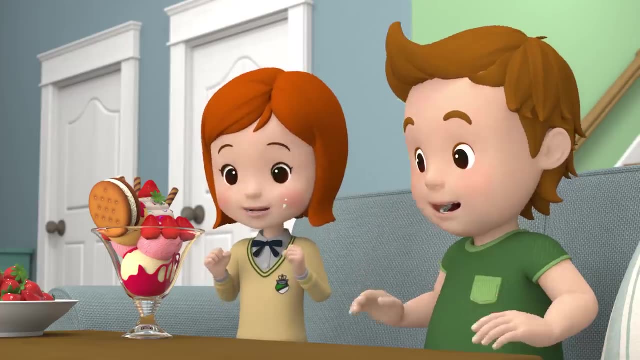 Do you think we should heat it up? Yeah, And I'll get us some plates. Huh, Wow, That looks delicious. Wow, It looks great. Aw, It belongs in a magazine. Ha-ha-ha-ha. What's so funny? 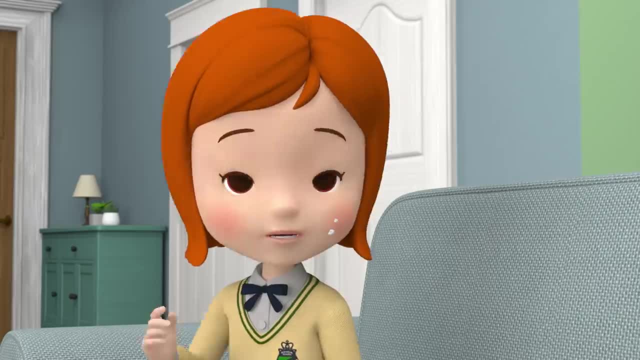 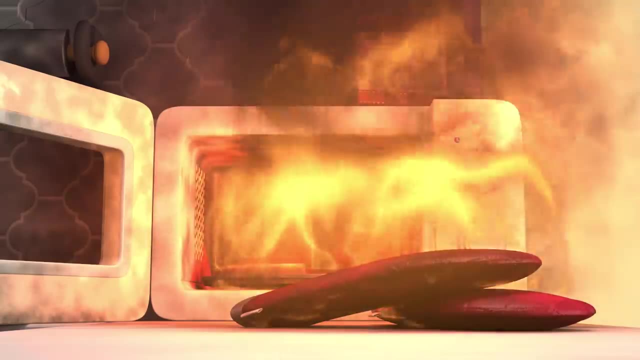 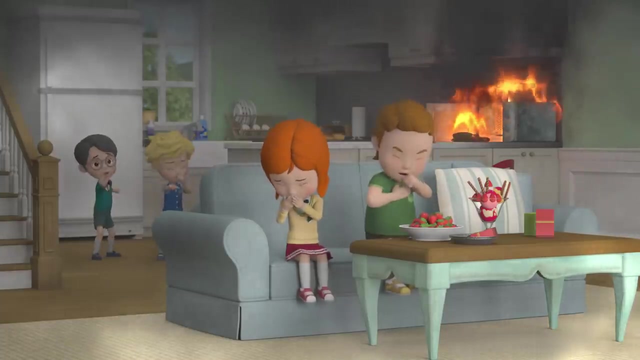 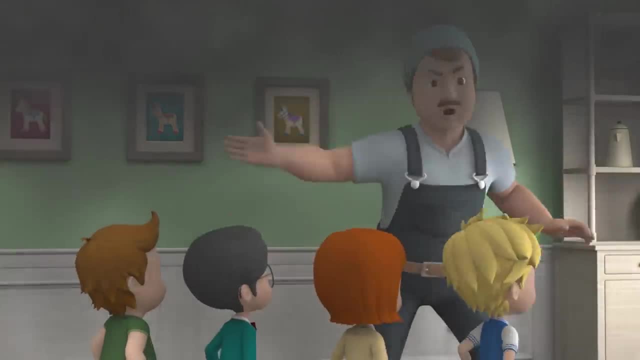 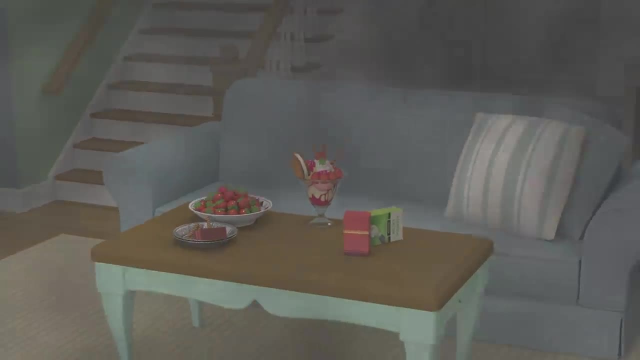 Get out of the house right now. Come on Our sundae, Ah, Ah, Ah, Our sundae, Ah. Come on, Johnny, Our sundae. Fire, Fire, Fire. Oh, We have fire. There's smoke at Johnny's house. 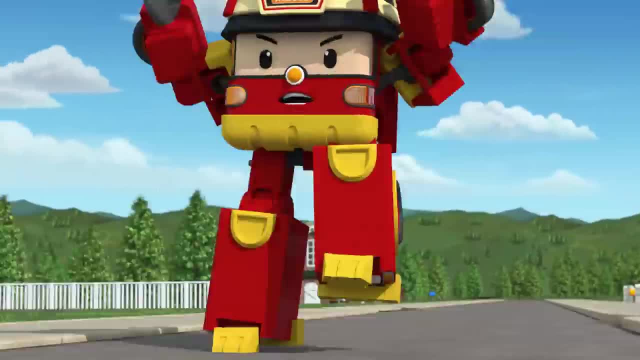 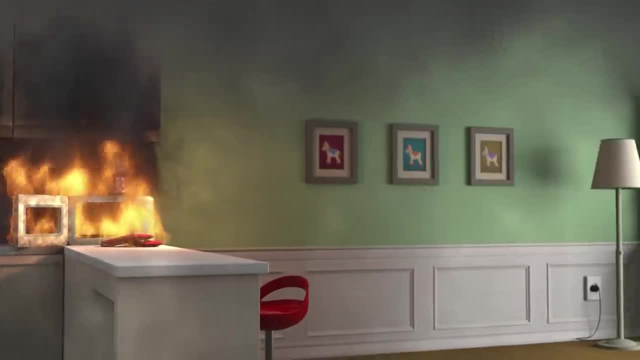 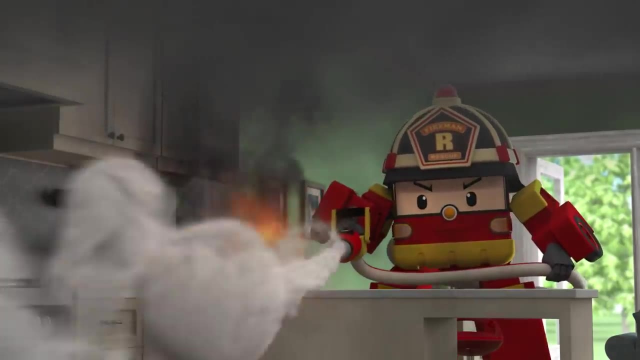 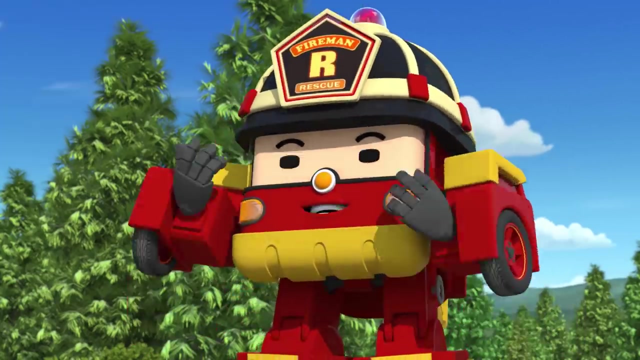 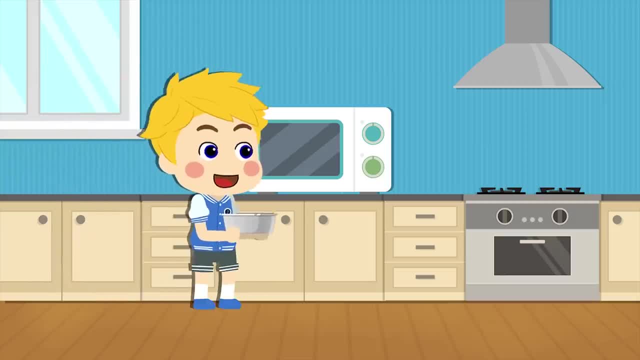 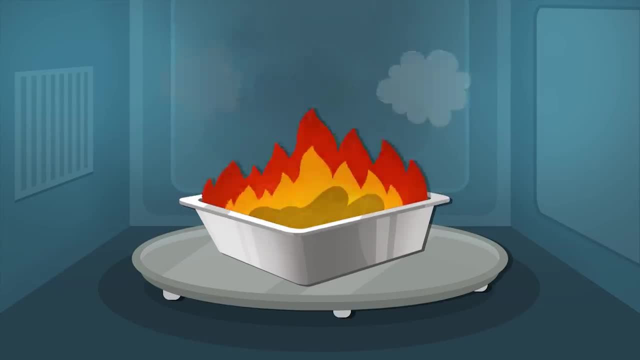 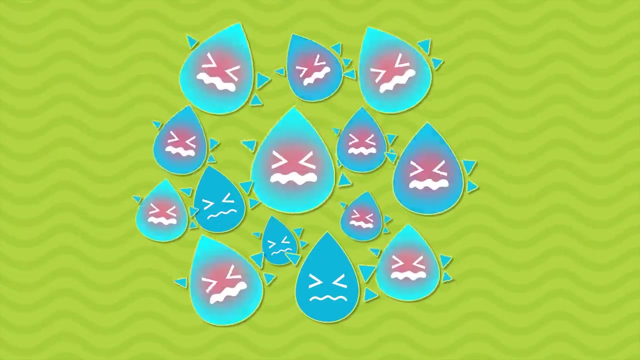 Ah, Ah, Ah, Ah, Ah, Ah Man, Oh God, Uh-oh Shit Hide Save Argh occupied Argh. Merci Ik sixty Ever To Those Young Watch. 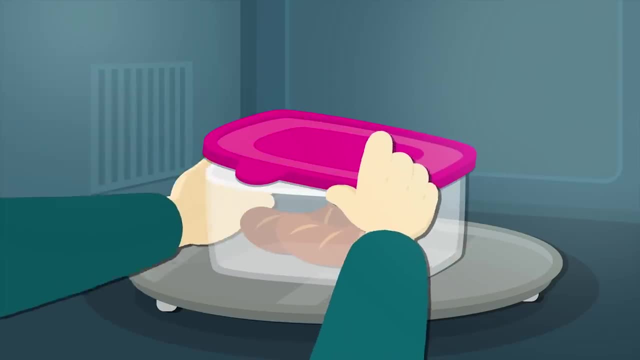 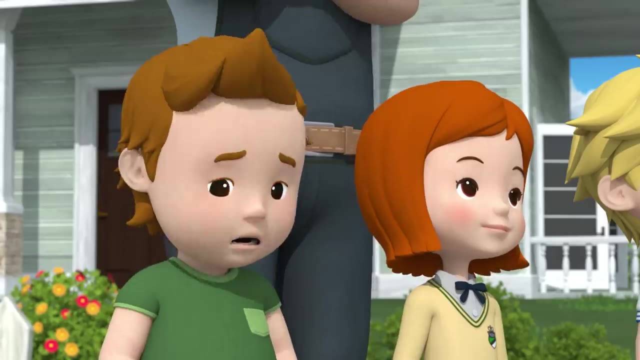 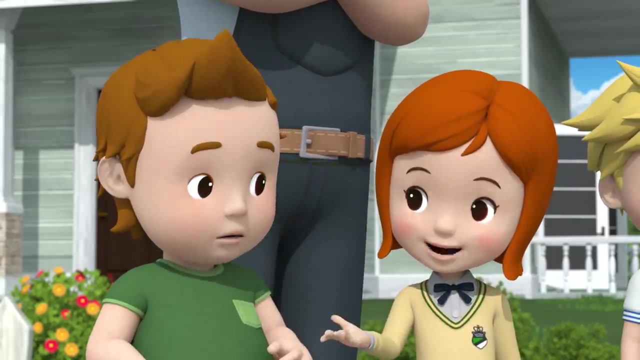 The funciona, Don't do something. unsealed containers to keep them from bursting as well. simple, right. yes, we can do all that. our poor sunday. cindy and i worked so hard on it, yeah, but we had a lot of fun. right, we'll just make. 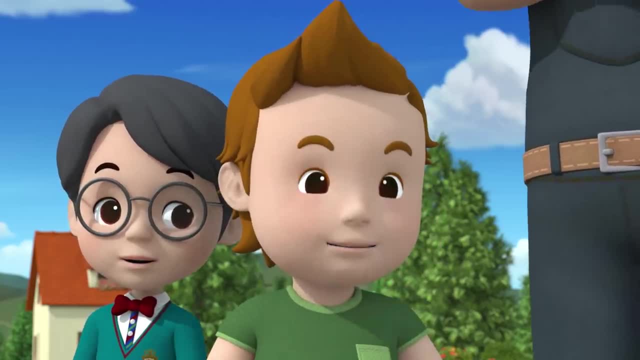 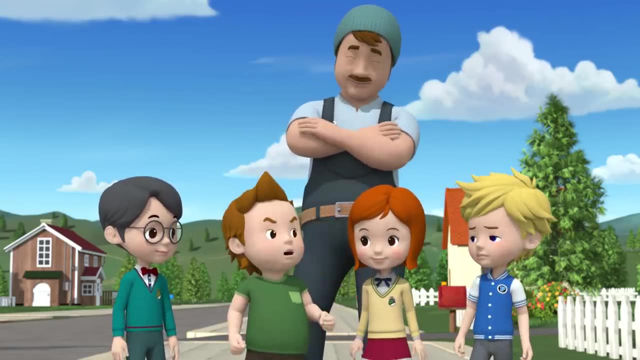 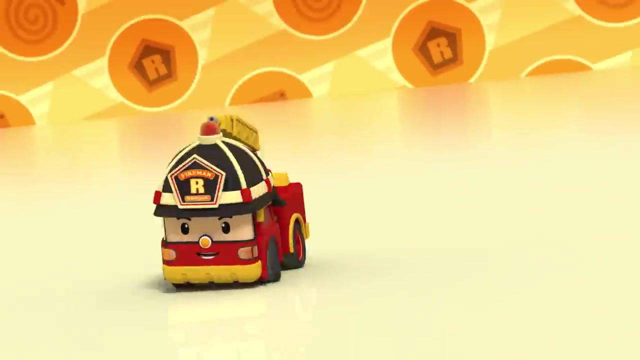 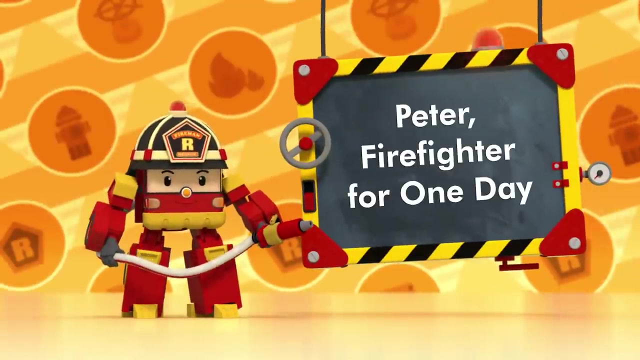 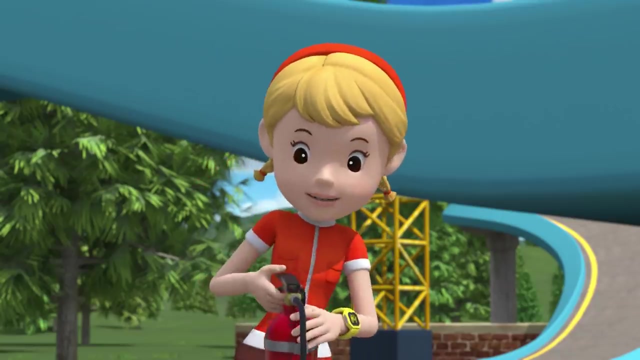 it again, can we? ah, you're right, that would be really great. all right, just don't forget, i like chocolate the best. peter, you're never coming over to my house again. oh, i see, only the pretty girl gets the ice. peter firefighter for one day. guys watch, pull the safety pin out, point the nozzle in the direction of the fire and give. 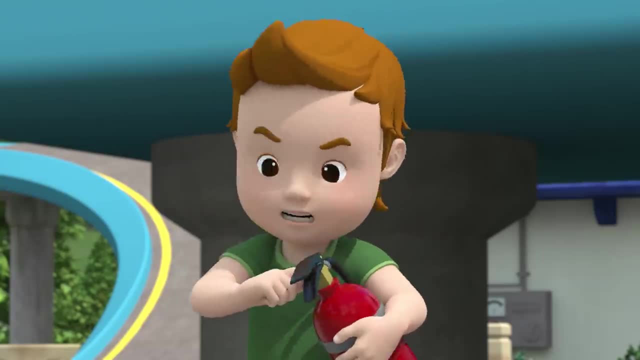 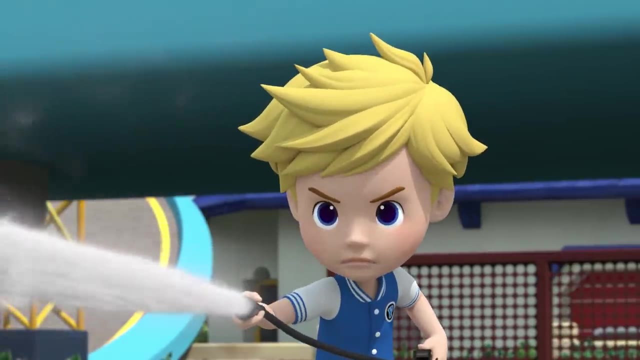 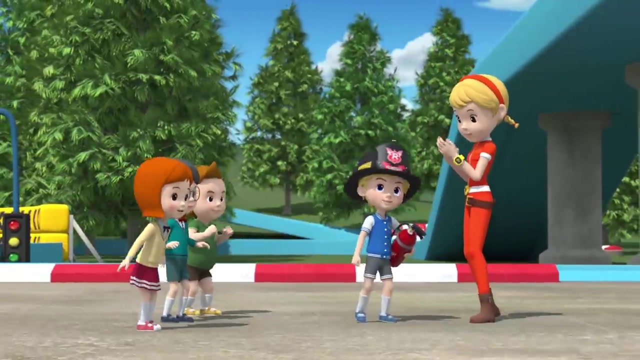 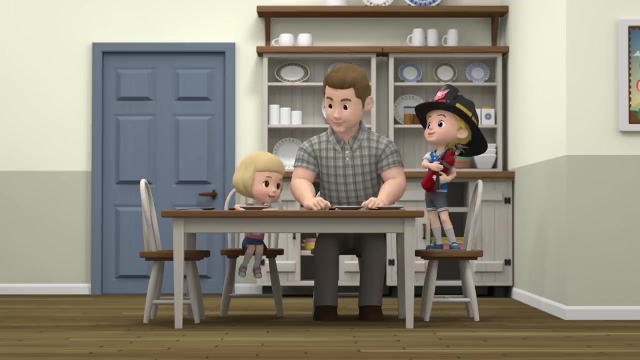 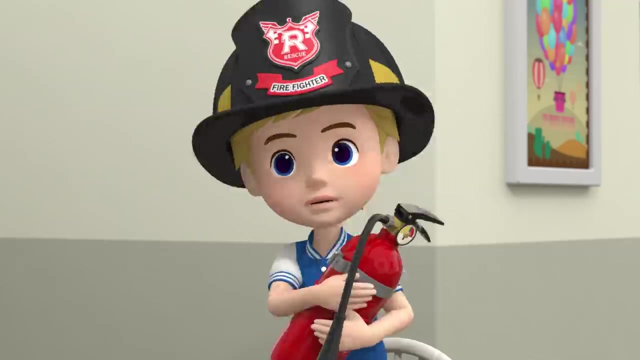 the lever a squeeze, give it a try, uh, the pin won't come out. hmm, ha you, peter. congrats on being a kid firefighter. wow, awesome, yeah, wow, you look like a real firefighter. i'm proud of you. son, i'll find a good place to put the fire extinguisher. no, you won't, mom. the safety of our house is in the 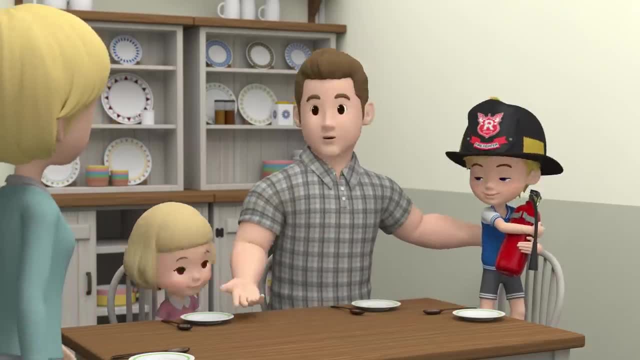 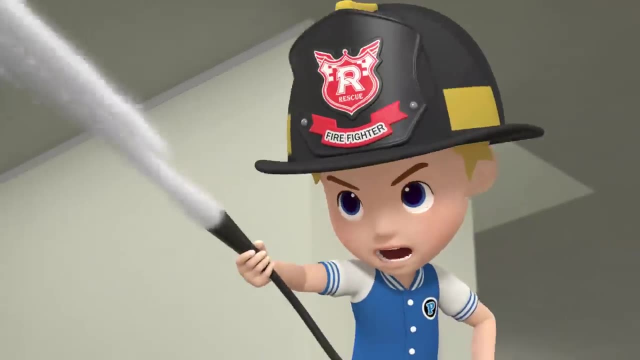 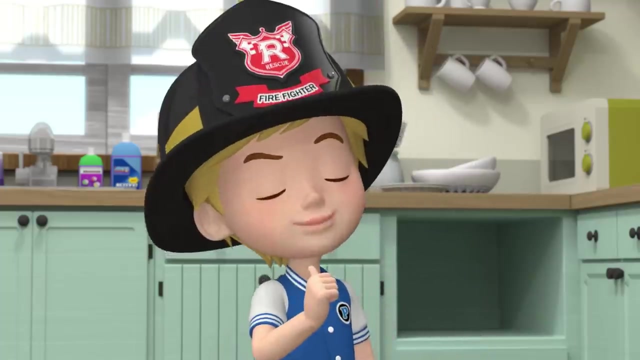 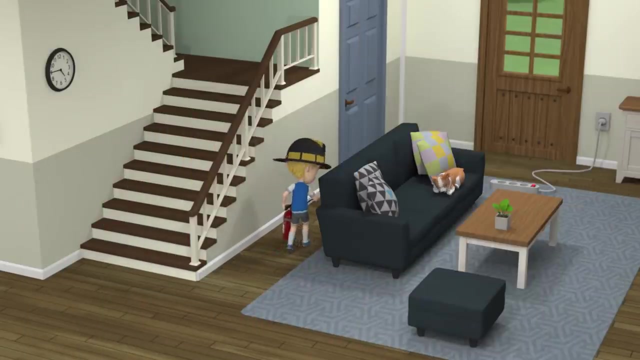 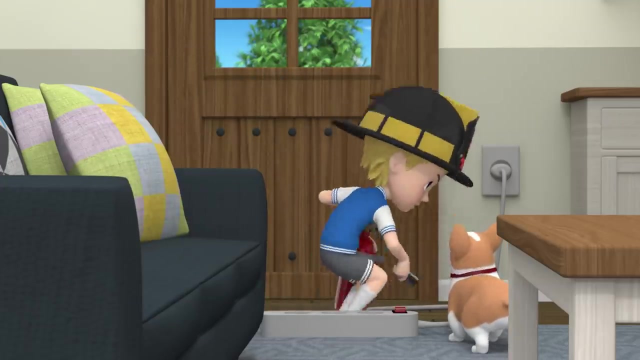 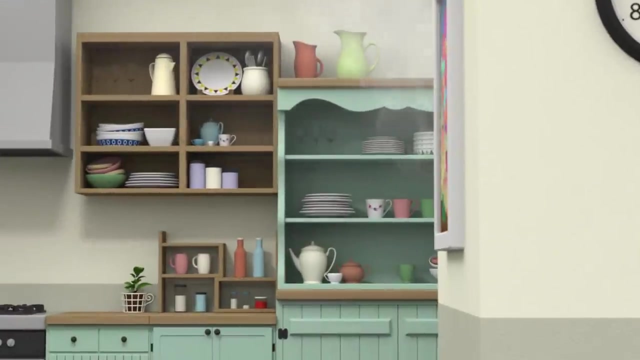 hands of the fireman. he's right, let him be the fire expert. huh, everyone's safe. am i a real firefighter or what? wow, peter, that was really awesome. my brother's the best. whoa easy, buddy, keep back, it's dangerous. hmm, look safe, huh, is that? 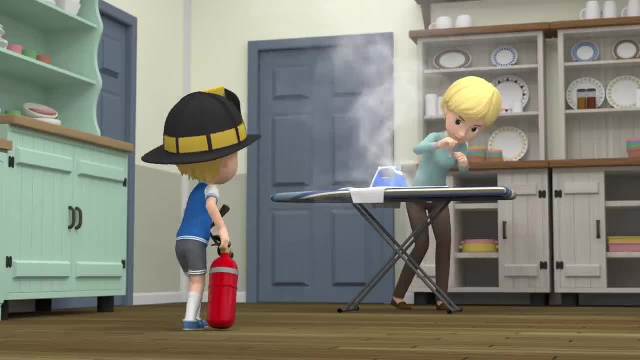 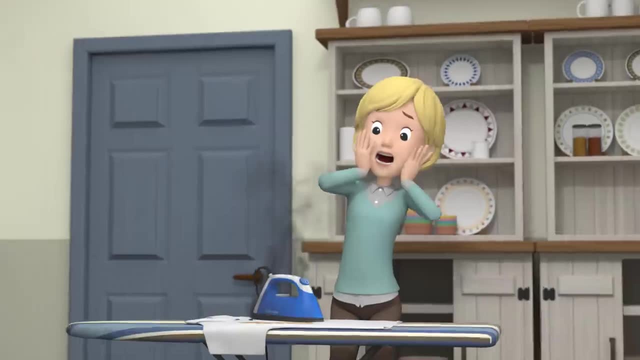 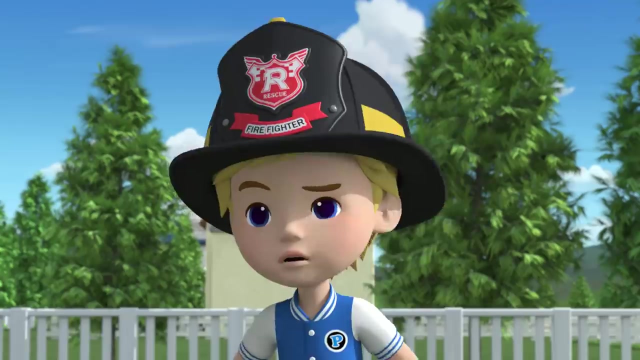 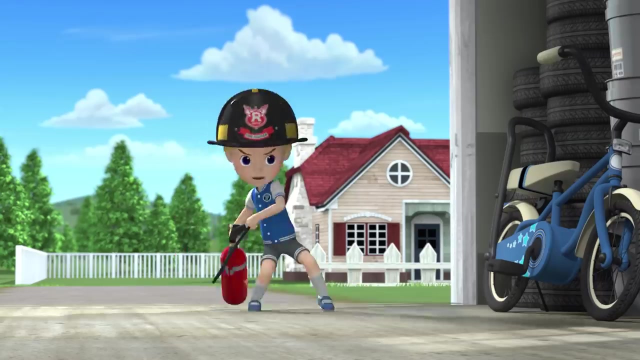 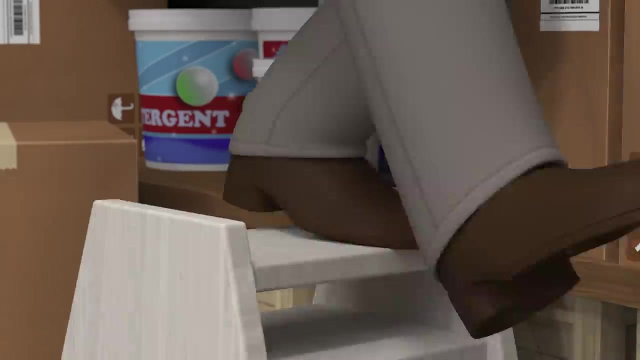 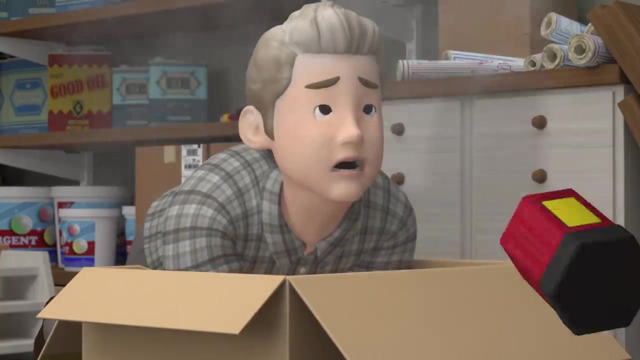 huh huh peter. oh man, i thought it was a fire. goodness, i was scared. huh, ah, my clothes are burning. huh, huh, huh, huh. what is that could be? hmm, dad, i'm here, clear out. huh peter, there's no fire. huh peter, there's no fire. hm um. 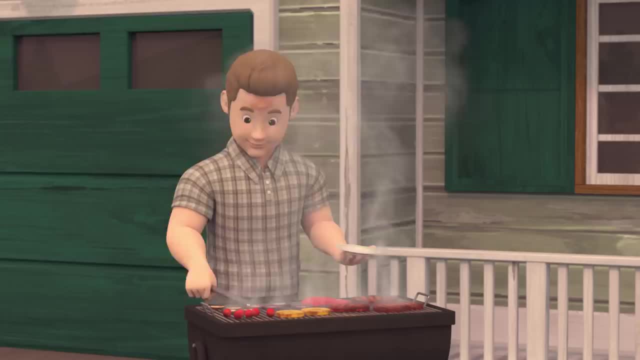 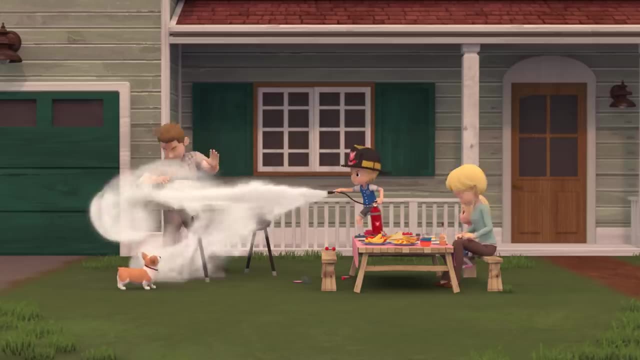 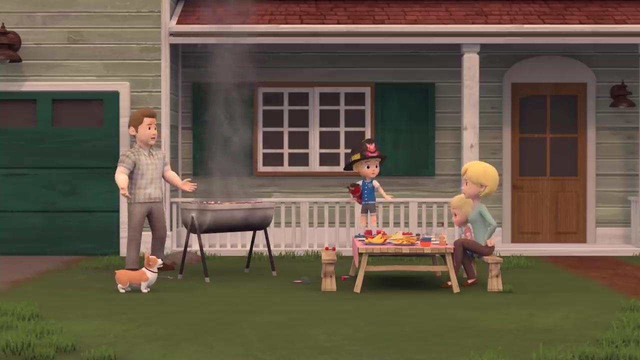 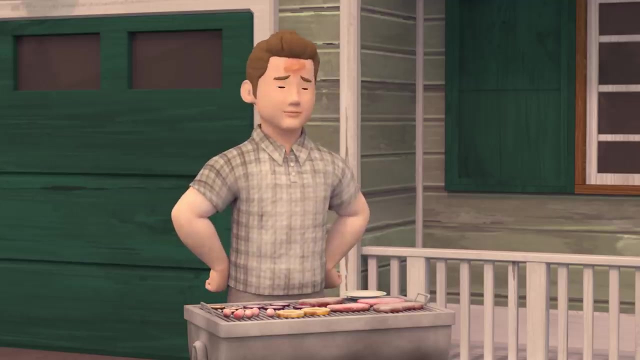 smells really, really good. honey. is it ready? yet we're almost there. huh a fire a fired. huh a fire, a fired. Ensuite. Oh Yeah, Well, you're on the list, but we didn't accept your proposal. close, Peter, this wasn't a dangerous fire, a little grease just dropped on the 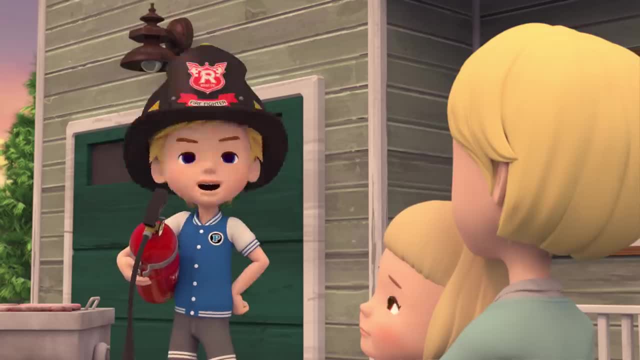 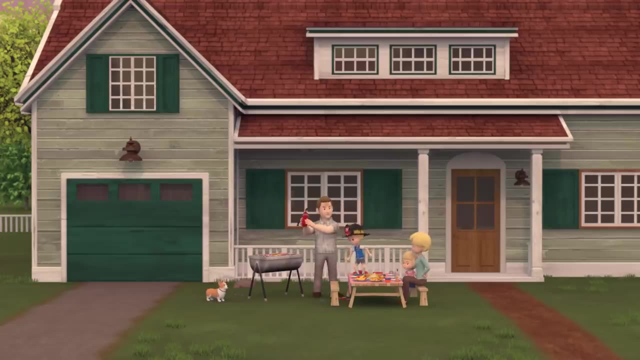 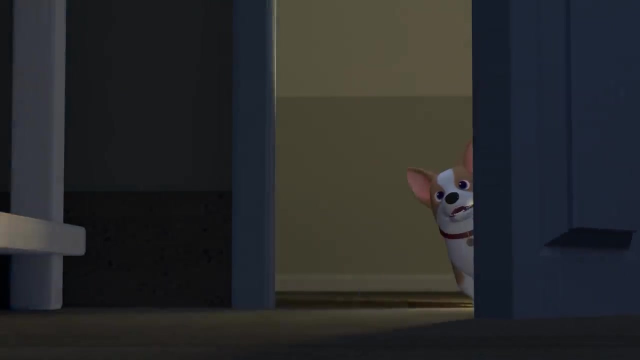 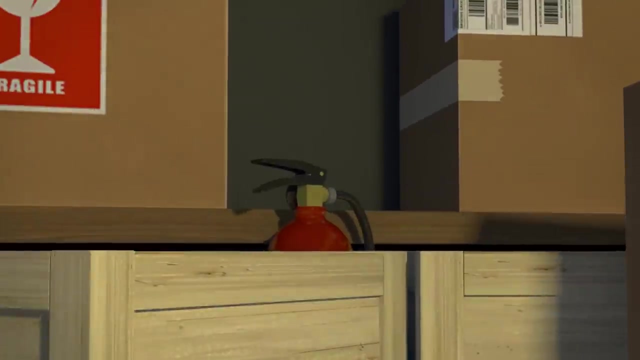 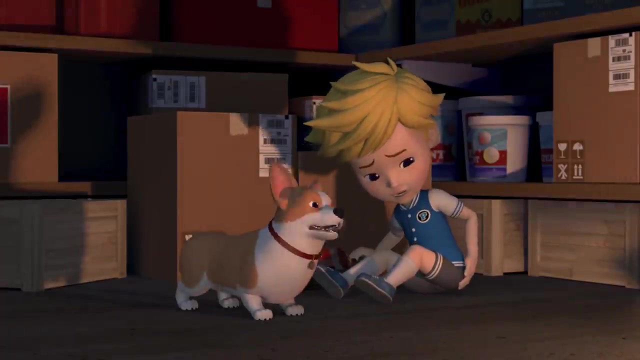 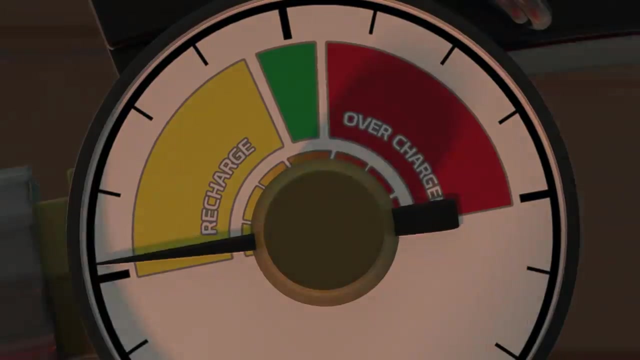 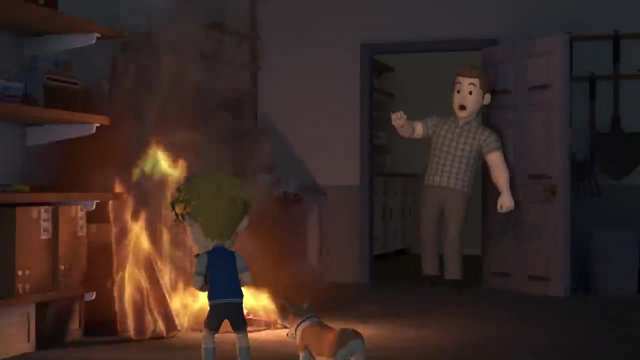 charcoal- yeah, it happens all the time when you're cooking on a grill, mom, that is just the kind of unsafe thinking that leads to really dangerous fires. and that is the final straw I'm taking. this gotta be here somewhere. oh, what is it, buddy? why isn't anything happening, buddy? what is it Peter? hmm, what's up? Jen Roy get to.